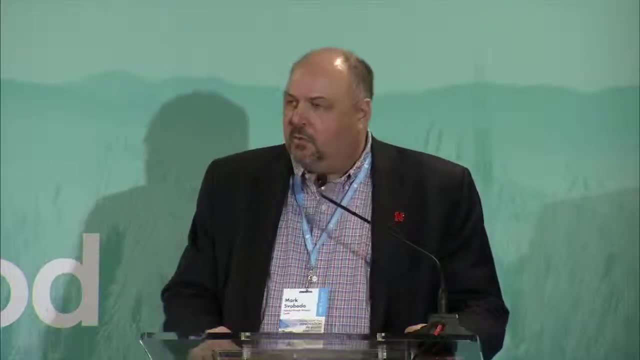 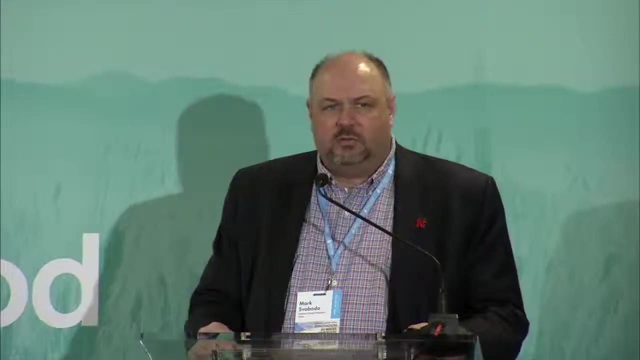 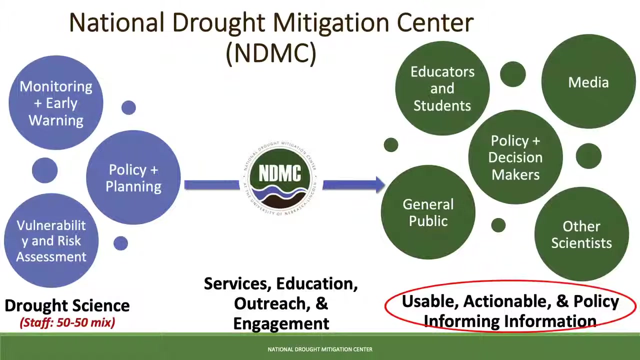 for a comprehensive drought risk management program. So the Drought Mitigation Center- for those of you who are not familiar with us- is what I would categorize as a boundary organization. So one of our main chores is to translate science for the public, for policy makers, for decision makers, to the media. So we're 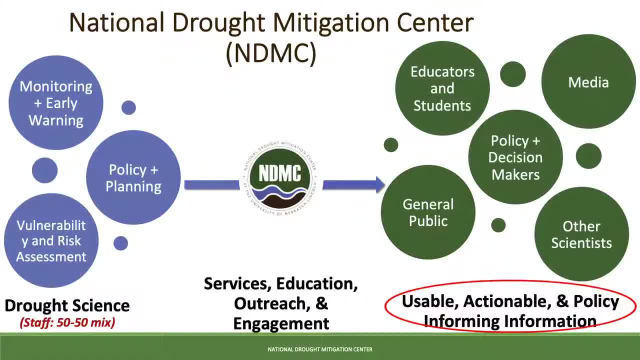 focused on making things understandable and usable. So not just usable but – not just useful, but usable. So our staff, with that goal in mind – and actually Dr Hayes didn't mention this prior – he preceded me as the director. for ten years We've been around – the Drought. 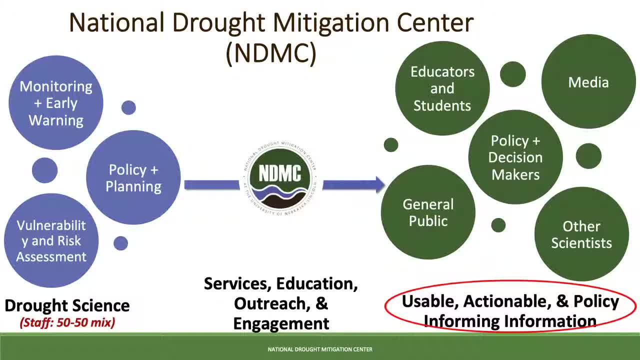 Center's been around since 1995.. Mike and I joined one month apart, back then on day one. Okay, director at that time, Dr Wilhite. but where I'm going with that is that half of our staff are focused on social science. so we really put a lot of emphasis on the now, what type? 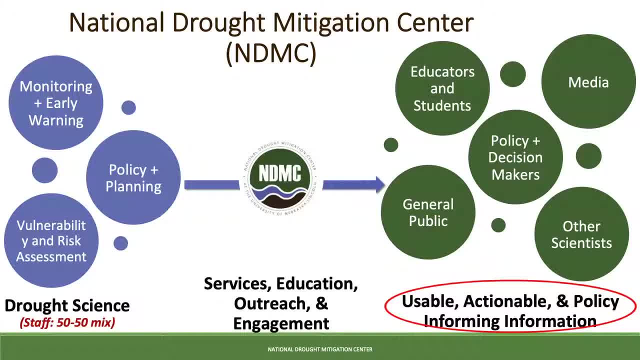 of stuff. so that's what I'm going to focus on here today and we do that through a variety of services oriented sort of approach, very stakeholder oriented, getting out there on the ground with people to develop trust and then carrying that through so they have a 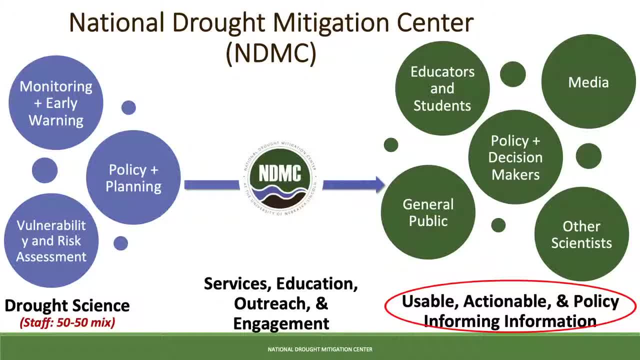 voice in the process, all the way from the very beginning to the end product, and then we carry on those relationships well after the project goes away, which is the very rewarding part to me. So we're very applied in nature is the bottom line. 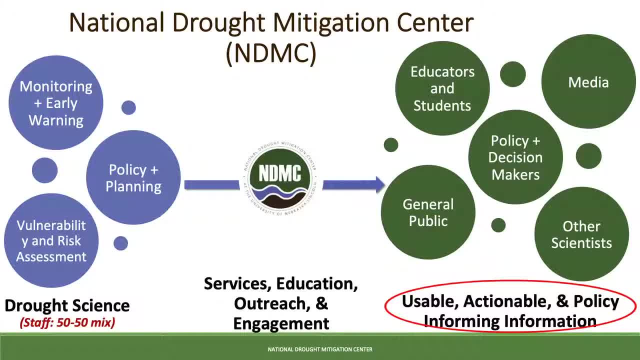 So you can see the green circles. well, to back up the blue circles there, we talked about the three pillars, right? So we have drought early warning, which is the monitoring- personally, we don't do the forecasting per se at the Drought Center- and then we have vulnerability and risk assessment. 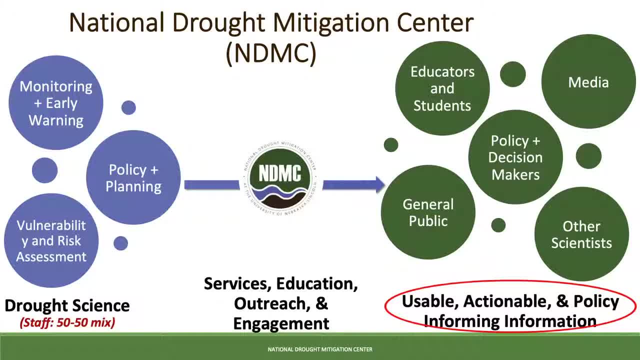 which the social team focuses on closely, And then the policy and planning. of course, is the now. what On the far right, on the green? this is the different areas that we work in. Again, I mentioned those up front, but the bottom line is we want to make things usable. 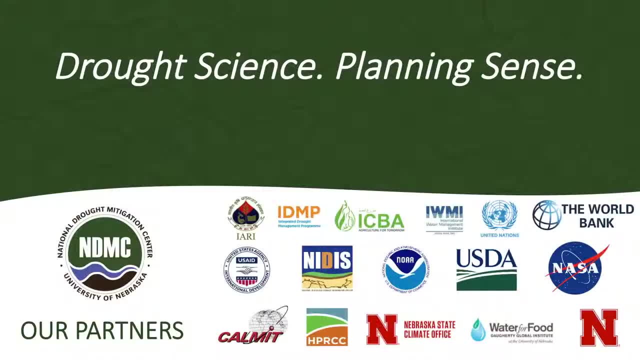 for folks to use. So here I want to acknowledge a lot of our partners, many of whom are in the room on this panel, but also sitting in the audience that we've established over the years, and this is certainly not all of them, but these are some that are again focused on the topic. 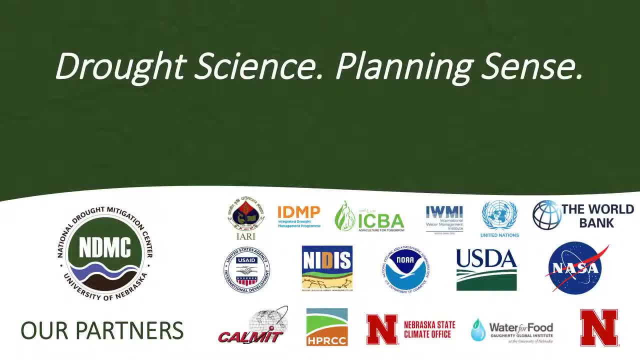 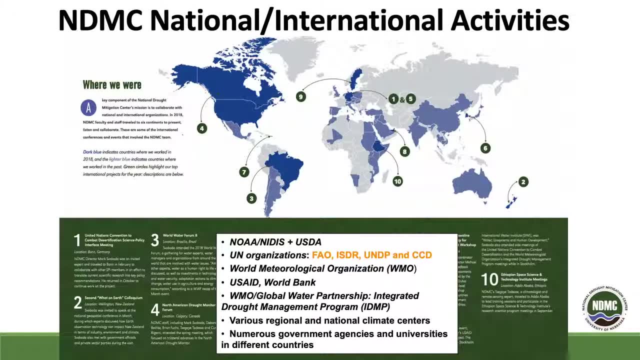 of today, And so I just want to acknowledge all the friends in the room, Because each of these projects, you'll see, this is where we've been our footprint spatially over the last few years. The countries in dark blue are those we've worked with, say, over the last five years. 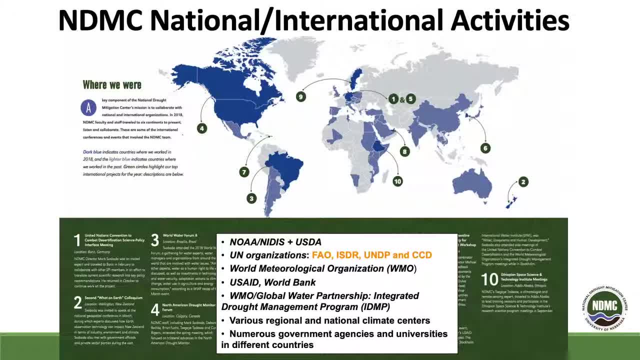 three to five years on a variety of projects. So these aren't just going to a meeting somewhere. these are typically more project oriented And that falls within the group of the United Nations family where we're working with a lot of those different groups. 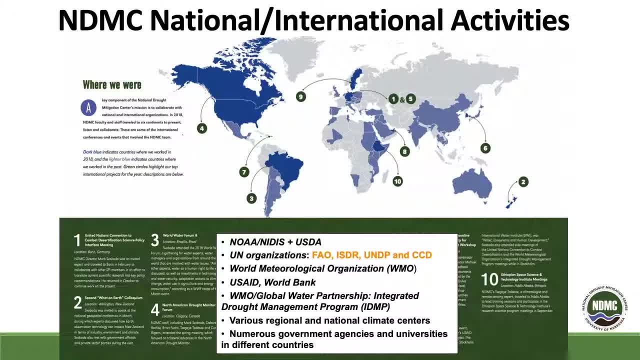 But primarily some are here this week as well. We've heard from like FAO- the Food and Agriculture Organization do a lot of work with the World Meteorological Organization and the Convention to Combat Desertification Group as well. So a smattering of those groups. and then you heard the speaker this morning, Jennifer. 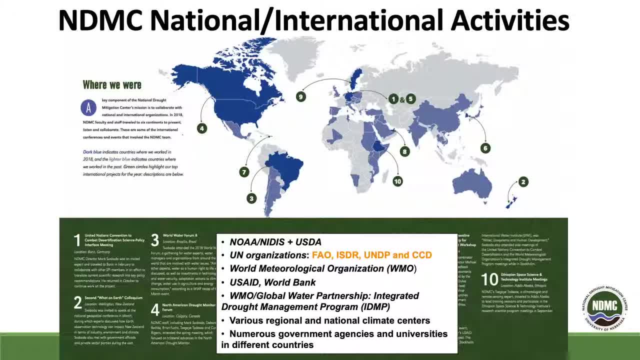 from the World Bank. We're doing projects with them and in fact, hosting a group from. she mentioned the Botswana Project in Eswatini And we'll be hosting a group. We'll be hosting a group of their technical scientists here to start to go down this road. 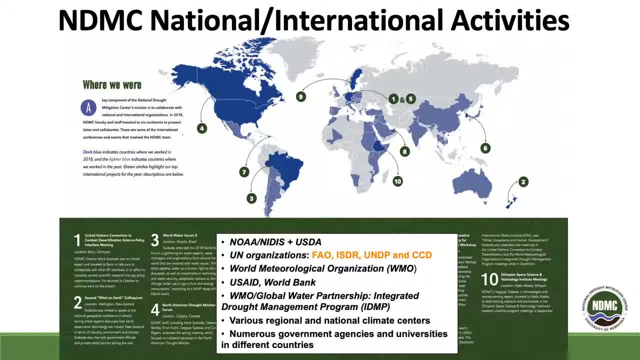 of developing all three pillars, So very excited to start kick off that project here in June. So one of the first Belcal products that we put on the map that really helped put the Drought Center out there in front of people was the US Drought Monitor. 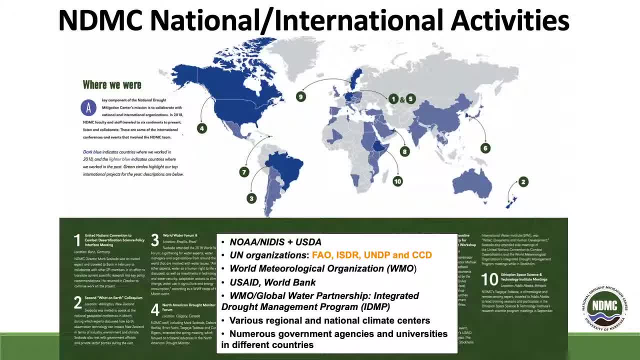 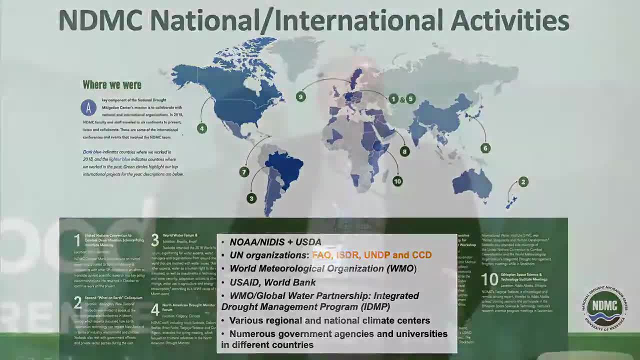 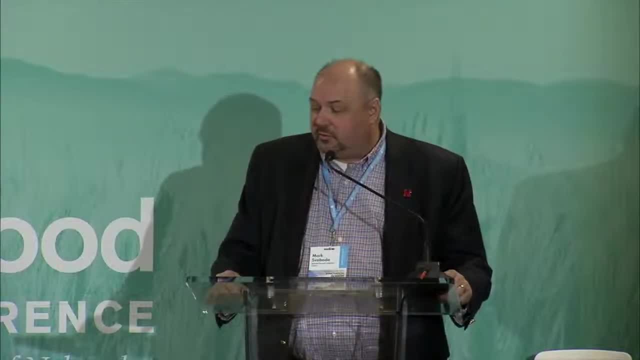 This was developed back in the late 1990s And it's a three-way collaborative project. It's a three-way collaborative project that doesn't have a line-item funding budget. We've done this out of Hyde ever since we started. We've just kind of pieced together what we can here and there, but it's with the United. 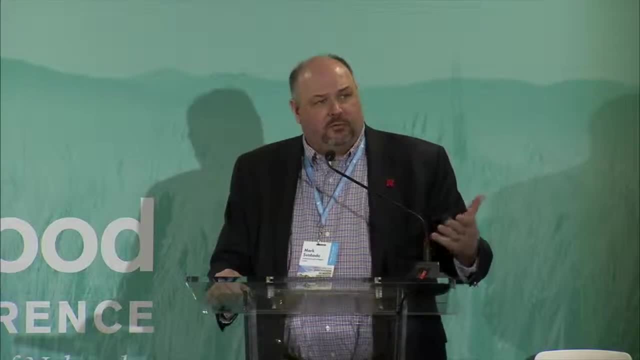 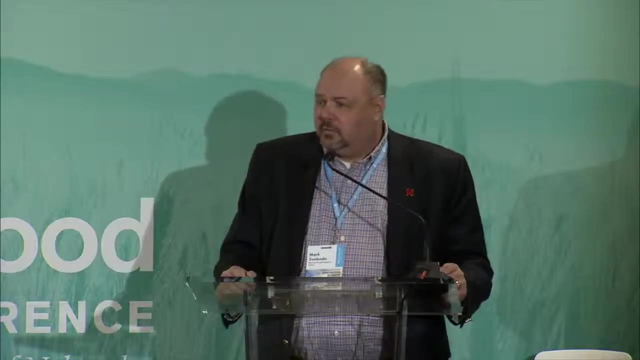 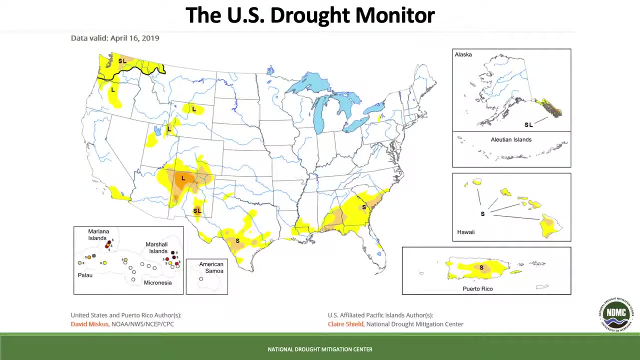 States Department of Agriculture and NOAA, which houses both the weather service that most of you are familiar with, but the Climate Prediction Center and what used to be called the National Climate Data Center, which is now the National Centers for Environmental Information. The reason I put this screenshot up here is just to show you. 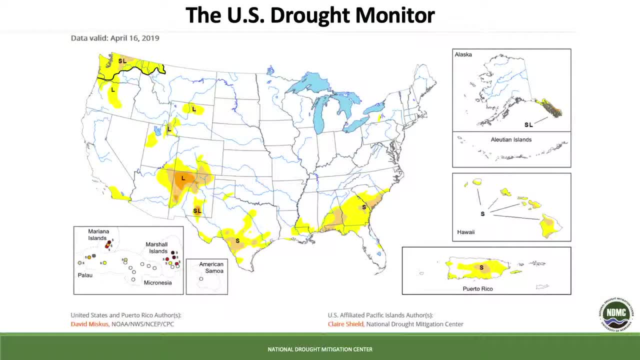 We've recently expanded it. We've expanded it. On the bottom left you'll see an inset map. If you go to the website you'll see the large-scale map If you click on that. we just launched operation of the United States-affiliated Pacific Possessions. 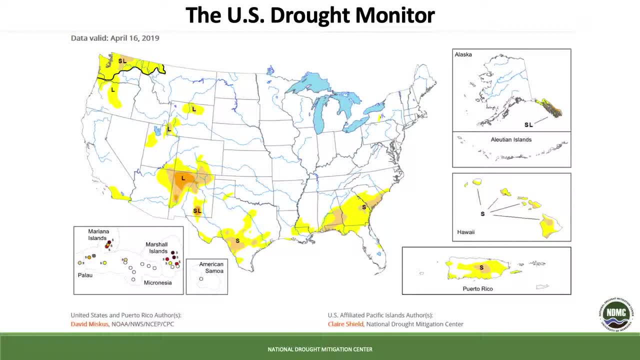 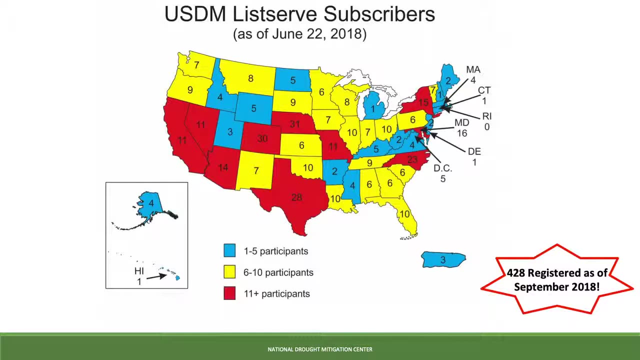 Islands, I should say, And that's just kicked off and will also be doing the US Virgin Islands here this summer to expand the breadth of where the drought monitor is covering, What makes that product unique and I think got us a lot of buy-in and trust was again. 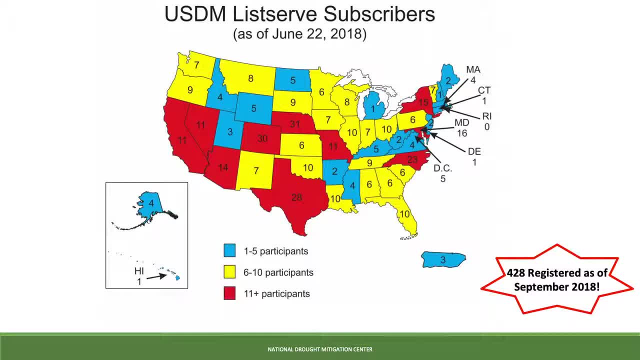 I talked about engaging folks and users from the very beginning at the ground level. So this is a distribution of over 400 people that contribute to the drought monitor each week. Not all 400 every week, depending on where drought is, but during active weeks it can. 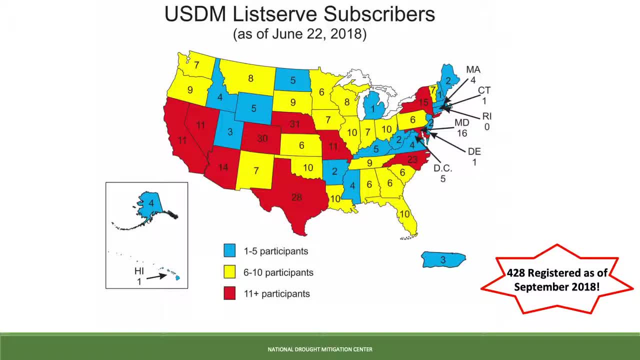 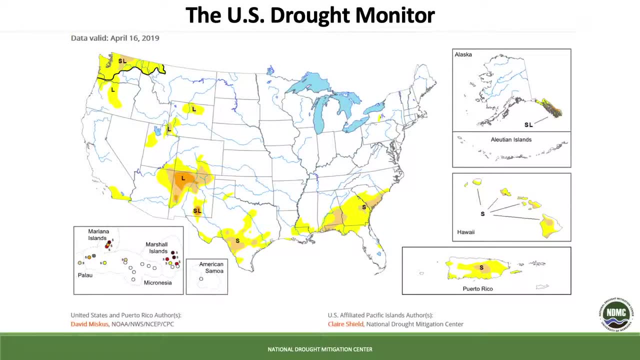 be pretty hectic to get that information into the process. Now, of course, the map I showed you. we only have less than 4% of the United States in drought right now, So this is a record low Since we started making the drought monitor map, but certainly historically pretty darn. 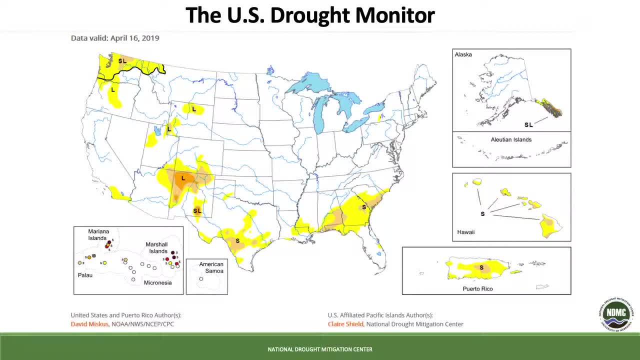 low when you compare it to periods of active drought and even actually compared to even periods of non-drought. That's a very low percentage given the size of the country. We typically average around 10 to 14, 15% of aerial coverage in drought. 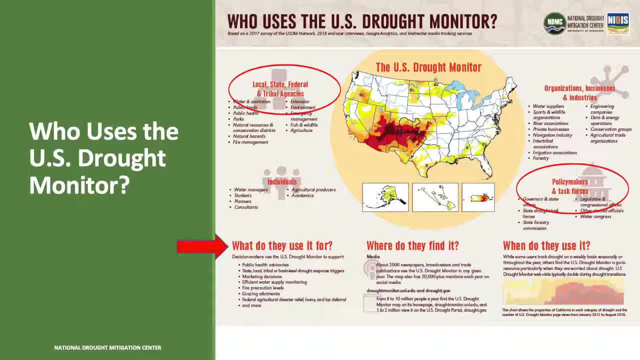 So who uses this? So I talked about users top left. there Again it all scales Local, tribal, state, county, municipality, federal and state agencies and NGOs as well, And it's gotten a lot of play when it started getting shown on the Weather Channel back. 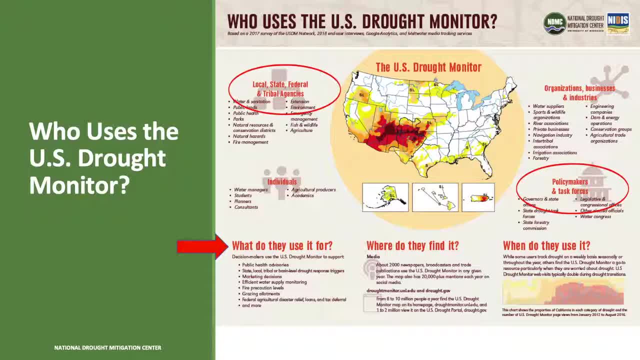 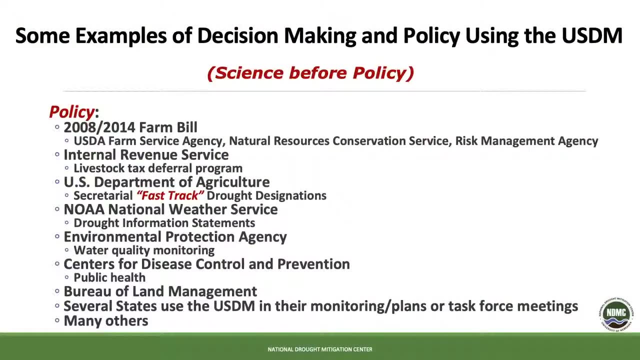 in the day That really put us on the map. But more recently, what's made it work has been we were building this sort of science, as I call it, science before policy. So it wasn't mandated from the top down saying build this drought early warning product for. 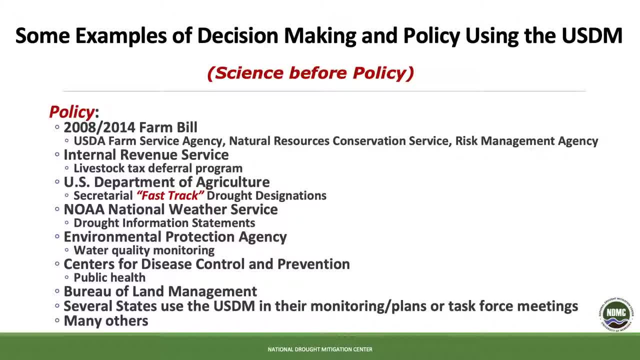 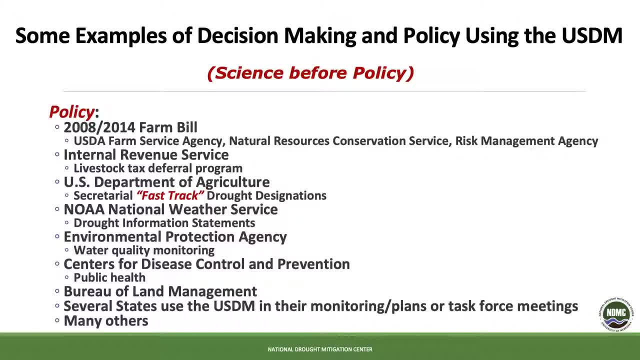 And so the state level. they kind of watched, or lurked, if you will, before it actually got implemented into policy. And now you can see there's a whole bunch of groups now at the state level. Several states use it as a trigger. 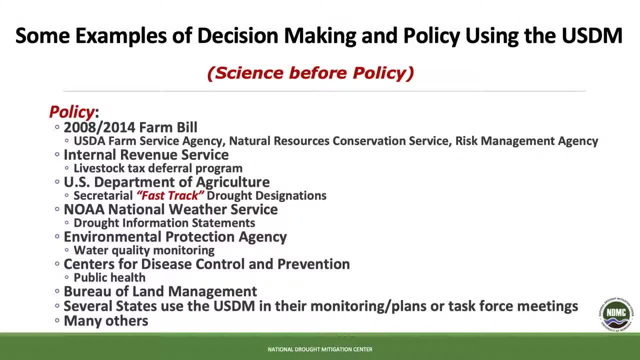 But, most importantly, what put us on the map here was the 2008 Farm Bill, which used it to trigger livestock forage disaster program. To date, that's $7 billion of assistance to livestock farmers that didn't have the the 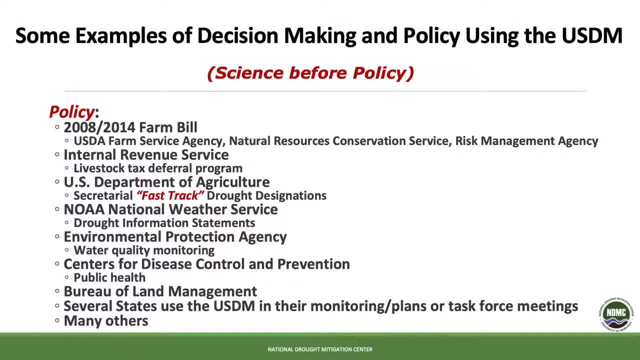 the, the, the crop insurance sort of net at their disposal. So we were providing, I think, a very usable service to the livestock community, Worked with the cattlemen's associations and others around the country, listening to their needs and developed this independently before they used it. 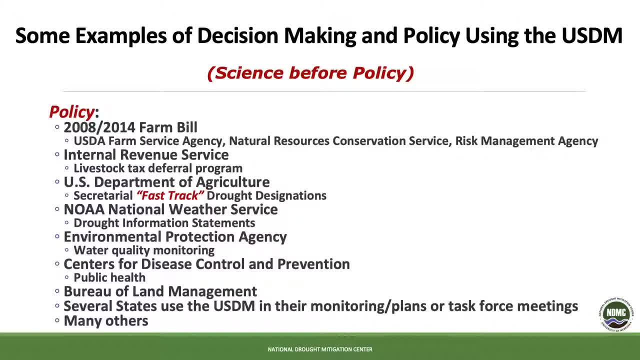 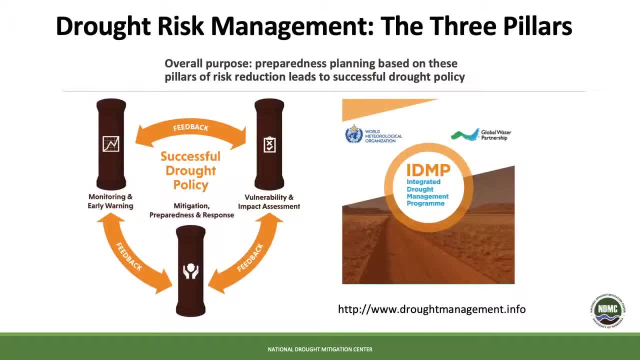 So, again, we have to keep it very unbiased and use let the science drive our decision making, But you can see a lot of others here that I don't have time to go into. So I talked about the three pillars. This is another thing that was born out of Dr Wilhite's initial vision for the Drought. 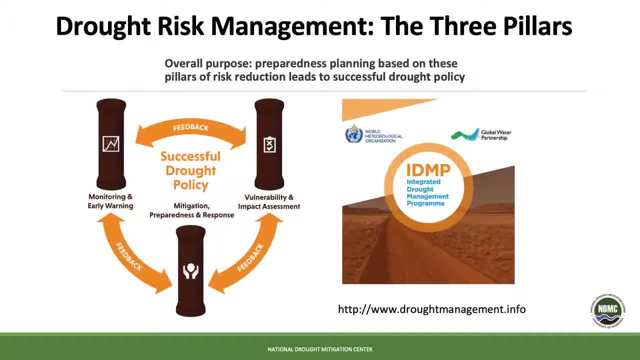 Center was to focus on the three pillars- Drought, Early Warning, Risk Vulnerability Assessment, and Policy and Planning, And so we've been coordinating and working with the Integrated Drought Management Program. That's a partnership between the World Meteorological Organization and the Global Water Partnership. 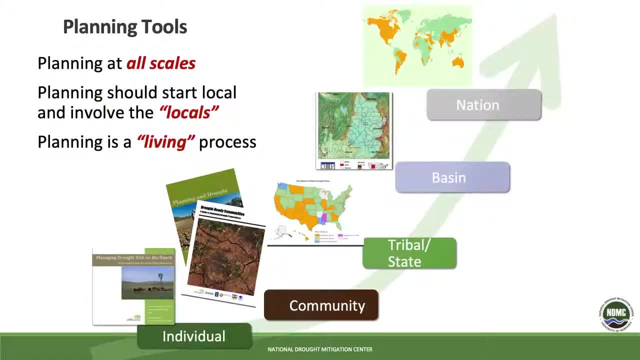 in Stockholm. So a lot of the services that we provide, not just on the early warning. I wanted to show two examples: One, the Drought Monitor, and then on the planning side. you can see here it's a continuum from the very local or even individual scale. 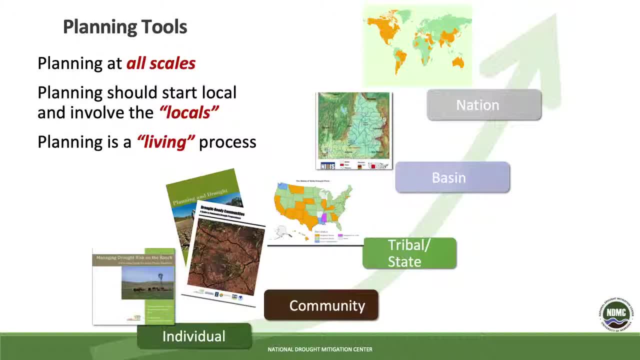 I'd say in the last 10 years or five years, a lot of our requests are coming at the sub-state level. So not even at the state level but at the individual rancher producer level, And certainly at basins and communities. 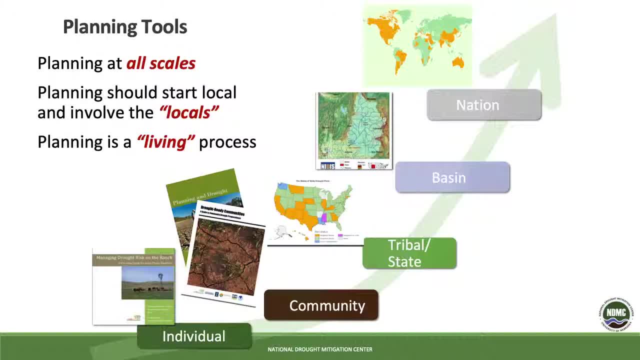 With all the climate change adaptation sort of planning efforts, water planning, et cetera. So we're able to grow and adapt on a daily basis. And then we have some backup plans. We have a lot of additional ground work. We have a lot of land work that we need to include drought in their mission, if you will. 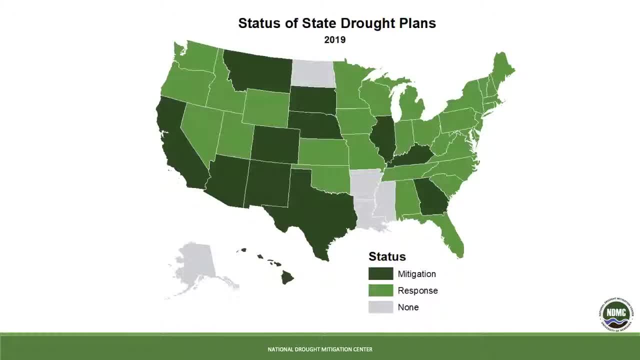 So we're providing a lot of resources. Droughts all start local because that's where the impacts hit the road. So you can see here when, if you go back to 1982, only three states had drought plans. Now on this map we show 45 with droughts. 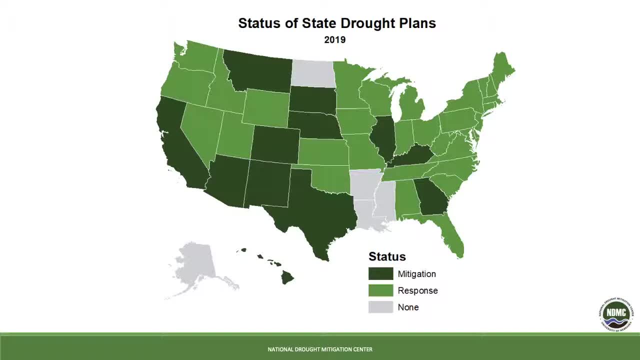 So you think, oh, our work's almost done, what we'd say: all three pillars, not just one or two. so that's our focus is on a lot of work to do to get that whole map. dark green is what we're shooting for. uh, to kind of wrap up here, i just 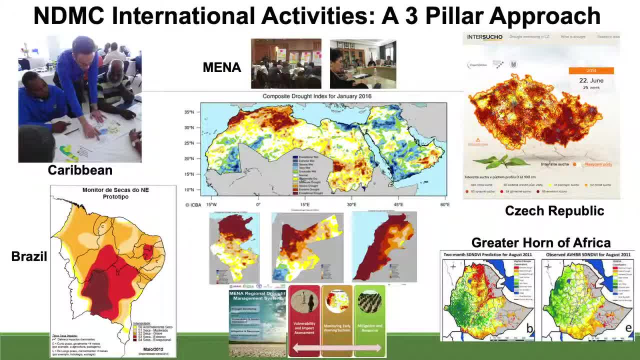 want to show a collage of a lot of different partners that some are in the room here. we've heard a little bit. we'll hear more from eduardo on the brazil- uh, northeastern brazil drop monitor, that we had a part in playing with world bank as well. and most recently you're gonna hear from 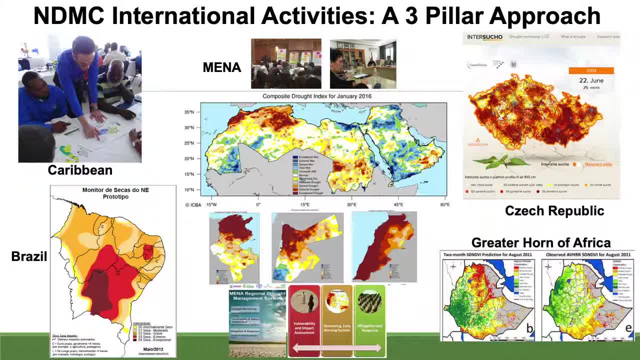 rachel, the bottom, the whole center panel here on the middle east, north africa. it's been a great project: the first three years, phase one. we're phasing into phase two. you'll hear a lot more from her on that. and then you heard a little bit about our work in africa from dr uh sagai. 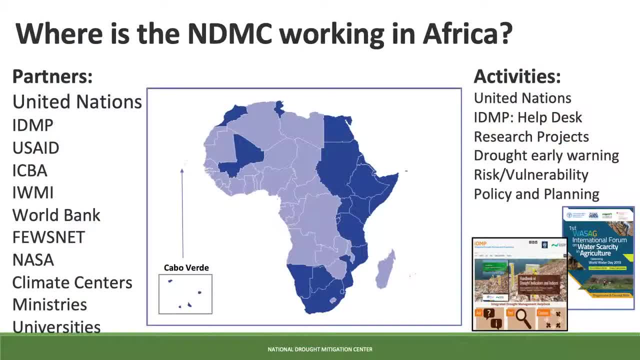 todessa yesterday. here's just a smattering of where we've been at here in africa lately: a lot of different groups on the left. you'll see a lot of the partners that are here, uh, this week. so i can't, if it's over, emphasize that enough. it is really, um, it's a big sandbox. there's a 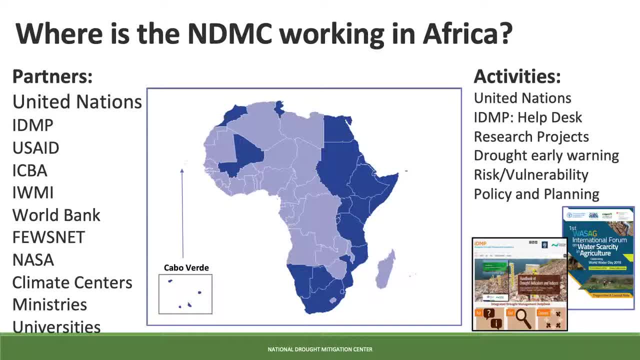 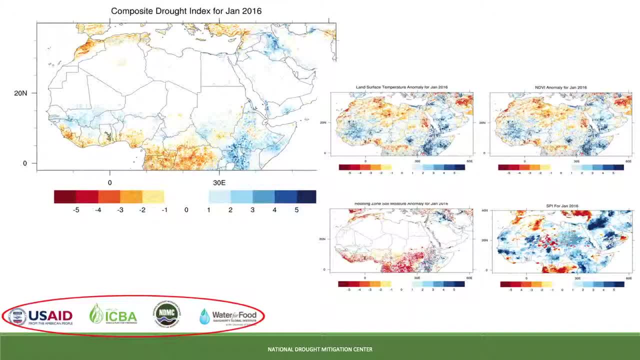 lot of drought is so cross-cutting. uh, there's plenty of work to do and and we welcome partnerships in helping us do just that. this is an example of the drought early warning system we've been developing with rachel's team, prior at iqba and now at the international water management institute. 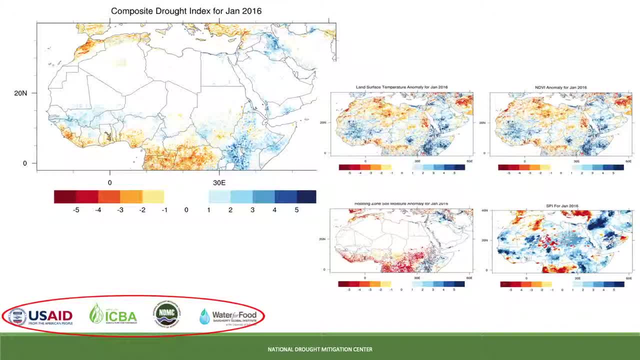 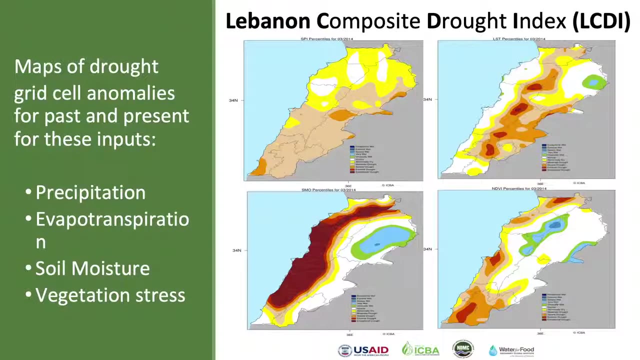 in sri lanka and is to develop- uh, drought, early warning, global hot spot maps and then work with them to take that information into policy and planning, which is what phase two is starting to do. there's our partners there at the bottom. this is just an example. we were in lebanon a couple weeks ago to to wrap up a workshop there. 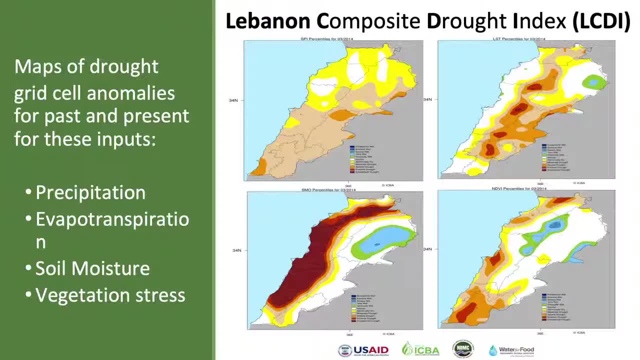 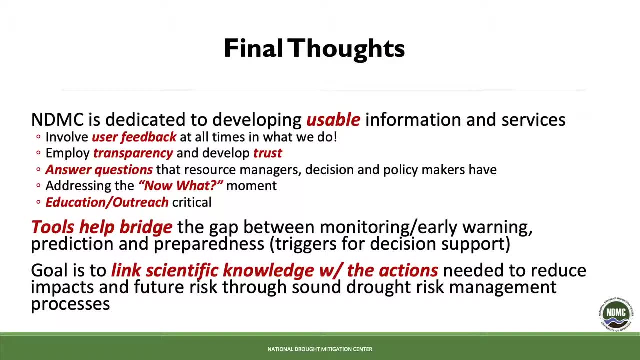 phase one as we go into phase two and developing their drought early warning system, and now we're gonna work into policy and planning. so just to wrap up, i think again we're very applied in nature. we're trying to develop information and tools, decision support. that's usable. 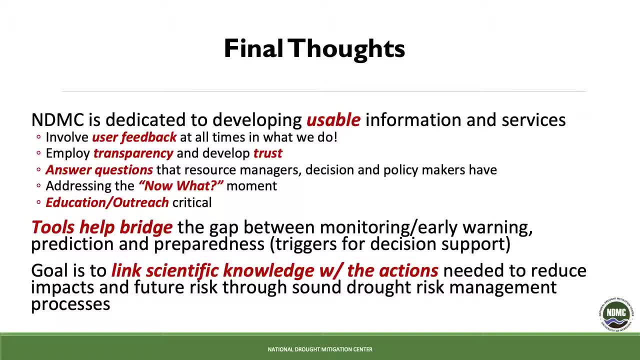 by the locals. they take ownership of it and run with it themselves, which i think is critical. we don't do it for them. so we want to work with them and give them the capacity and training and and work with them after the project's over as well, to sustain that as they go forward. so i've 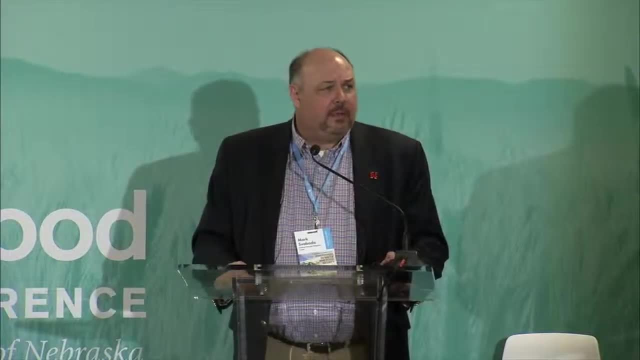 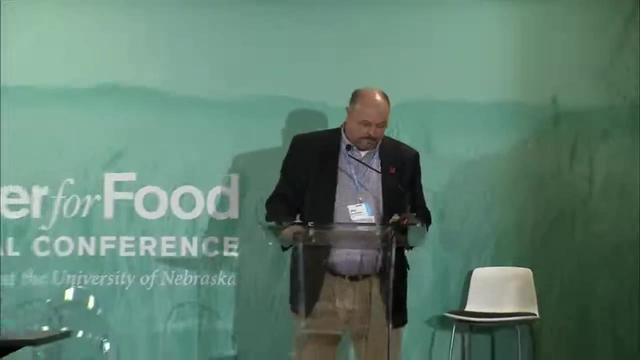 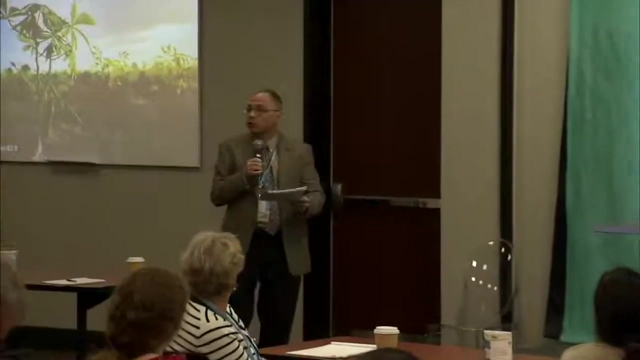 touched on all these. i won't uh reiterate them all, except to say um, thanks again for coming. i think you're going to hear a lot of good examples of the folks i've had the privilege to work with uh on this panel. thank you all right. our next speaker is dr martin. he is the president of fusami in brazil. 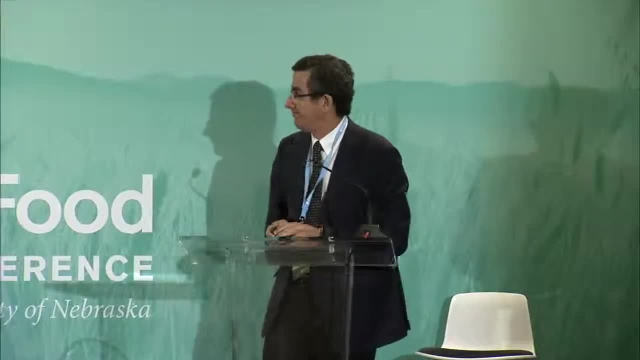 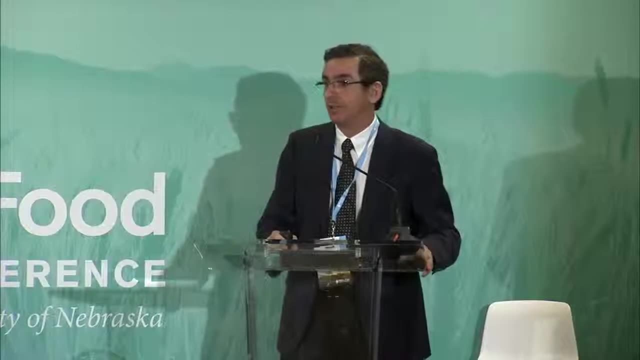 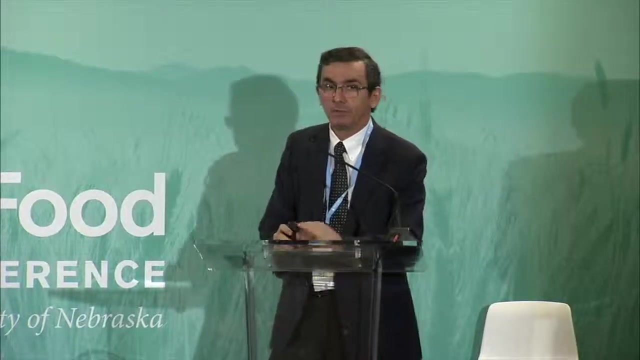 is a zero state, so he will be our next speaker. okay, thank you, mike. thank you, mark, for inviting me here. it's a pleasure to share our experience together with a national drought mitigation center. they really play a key role for us to move the agenda of drought preparedness in brazil and 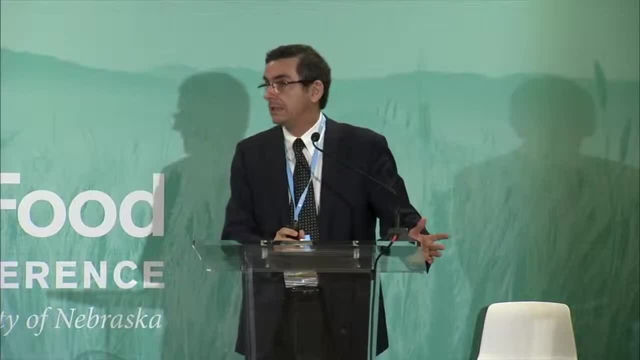 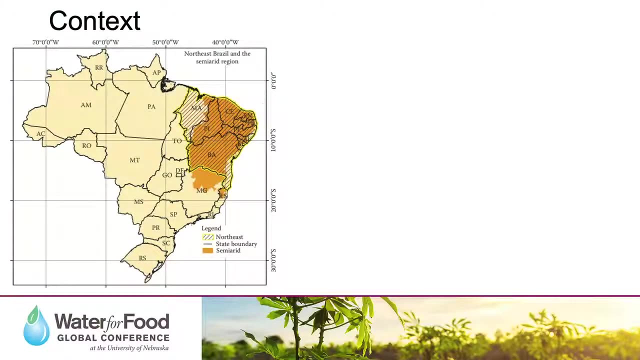 also like to recognize the work that world bank did and supporting all the activities that you carried on in the northeast of brazil. so i will give a little bit of context. maybe folks here don't know where the sierra is, where northeast is. this is, uh, brazil, and this dashed area is the polygon of droughts. 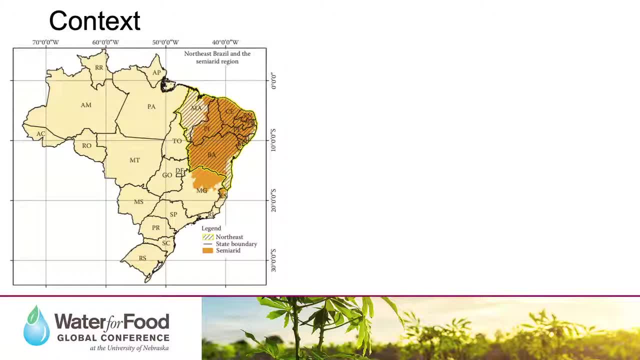 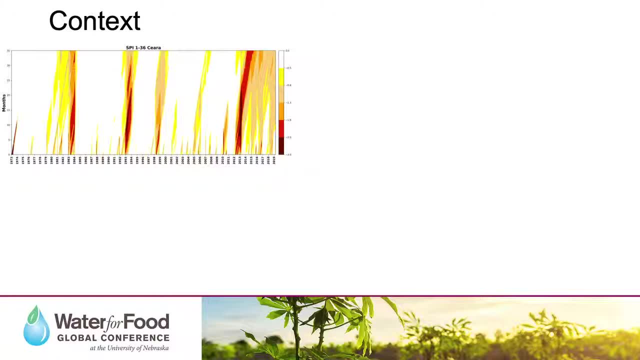 it's the, an area that's really uh cope with a lot of droughts through time and just to give an idea, this is a spi figured from 1 to 36 months- uh the how it is evolving through time. as you can see, the uh drought that we experienced was very long drought and although this is an average, 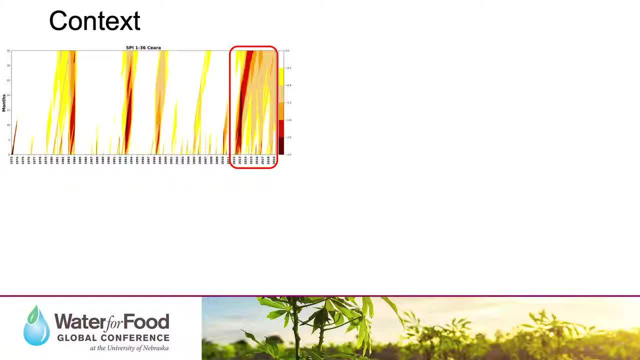 for the state, we see that there are some areas that really cope with very, very severe drought. as you look at the the individual years, we don't see very severe years when compared to the historical record. the problem was the sequence of those years. so when you look for a 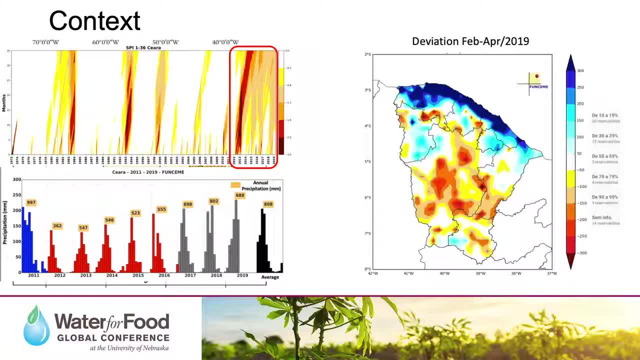 example, this year, 2019, as i would like to point out, we have a very strong gradient north- south, where the areas in hot colors are the the ones that really are coping with droughts still, and these are the areas that we have the biggest dams. so we are still having 30 cities out of 184 there. 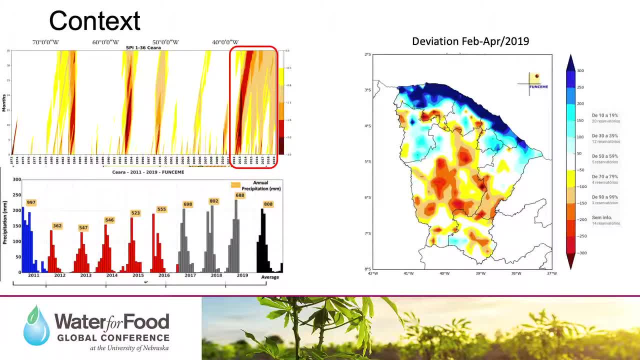 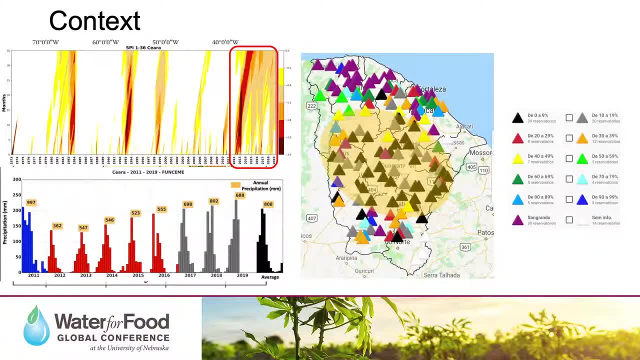 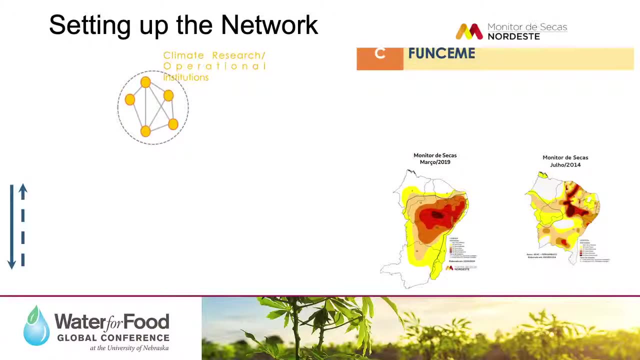 are in risk of water scarcity. so this is why, in this dashed area, we have very low storage levels below 10, and some of these dams are completely empty. so, just to give an idea, we we built the network of the drought monitor on the existing network- uh, the climate network. it was very strong. 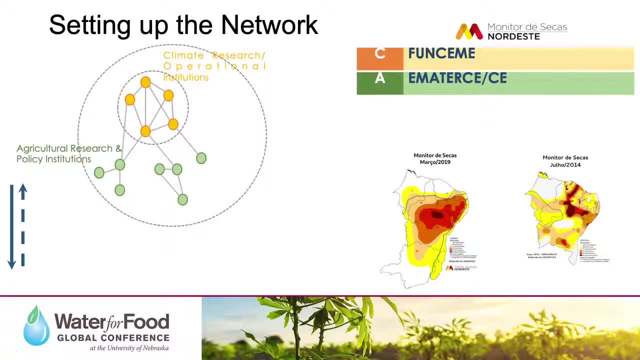 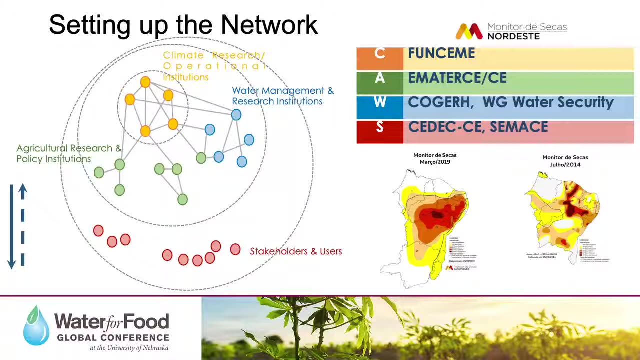 in brazil. so we're starting uh increasing the connections with the what uh the water, the agriculture sector, the uh water sector, and also trying to reach out the the stakeholders itself. so now we are working with the agriculture secretary to have a strong connection with farmers on the field and also not only provide information to them, but 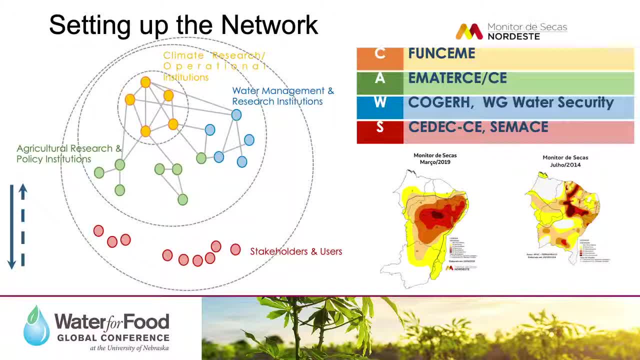 then getting the information to us as well: how. what are the impacts? we are a network of around 47 000 farmers, small farmers and and the triple of that indirectly through the, the agriculture extensionists. so in the in the right, you see the doubt window as evolving through time. 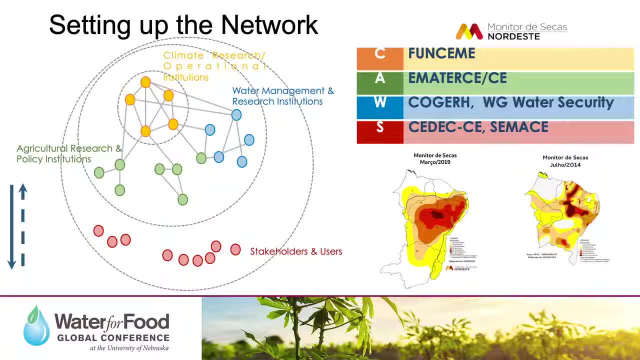 is a very recent uh project, i would say five years. in july we start with nine states in the region with support intensely of the national drought mitigation center and now we are expanded to the parts of the country. so we now have minas gerais and spiritus santo and we're starting talks with 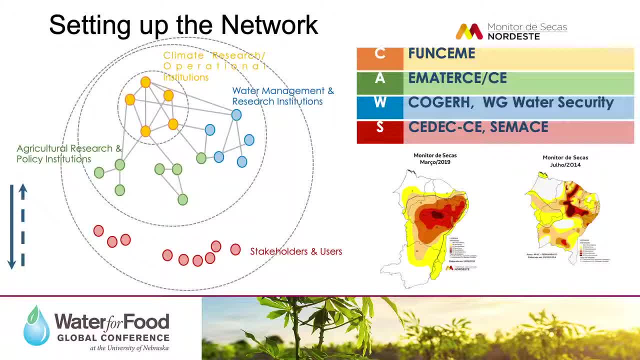 goya's as well. so the the idea is to have the whole country all together and i i'm looking forward to continue the collaboration with the descent and the national drought mitigation center on that. so now we're trying to establish uh field connections with people on the ground. that really 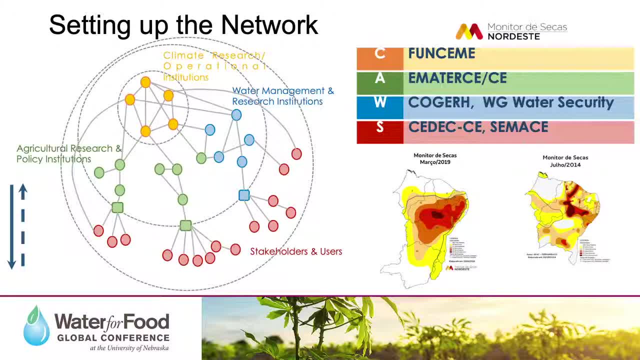 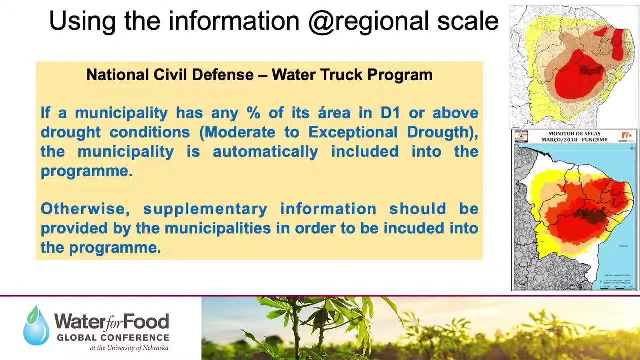 could benefit from this, uh, this project. okay, so we launched, as my uh max told about, the drought monitor here in us. we launched the monitor. don't worry too much from the start on the users- and just trying to convey the mention, the importance to get this information, uh in the in the open and see if people start using. 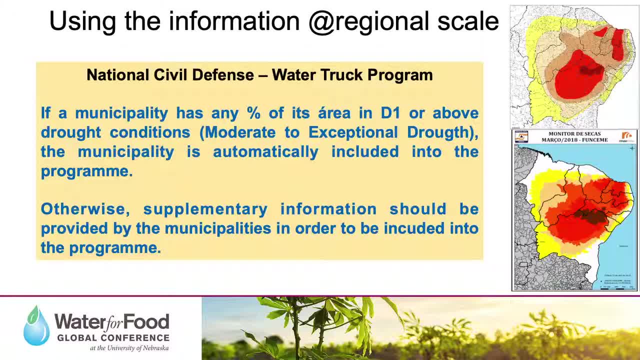 somehow- and we start getting some news on that- we we have the uh national civil defense program water truck tanks to guarantee water for a scattered population in brazil. so they start using the monitor and if the municipality has any percentage of the off area in drought severity level d1 or above, so they don't have to do anything. they they are already. 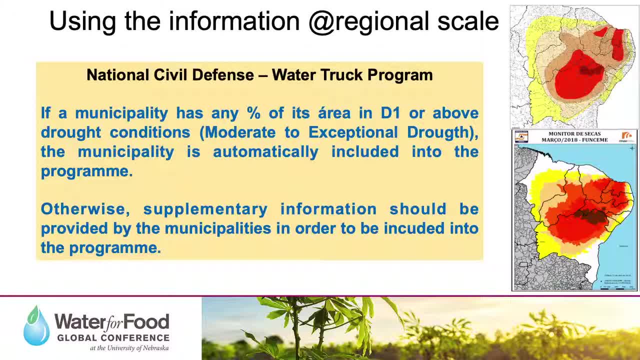 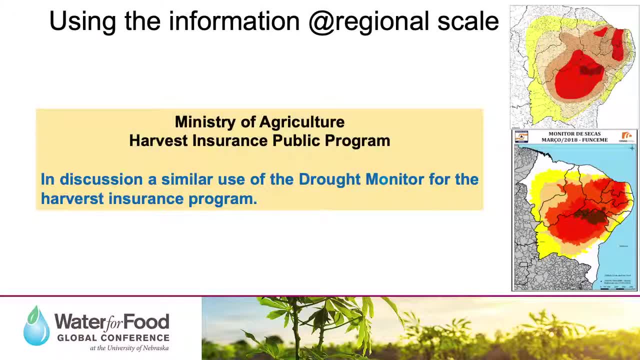 including the program. so this is something that we we really enjoy to to see on the ground people using the information to make decisions and at the same time, we are starting talks with the minister of agriculture for the harvest insurance public program. so if the the, the general idea will be that if the 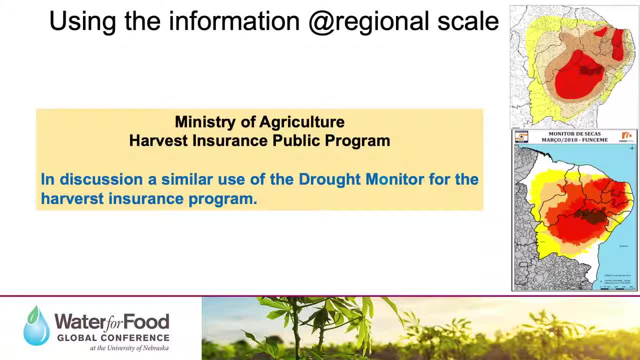 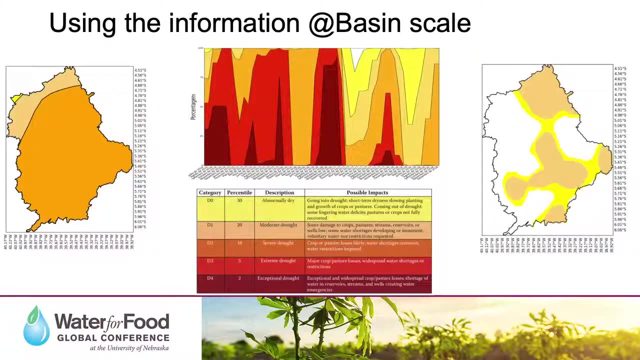 municipality has any percentage in the category d1 or above. we are discussing that they don't need to provide any additional information, so, but it still is in the initial talks, but i think there's some way forward for that. so we're starting, uh, coming up with ways to provide information for these sectors. first idea was to have the 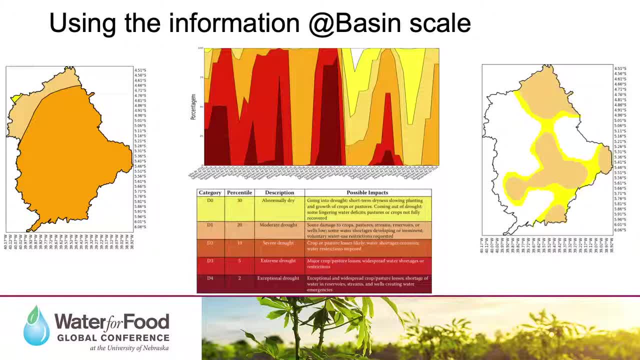 monitor for specific basins in the the state and see how the water sector react to that, and it is very nice because it gave us an alert of the level of drought that this basin is sustaining for two time. so we have some products that are really amazing. um first, come and get them: seven seconds. 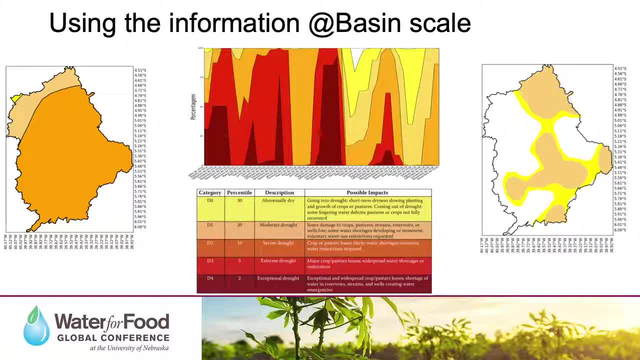 They can access directly through the site. We generated this automatically today to the water agency in Ceará And the idea is to expand to the other states of the country. But it's not that easy And the remote sensing folks could help us a lot. 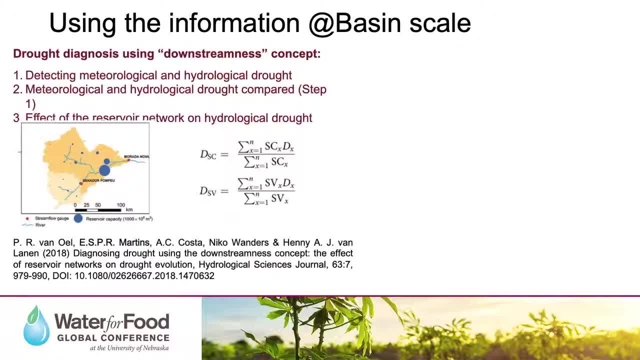 We have a lot of small reservoirs that we don't have any information about. They were private, built by farmers, and so, Just to give an idea, Ceará is one third smaller than Nebraska or so, And we have more than 30,000 small reservoirs with area. 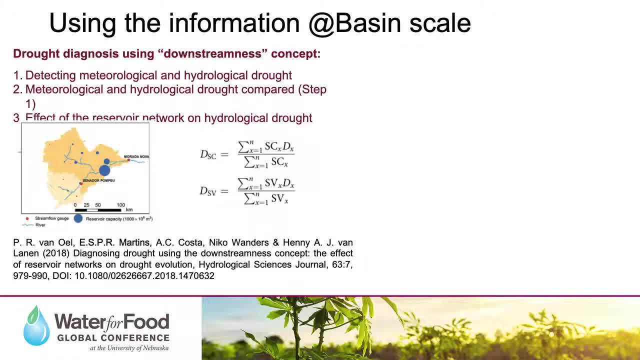 water area surface area greater than half hectare. So this have a huge impact on the inflows for the main reservoirs of the state when we are under drought conditions, And this is something that we need to make people aware of. So, trying to understand how the meteorological 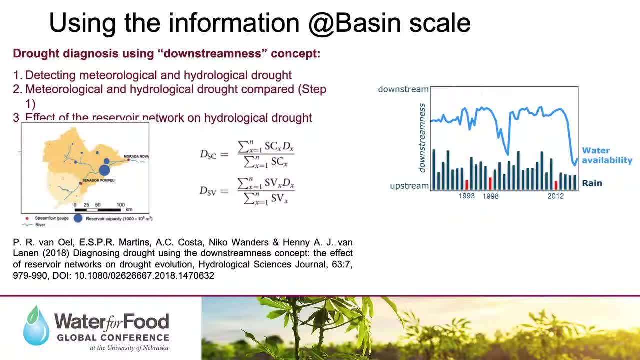 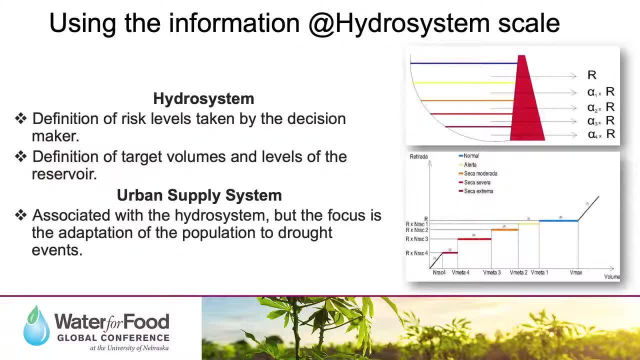 drought propagates onto the hydrological drought has a challenge here that we have trying to address. So also we have to work at the scale of the sector, Of the interest of the sector. So, for example, if you are looking at a hydro system, 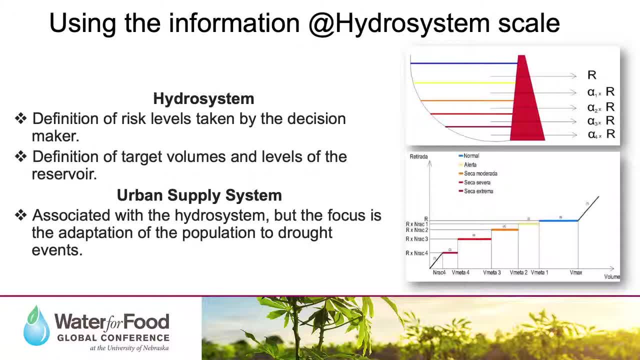 you have to come up with levels that are related to levels of risk, that you are subject to drought or not. Drought, Drought, Drought, Drought. The same thing for the urban supply system. So we did come up, with the help of the World Bank. 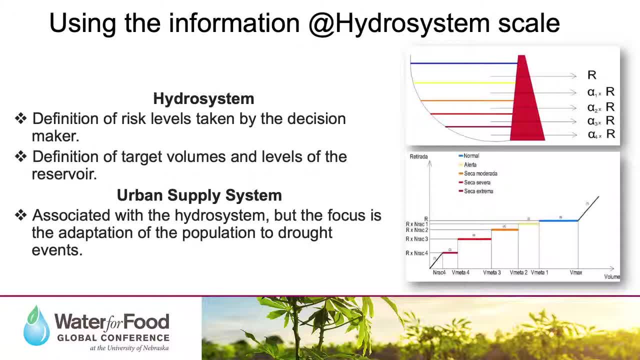 and now, with the support of the National Water Agents- that is running the show now- and come up with some case of studies on those typologies of users, So hydro systems and urban supply systems and rain-fed agriculture systems, and so. So we have some case of studies on that. 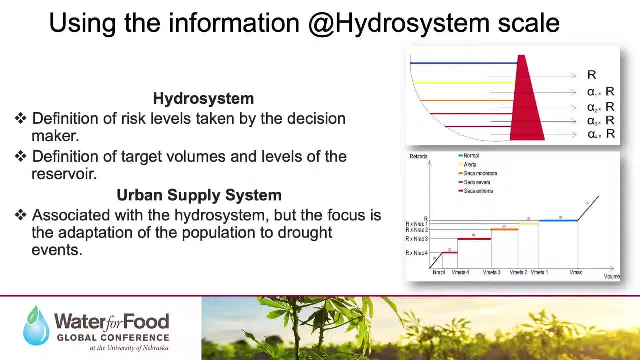 Try to address how would be the nature of the decisions and how they could incorporate the use of the monitor, or if they need to come up with a specific monitoring system that is related to the monitor itself. So for a reservoir, a hydro system scale. 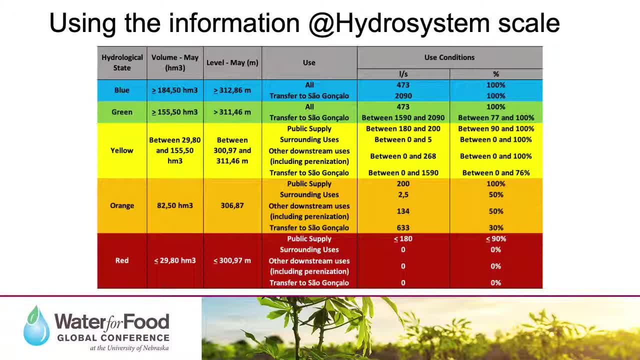 we would have different levels of these reservoirs, associated with different risks and with different uses. That would be that would have water located if the level of the reservoir falls in the range that we are seeing different colors in the screen. So this was one of the ideas. 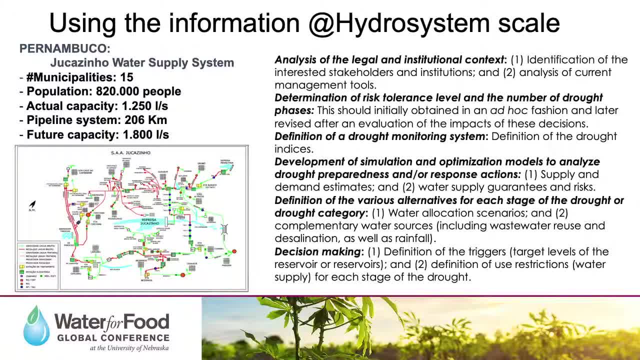 And the other was more complex one. It's a hydro system, So we come up with urban supply system. They're responsible for Recife water supply, So we did have different tools to derive operation rules for the system and associate to the levels of the reservoirs. 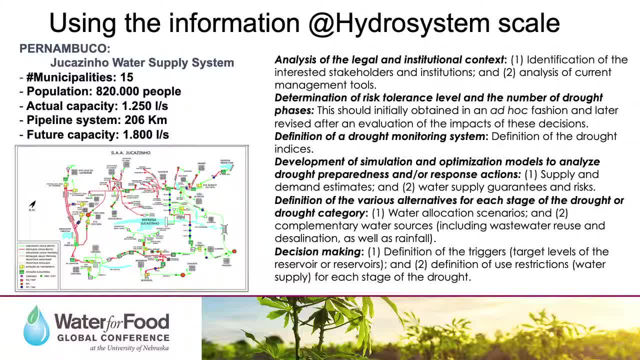 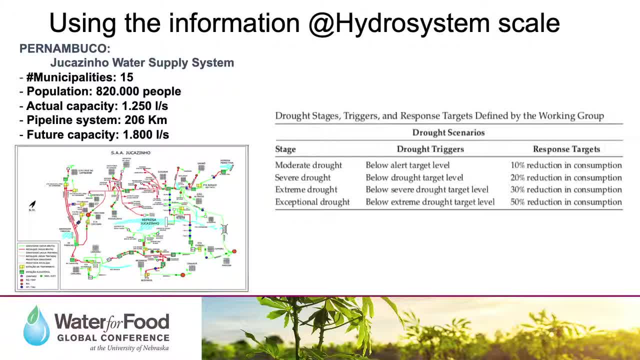 and the risks of being subject to a drought of D1,, D2,, D3, and so on, And this was an idea And by the end we start to derive, depending on the stage, the drought triggers and what would be the response targets. 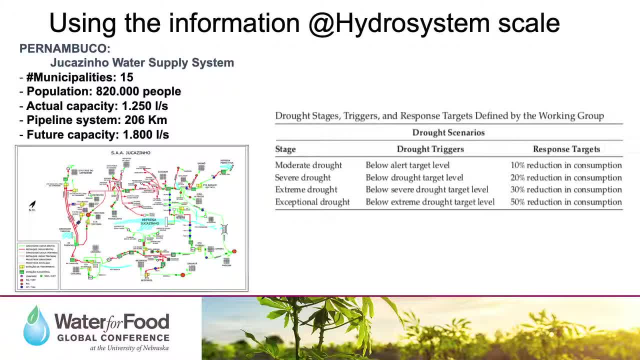 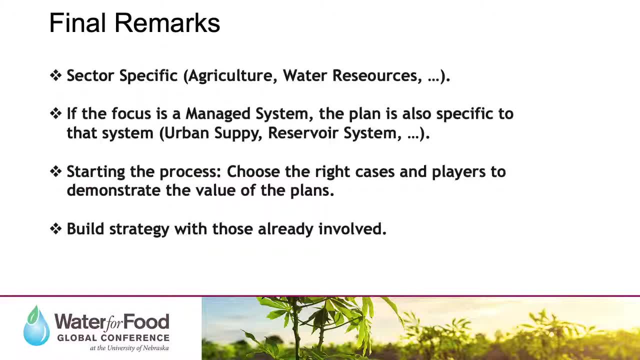 to have in terms of reduction of consumption for the urban area. Well, the challenge: what's next? now what? Well, it's sector specific, the now what. in my view, We have to work with the sector itself and really try. 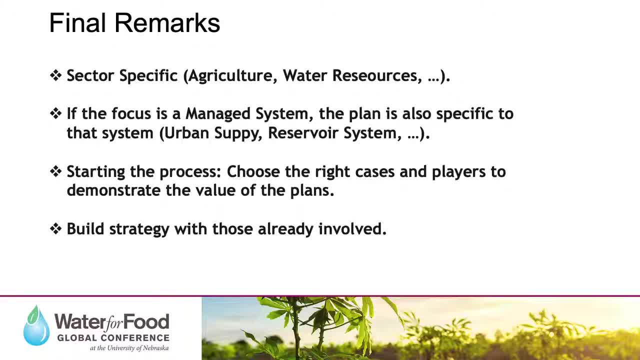 to understand the kind of the decisions that they have to make and try to map that as good as we can. If the focus is a managed system, the plan is also specific to that system. Okay, If the focus is a managed system, this is why it's. 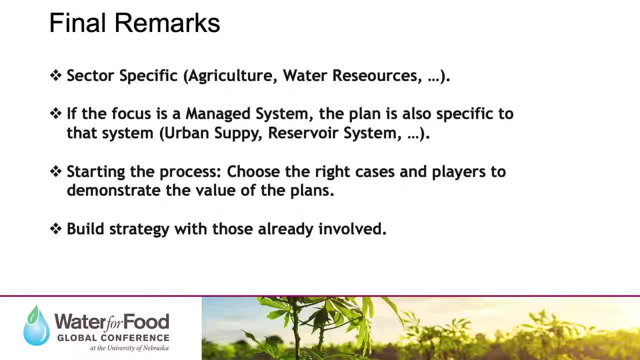 so challenging for us to, because every decision is a new pilot, is a new study for us to come up with really coherent contingency plan for that. So, starting the process, choose the right cases and players to demonstrate the value of the plans. This is what we are trying to accomplish now. 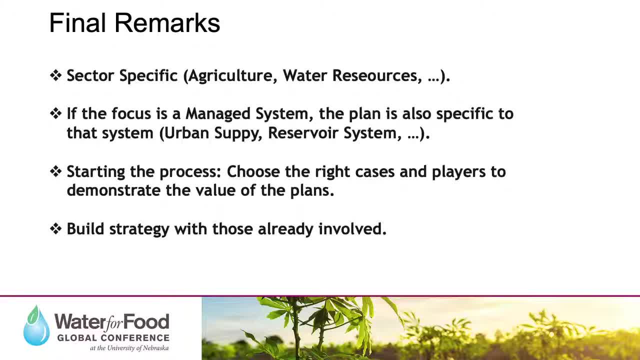 when bringing new states to the monitor, Trying to demonstrate to them how important it is to have this in And build the strategies with those already involved. This is really important. Try to identify the right people to get involved. There's a lot of problems in getting institutions involved. 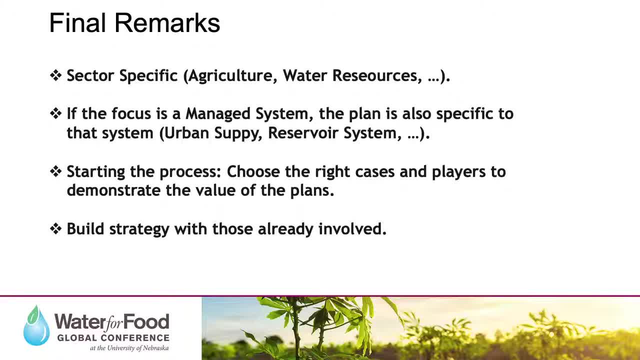 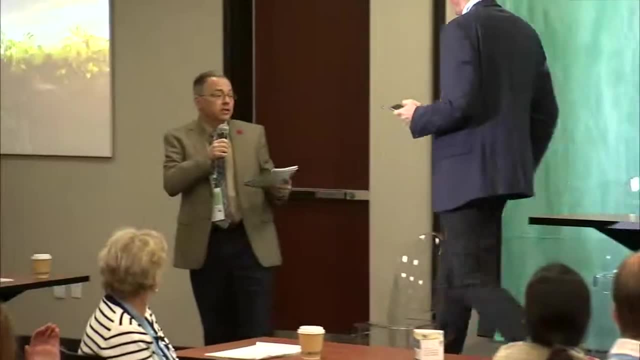 People have to be empowered and feel that the process, they are part of the process and they have some ownership on that too. Well, thank you very much. Our third speaker is Dr David S from the University of Michigan. He's a professor at the University of Michigan. 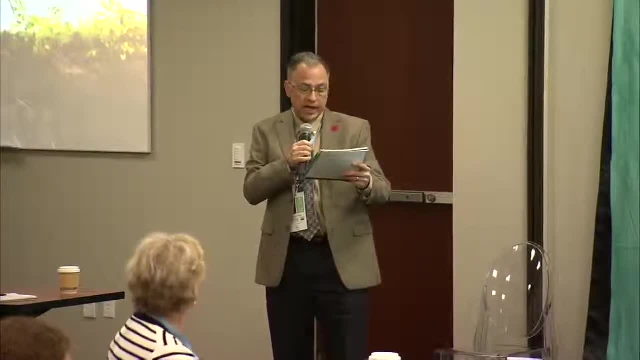 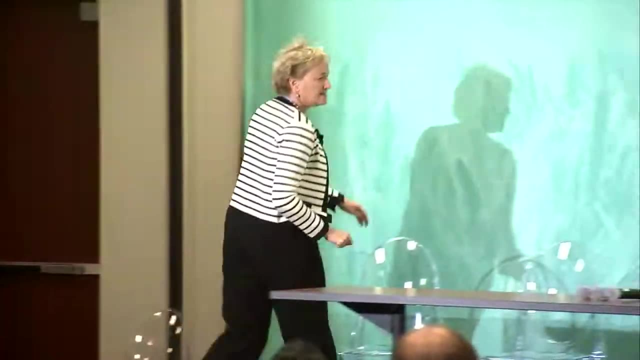 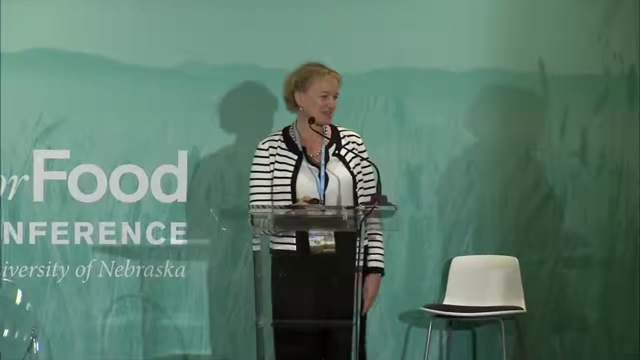 He's going to be here this morning. He is Dr Rachel McDonald, And Rachel is a principle researcher for the International Water Management Institute, IMI, based in Rome. So, Dr McDonald, Thank you Mike, And it's a great pleasure to be here, as ever coming to Nebraska. 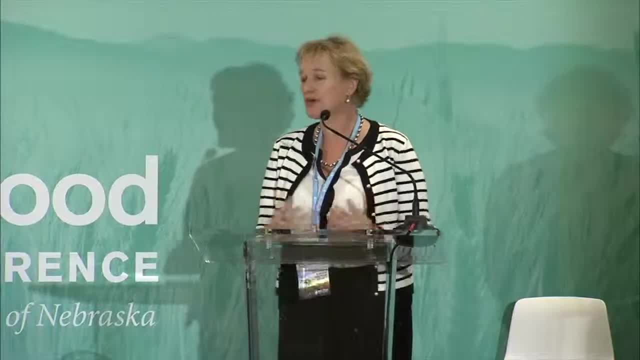 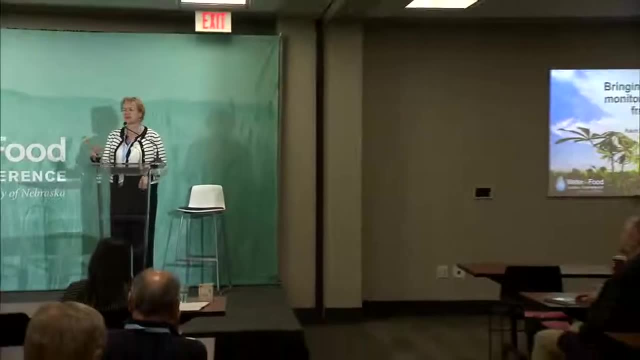 What I wanted to share with you today is the work that we have been doing in the Middle East, North Africa. If you think about it well, North Africa is like this and Jordan, Lebanon, those countries is quite a bit of similarity and it's a relatively arid area already. 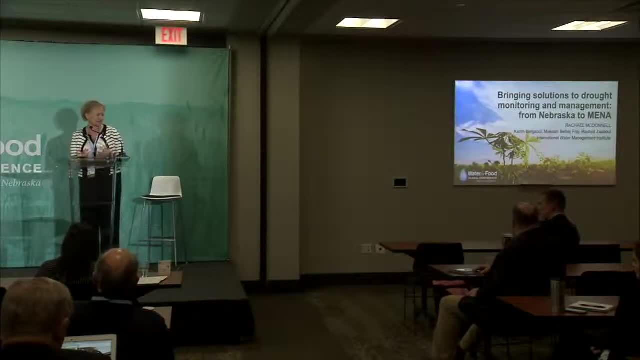 But what we're finding in our project is: it is very different. Drought in each of these countries is very different. So what I want to do is I'm starting with the so what's next? and this is really looking at the second phase. 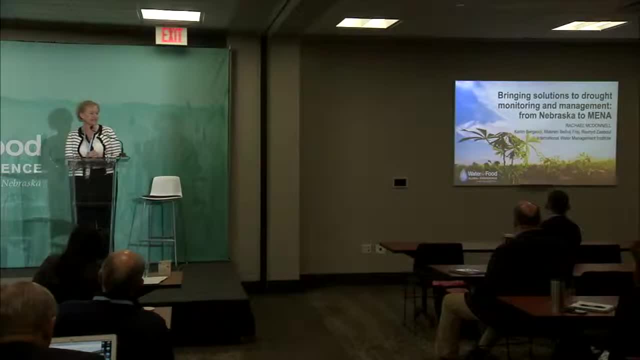 of a USA project that we've been doing, And all of this. we started working with Nebraska probably five years ago and we could see that droughts are going to be an increasingly challenging issue in the Middle East- North Africa. You've only got to look at the situation in Syria. 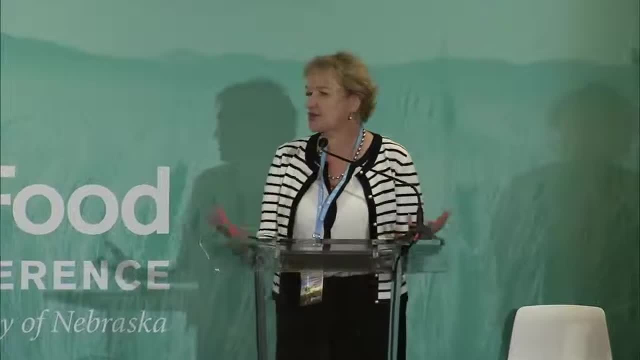 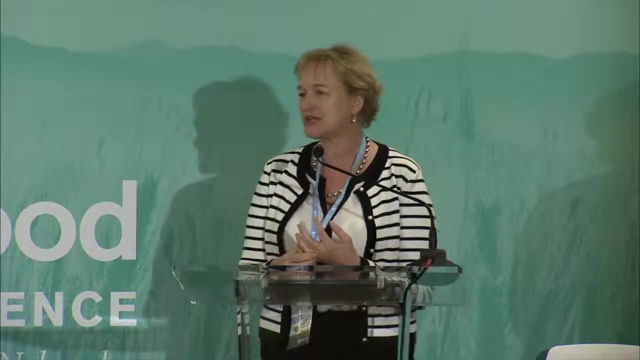 and many of these areas here, But where do you start? You can download your idea, you know your 10 steps from the World Meteorological Organization, GWP, but that doesn't really tell you how to start. So we were delighted to hijack Nebraska to join us. 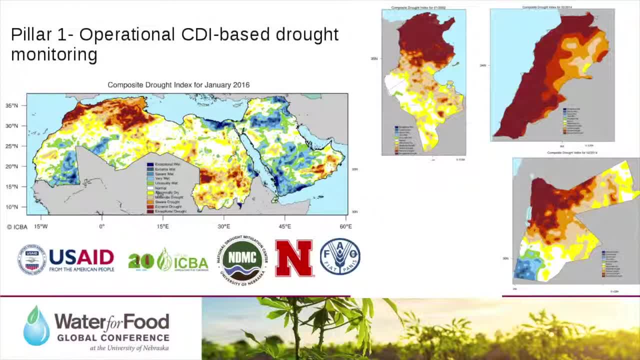 on our journey, and so it's very much from Nebraska to the MENA. So Mark's talked about the three pillars. so our first step of it all was setting up drought monitoring, and we've just been hearing from Dr Eduardo about this. 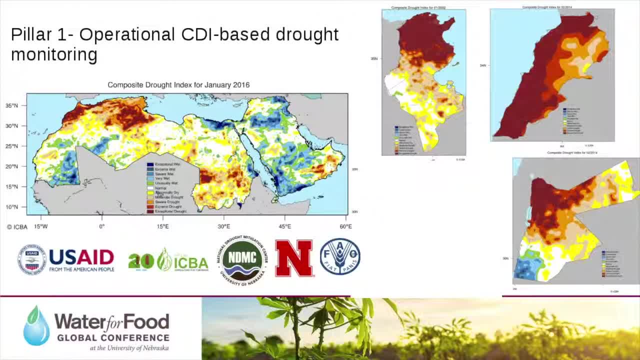 So if you're going to set up operational drought monitoring, this means it's got to be able to work when the internet is a little bit difficult, when the budgets are being cut, and it's also got to be about accessing data that's free. 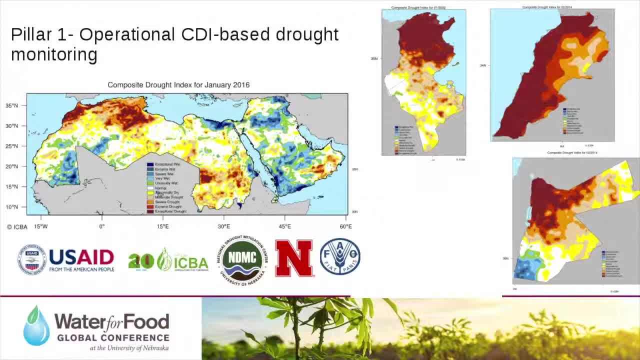 So, in designing that, we could make a very complicated drought monitor, but we have made a relatively simple one, building on the experiences of the MENA, And so we have developed a drought monitor for each of those four countries: Jordan, Lebanon. 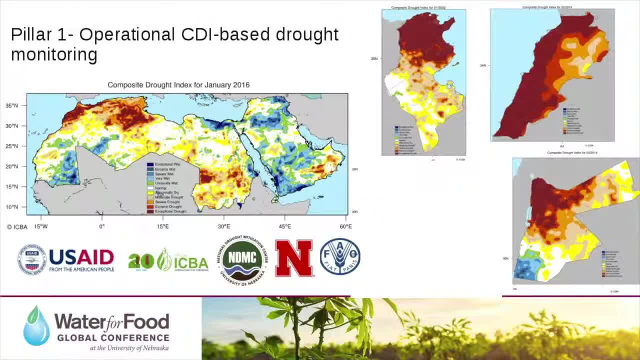 Tunisia and Morocco. This was undertaken at the International Center of Biosaline Agriculture, my former organization working with Nebraska, and at the regional level, And here we've brought together drought maps. but what we then did was, you know, the bringing together the data technology. 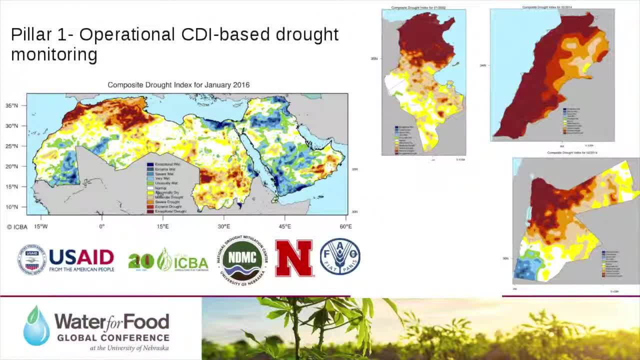 and pressing the button is an easy bit. We now have to validate it. So what we've been doing is we've been working with in-country partners and we're going to say we can generate the maps for 2014, but does it actually reflect how you were experiencing drought? 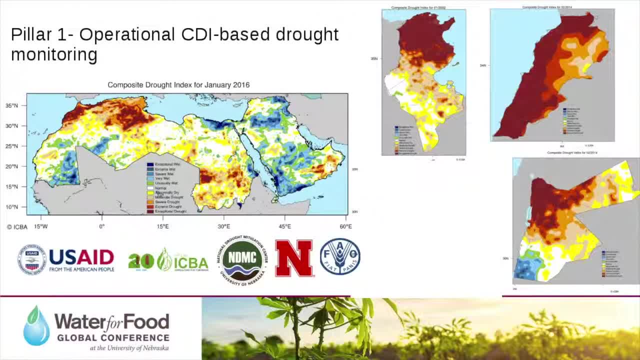 in that year, because drought is a very local, it's a very subjective, it's a very unique experience. So we've had to look, for example, in Morocco there's a lot of snow, and in Lebanon, So if the drought is during that winter period, 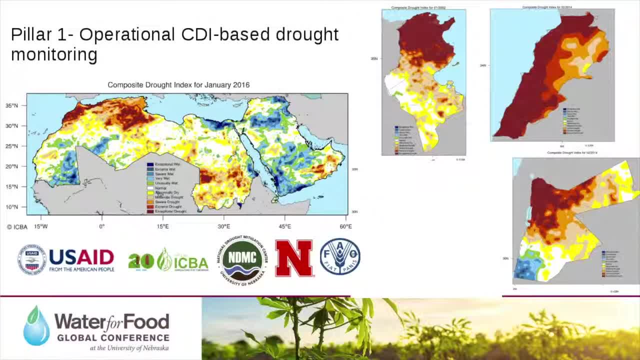 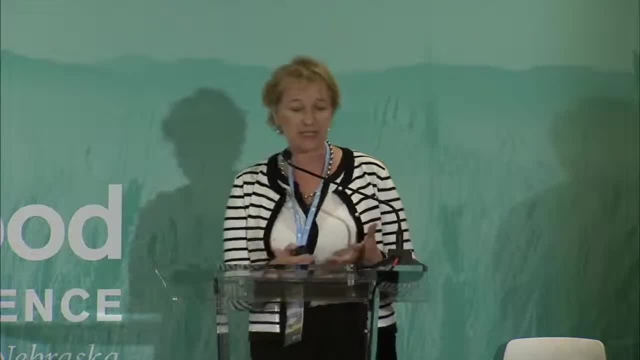 and the snow doesn't fall. it means that spring and summer stream flows. So we've been working with the federal government to make sure that the maps are really messed up. So we have- and not only have we had- the validation take place. 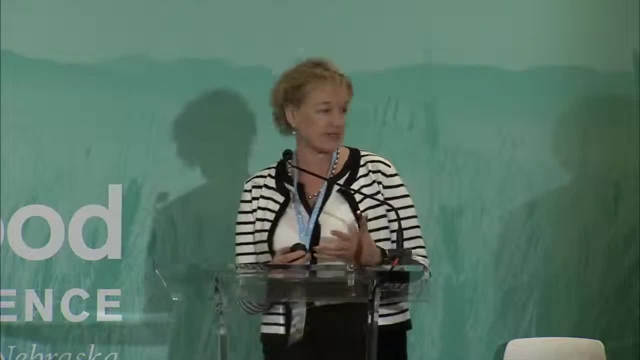 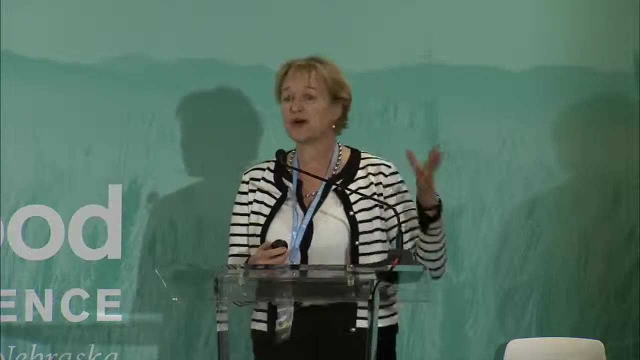 in the country. we're also building from Nebraska's experience US Drought Monitor and setting up evaluators. So as we generate that data, we need people in different parts of the countries to check. is it okay? Is this drought map okay? 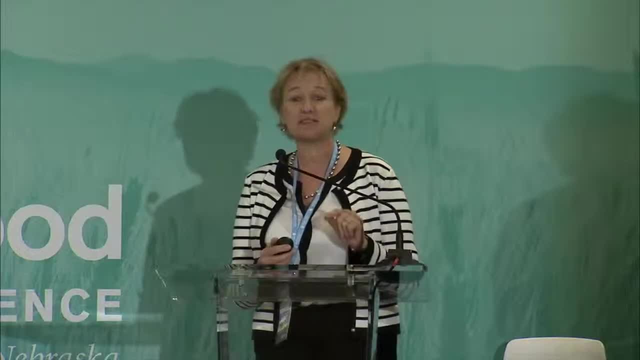 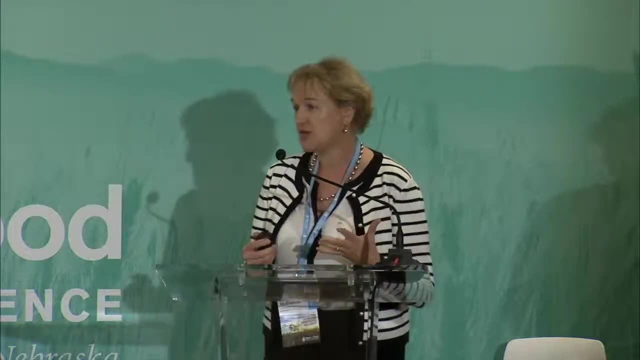 Because what we have to do is we then have to be able to make decisions based on that drought map. This might be involving funding, It might be involving turning water off, So we have to be able to trust that drought map. So this is the stage we're at. 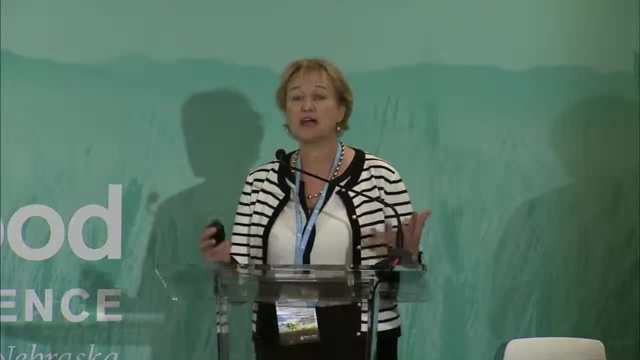 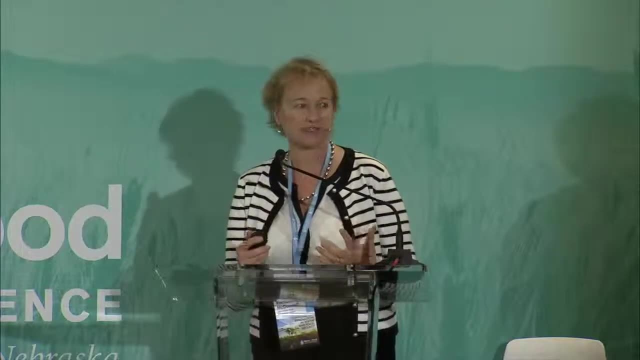 The other thing that we learned from Nebraska is that it has to be multiple ministries, interdisciplinary, everybody coming together. So that means sharing the funding, sharing access to the technology, sharing access to when Nebraska comes to town, which is always a big pull. 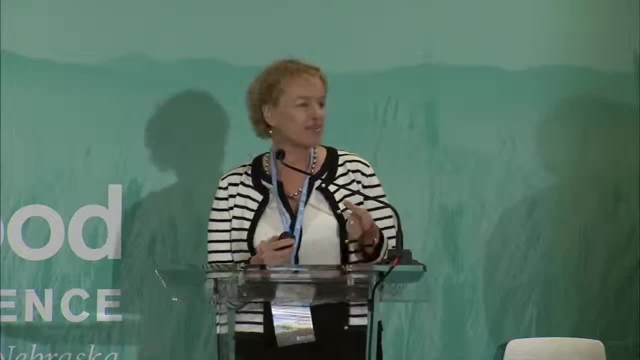 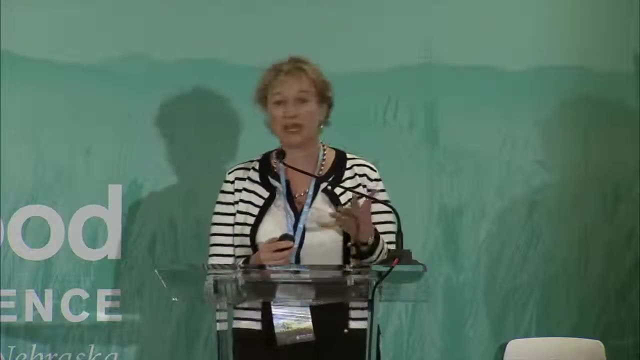 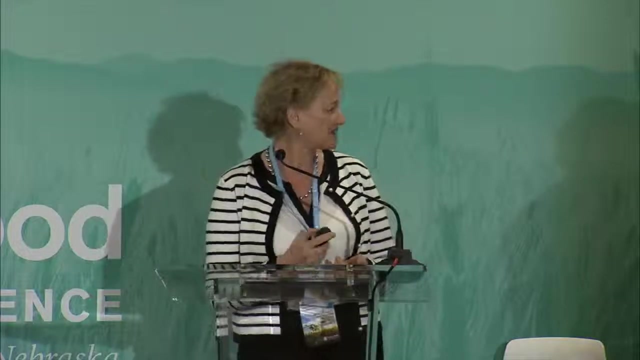 So this is how we've done So in each of the countries. the generating group tend to be young engineers from meteorology, agriculture, water, economics and environment, and they generate the map, which means that their stakeholders are happy with it. 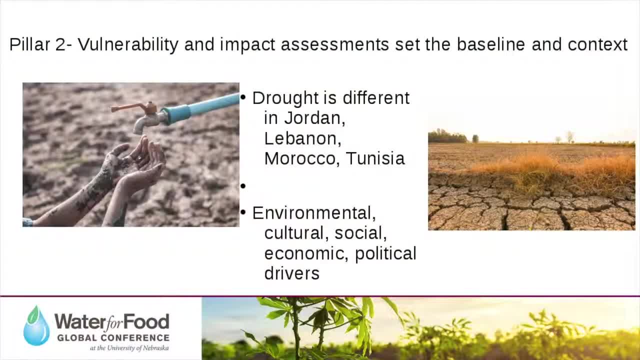 The second pillar is looking at vulnerability and impact assessment. We need to know who is impacted and why are they impacted, because just because you have a drought does not mean to say that you are going to be as negatively impacted as that. So we need to look at which sectors and because of our 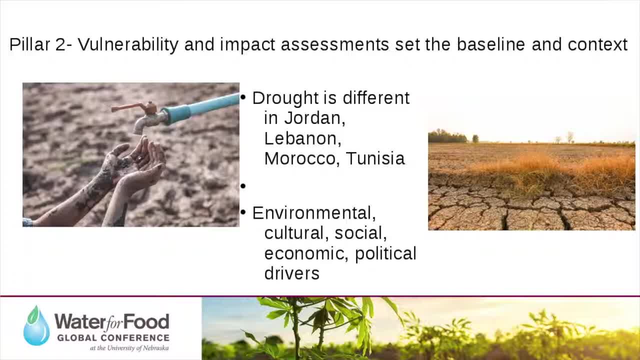 anyway, we need to look at the impact sectors In each of these countries. rain-fed agriculture is very important. We know that agriculture, and so food security, is a major impact. But what we also know that a drought in Jordan and a drought in Lebanon can be equally severe. 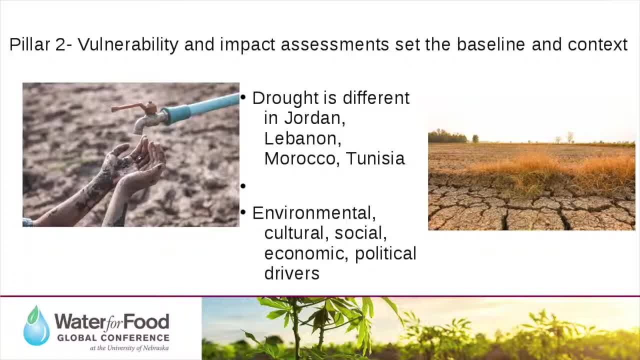 But the impact in Lebanon is much less because there's 50% irrigation. But the problem is it looks as though it's less severe because the crops keep growing and the vegetables make it to the market and they export to Europe, So it doesn't look that bad. 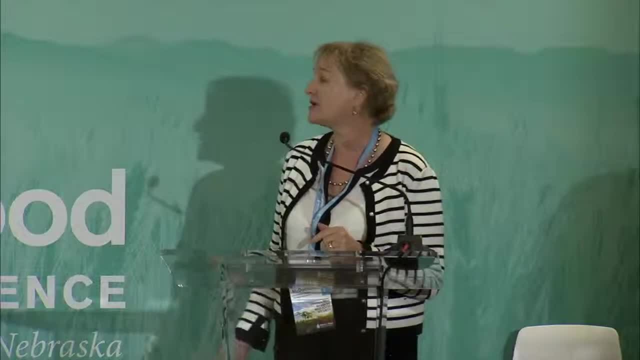 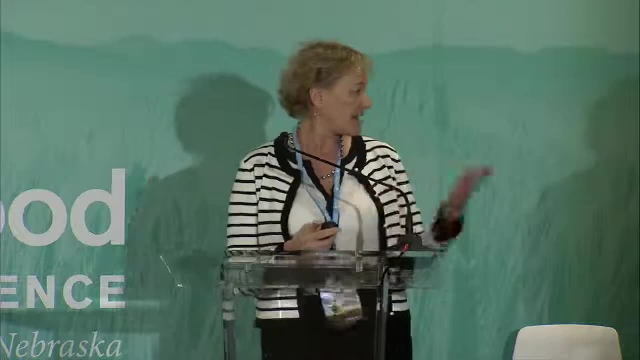 But what's happened is there's been 50 or 100 more illegal wells put in, So groundwater has gone down, So the ability to cope, going forward is challenged, And so we've been looking at and finding that drought is very different in those countries. 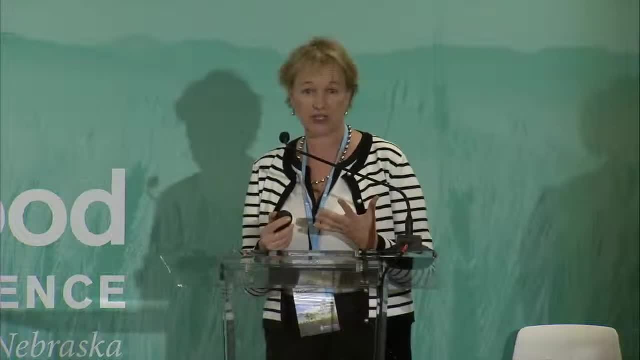 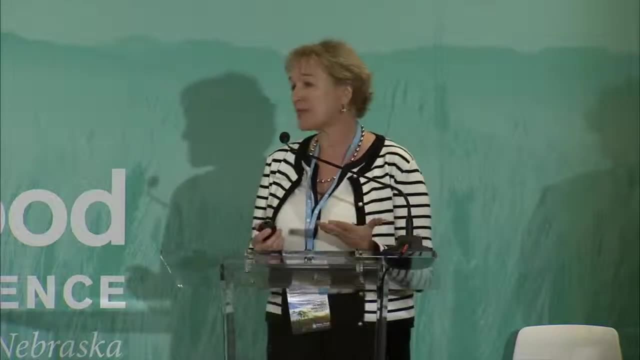 And it's political, One of the big challenges in all those countries. all four countries have received a lot of refugees. For example, in Lebanon the population was 4 million, It's now 6 million, So we have the stressors. 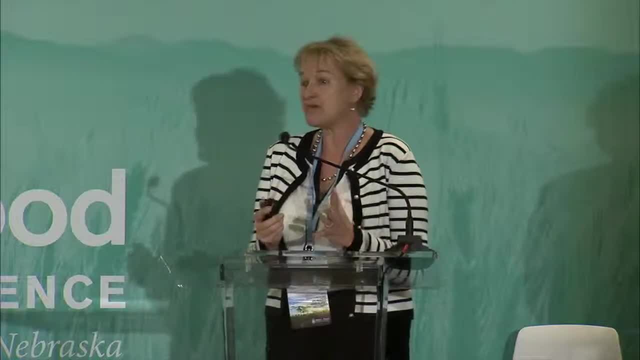 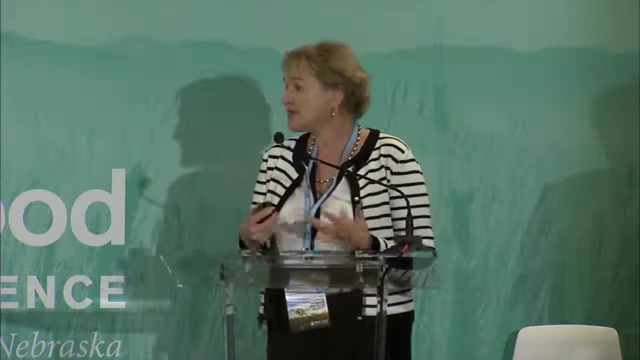 The stressors of very strong input and water insecurity, And then, on top of that, came the worst drought in 60 years. So what have been those challenges? How are we going to do it? We need to look at that And under that, we need to look at the vulnerabilities. 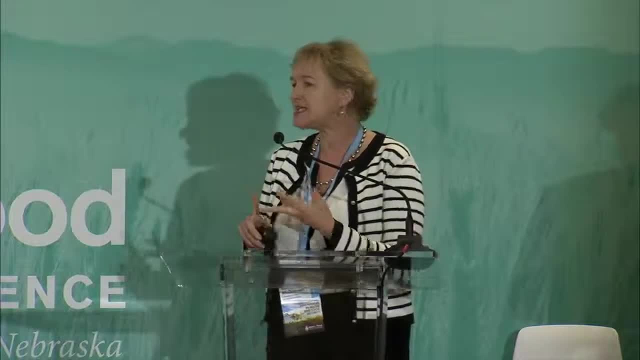 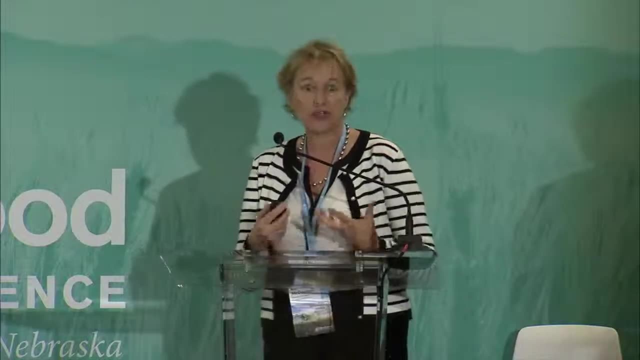 Why is it? Is it access to credit for the irrigation? Is it land ownership? Is it because the young have all gone to the cities to earn the money there, So the elder are struggling with it? We're really trying to understand that. 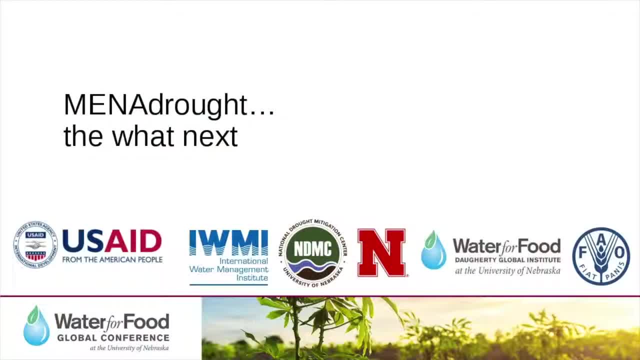 So that was Pillar 1 and Pillar 2, undertaken in Phase 1 of the project. So we've now started MENA Drought Project And this really is the what's next, Because now we have to do with that horrible politics and working together and working on diplomacy. 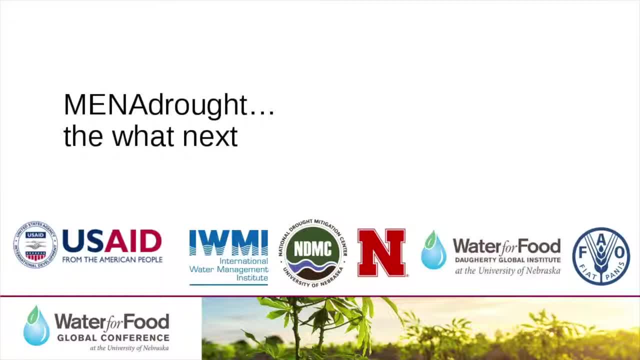 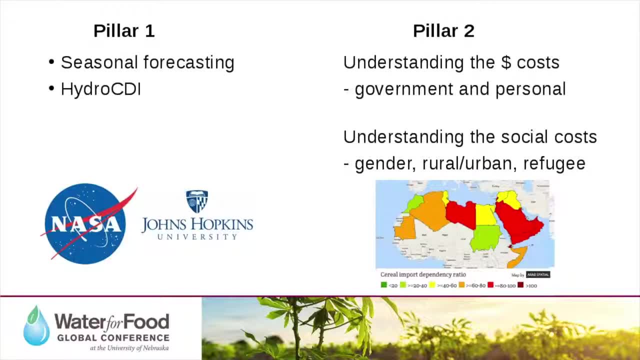 to be able to look at how do we trigger actions. So Pillar 1 is One of the things that came from the farmers and the various organizations- is: we don't need your drought monitor. We already know we're in a drought. 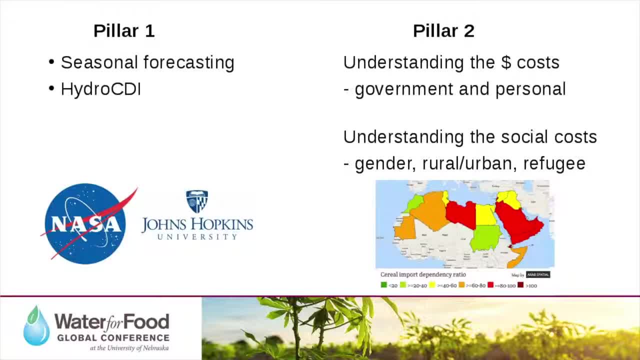 Yeah, We don't need that. But what they're wanting is they want seasonal forecasting. So, on my way back on Friday, I'm back with NASA And USAID has funded a sister project which is helping to produce seasonal forecasting: What's happening in the next 30 to 100 days. 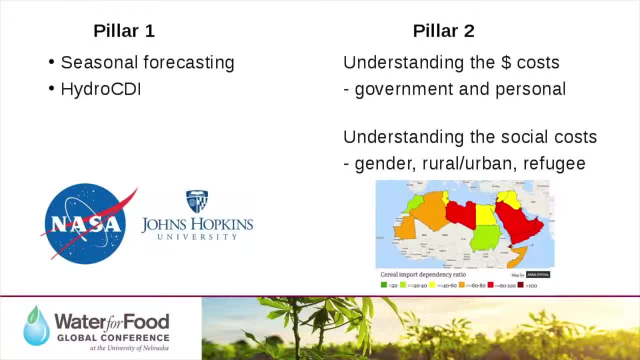 This is very difficult, We can't do it at the moment, But this is what the water manager wants and the farmer wants. the Ministry of Agriculture definitely wants, Because what happened, for example, in Lebanon, in the Bekaa Valley, which is the center for agricultural production in the 2014, is 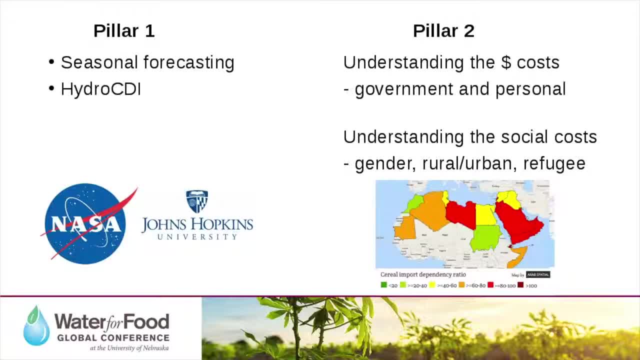 the farmers tilled their land and then the municipality turned the water off, So they wasted their seeds, they wasted their fertilizer and there was no coordination in this. So it's that sort of work In Pillar 2, this is where we need to bring the economists in. 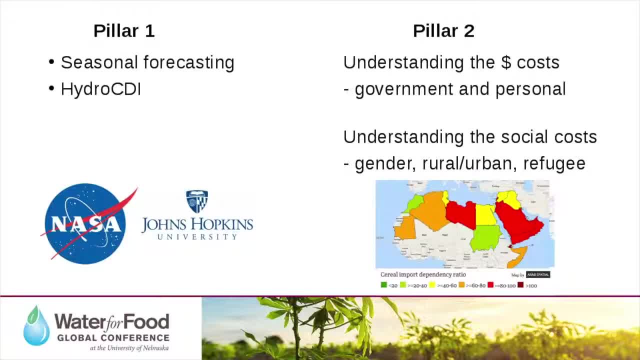 And we also need to bring those that can understand the differences in social costs, exactly what Jennifer Serra said this morning. So if we're going to go to the Ministry of, If we're going to go to the Ministry of Economy and just say 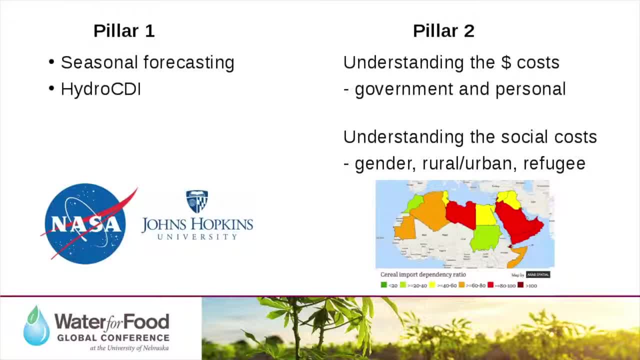 we need this investment, in whatever infrastructure, or we need information or we need new institutions. we have to be able to prove what is the economic cost of the last droughts, And in all those countries we don't know that. We can begin to see that food prices went up and it costs the government a lot more in subsidies. 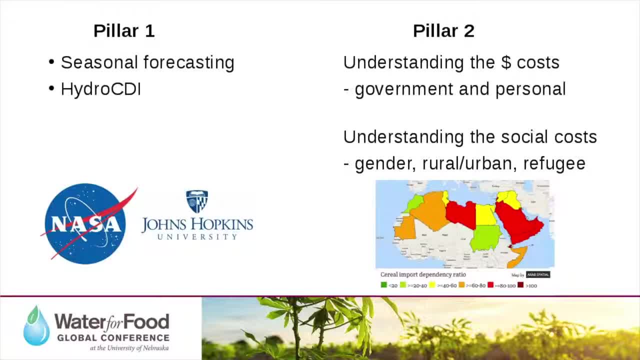 subsidizing food or importing wheat, whatever it might be. We don't know what it is, But if we're going to put forward a project or some sort of planning, we need to be able to put in front of that. Minister of Economy. 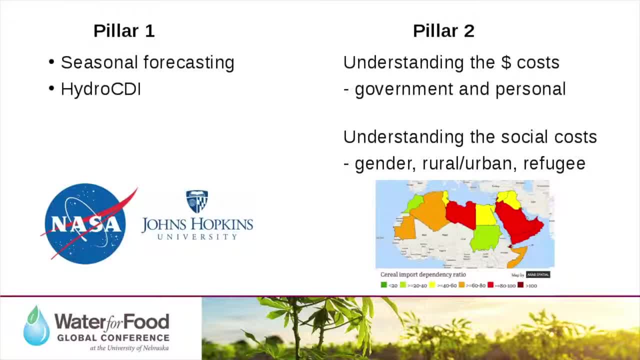 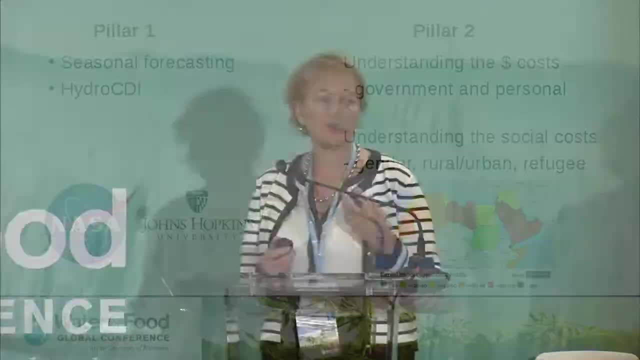 this is how much we can save if we bring in proactive drought management And in terms of the social costs we have the difference in gender, age, rural, urban. the way droughts are experienced is very different. For example, if you're living in an urban area during a drought. 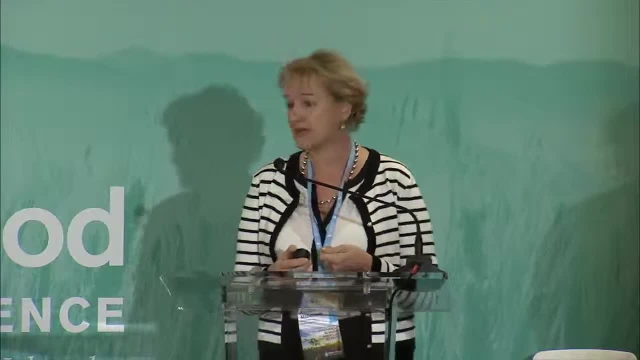 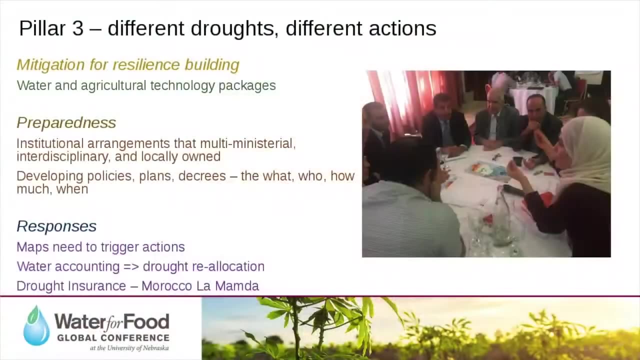 the water isn't running in your taps, so you have to buy it from the tanker. So you're often paying 10 times more for your water than in a non-drought year. And then the pillar three is the very difficult one that Mark talked about. 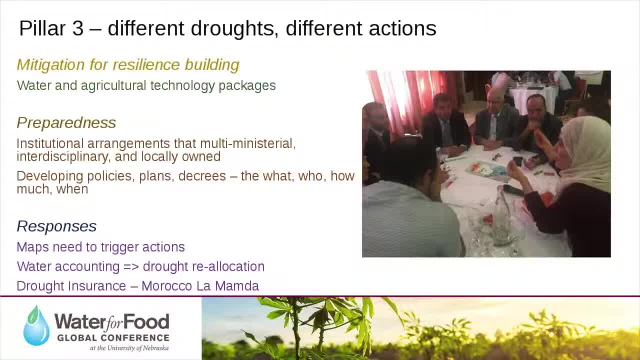 This is mitigation, preparedness and response. In many of the countries, for example Lebanon, there is no official declaration of drought. We can't say there is a drought. therefore, we need to trigger these actions. So this is part of the work we're dealing with. 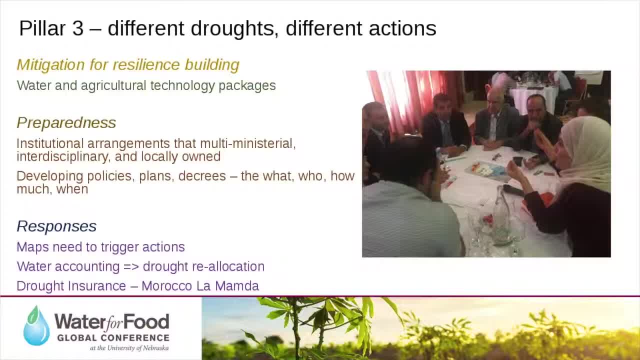 We're looking at water and technology packages, So my colleague here, Petra, is going to be helping us design resilience building. How can we bring in species that are more resilient? How can we bring in water technologies that are going to save water? 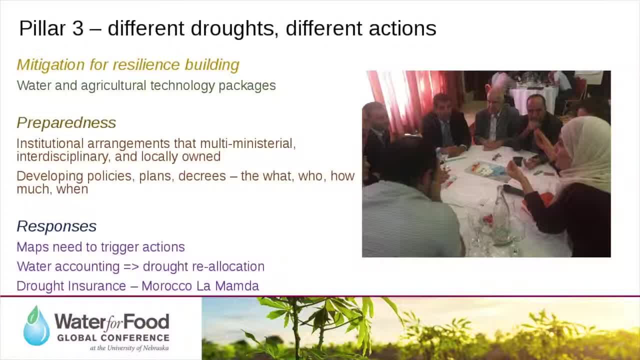 so then, during those droughts, we can continue that We want to look at institutional arrangements. Trying to get the Ministry of Agriculture and the Ministry of Environment and the Ministry of Water together is difficult, but to then agree: when the next drought comes, you will do this, you will do this and you will do this. 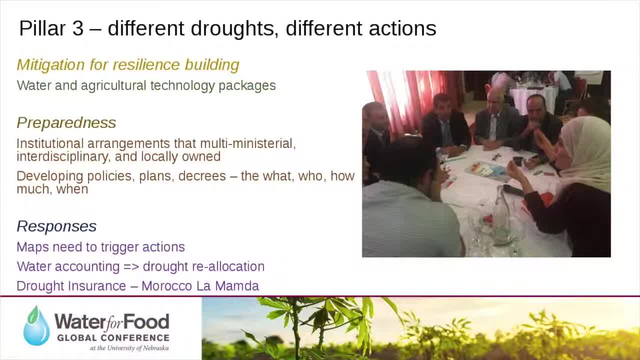 and have the finance and the budget and the resources to go with. it Needs endorsement from prime minister's offices or ones like that. So this is what we're working on a lot at the moment, And what we're also trying to look at is preparing plans now. 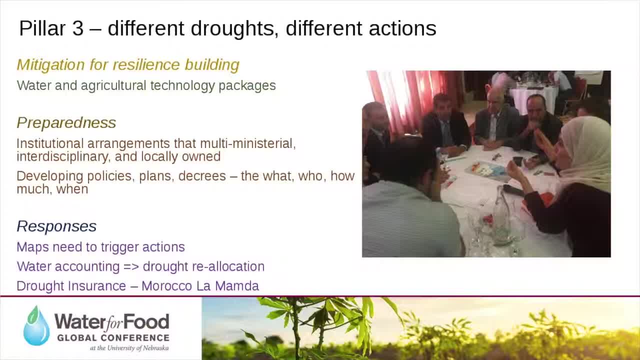 in a very calm, non-political way, because what happens when the drought comes? the newspapers are involved, there's lots of finger-pointing, It becomes a highly politicised session, And so we don't have that calm rationality. So one of the things we're looking at is: 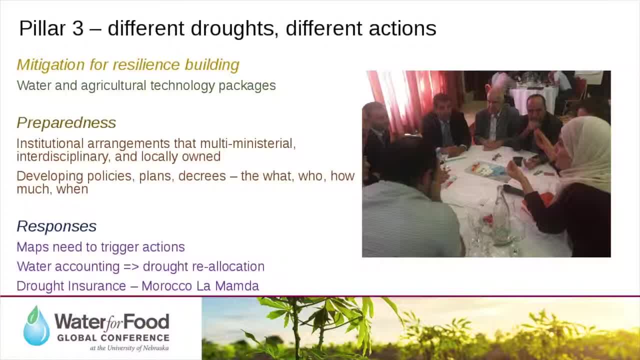 can we use water accounting? Because if we can say where the water is going to now and who gets it and what type of water from those many different sources, we can then agree, when the next drought comes, where we can turn that water off from. 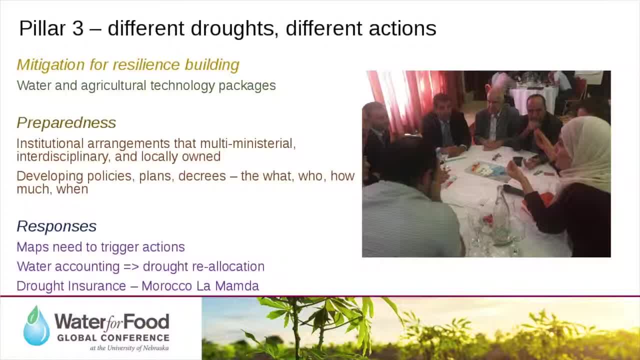 So this: we can see that we are moving on to the what's next. What Nebraska is always constantly telling us is: you have to take it slowly. you have to build the very strong foundations because we need to make sure that at the end of these next three years, 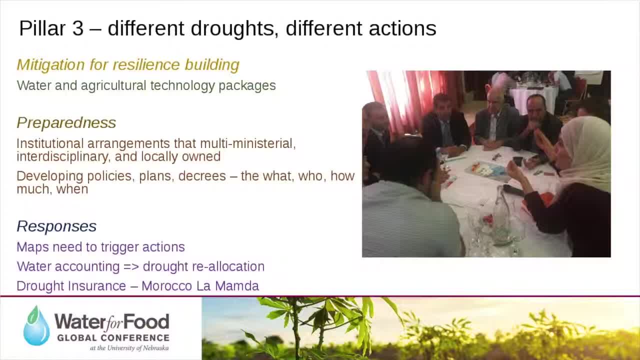 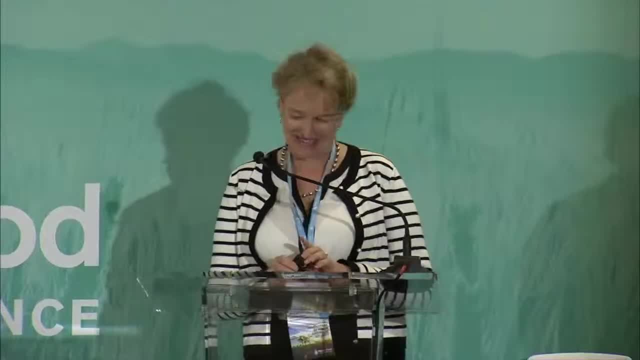 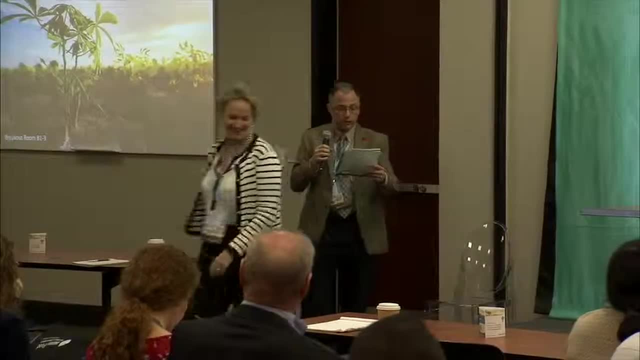 in those countries, there are policies and plans in action that will then be fit for purpose and used when the next drought comes. Thank you very much for your attention and for inviting me here. Thank you, Dr MacDonald. So our fourth speaker today comes from India, from Delhi. 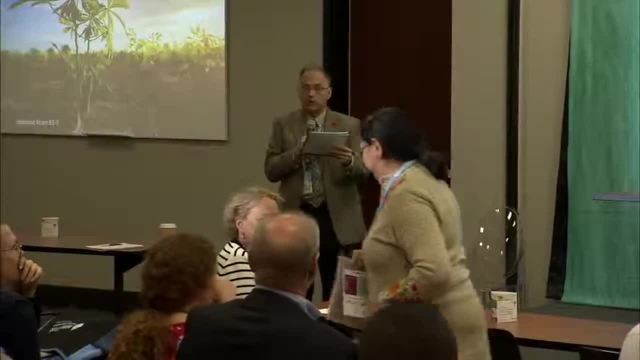 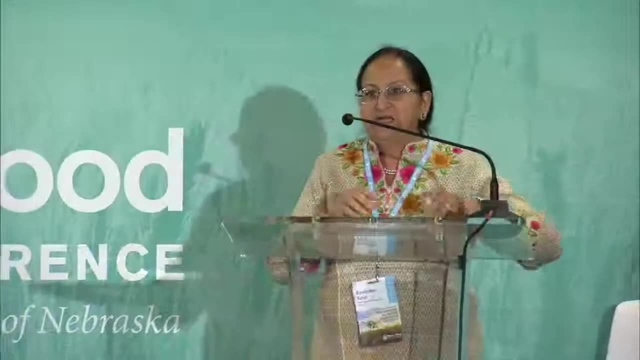 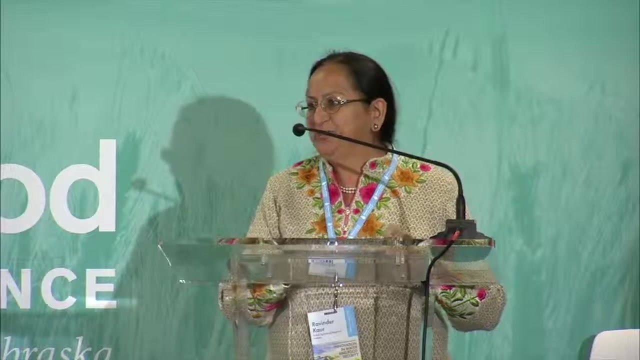 Dr Ravinder Kaur is the Principal Scientist at the Indian Agricultural Research Institute And I've had the pleasure of working with Dr Kaur for many years. Welcome, Dr Kaur. I'd like to extend my warm greetings to all of you and my appreciation to the NDMC. 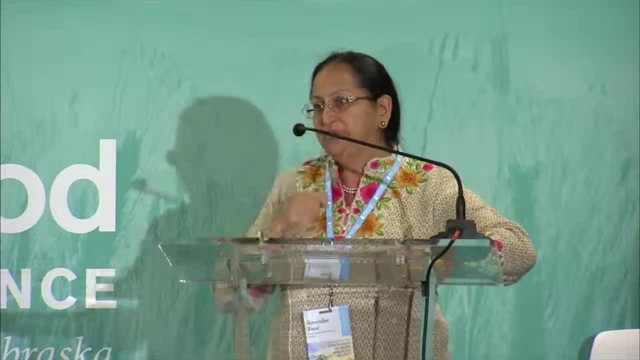 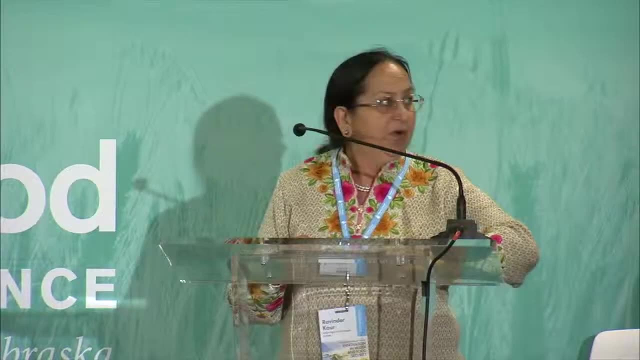 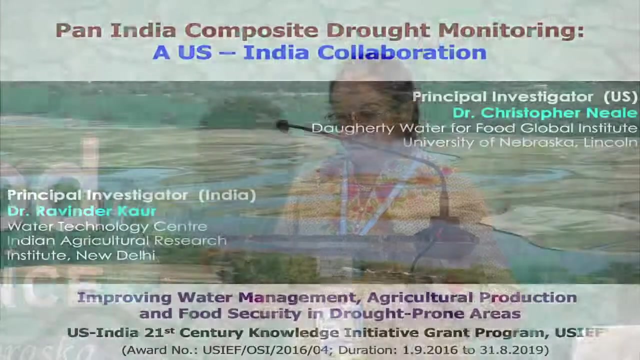 and the University of Nebraska-Lincoln for giving me this opportunity for being a part of this conference and to share some of our success stories on the Pan-India Composite Drought Monitoring, which is basically a US and India collaborative effort. Well, as you can see on the slide, 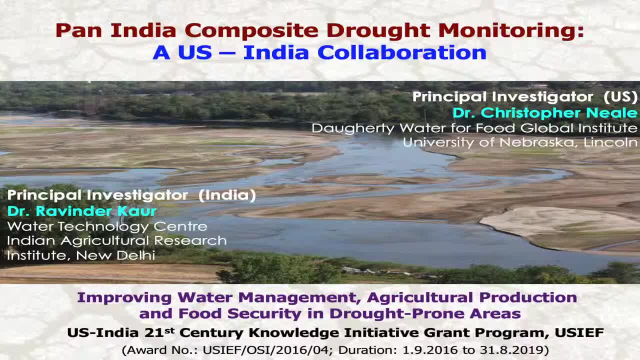 this particular initiative was taken up under a USIF-funded program on improving water management, agriculture production and food security in drought-prone areas in the year 2016,, with Professor Dr Christopher Neal as the Principal Investigator from the US side. 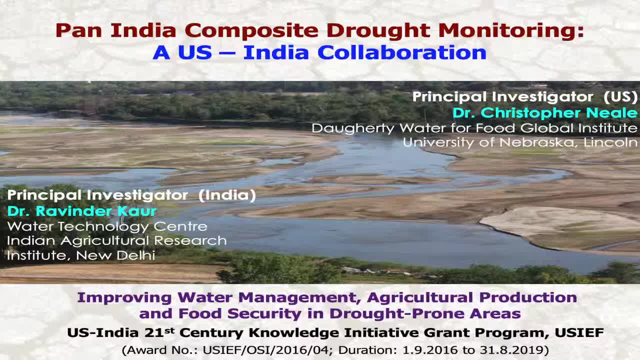 and myself as the Principal Investigator from the Indian side. But that doesn't mean that the work has been done only with these two people. I haven't put the name. There's a long list of team members, both the scientists and the students. 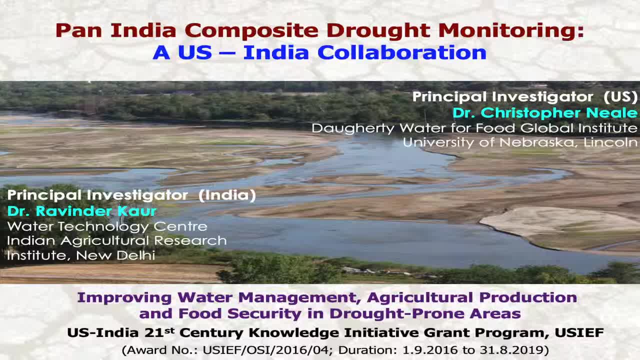 who are responsible for this success story to build up in such a short span of time. So we have folks from the NDMC Center, Dr Mark Suboboda and Dr Hayes and their team, and also a team of scientists from the Remote Sensing Center. 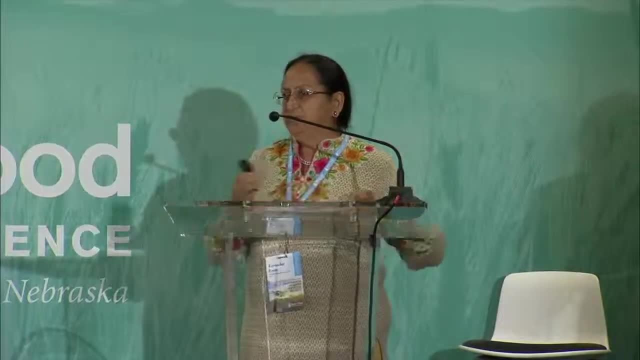 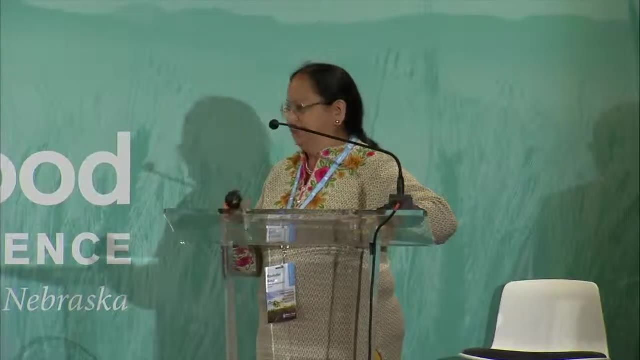 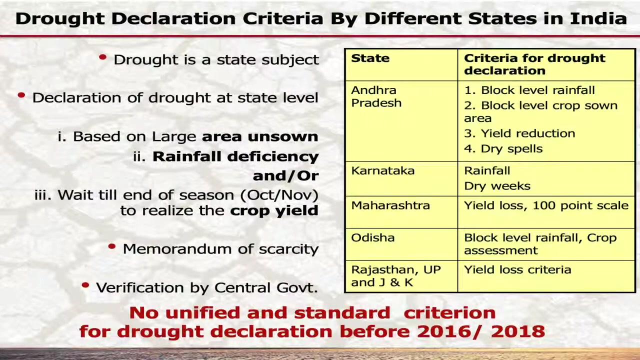 of the University of Nebraska-Lincoln, And we have folks from Water Technology Center, from the Indian Agriculture Research Institute and also from the Division of Agriculture Physics. Well before I come to our success story, I think it's very important for all of us to understand. 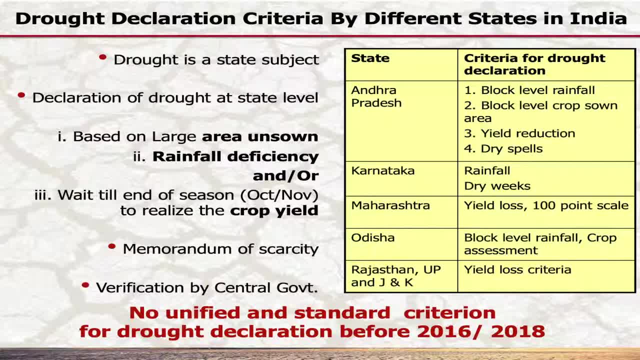 what is the process of drought declaration in India. I'll not be very elaborate because I've been allocated only 10 minutes. So, broadly, if you look at this slide, you will realize that drought declaration in India doesn't follow any rules. It doesn't follow any unified or standard criteria. 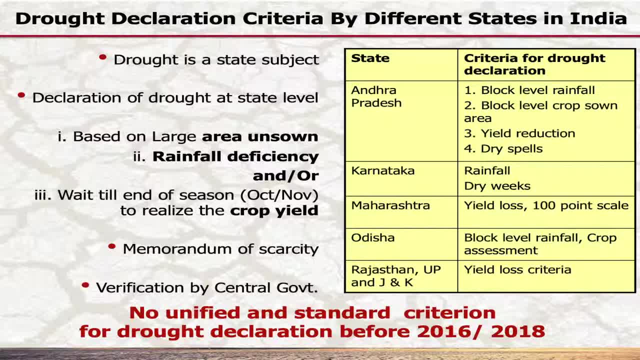 If you go from north to south and east to west, there are different criteria which are used to declare drought which is a state subject, because water is a state subject in India. Basically, the declaration of the drought from state to state depends upon the area unsown. 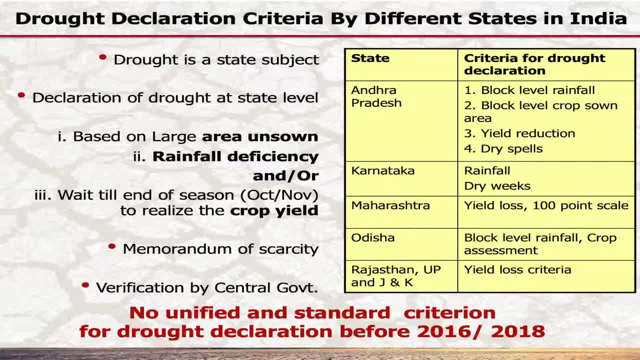 the rainfall deficiency and the crop yield deviations. So there are certain states which only make use of the area unsown rainfall deficiency and there are other states which make use of area unsown rainfall deficiency, as well as the crop yield deviations, to declare the drought. 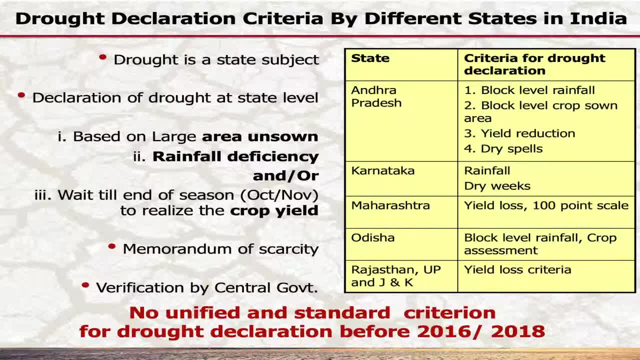 So it's not a common standard procedure of drought declaration. And once the drought is declared, then the memorandum of scarcity is passed on to the center. The centers, the states, are encouraged to use their state disaster relief fund to mitigate the drought, But if the drought is of a vast extent, 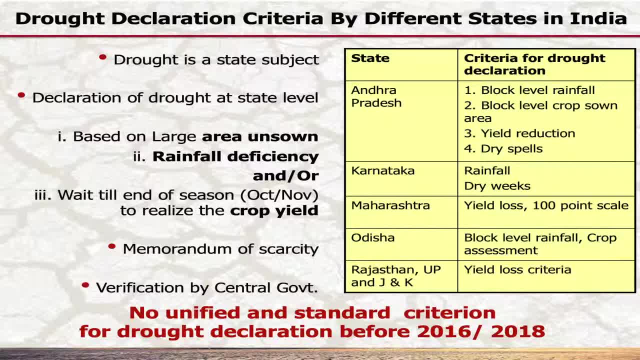 if the states do not have enough funding to cope with the situation, then they send a memorandum to the center and then the center sends the team, the verification team, on ground, which verifies whether it is a real drought or a fake drought and then, based upon what is the extent of the drought, 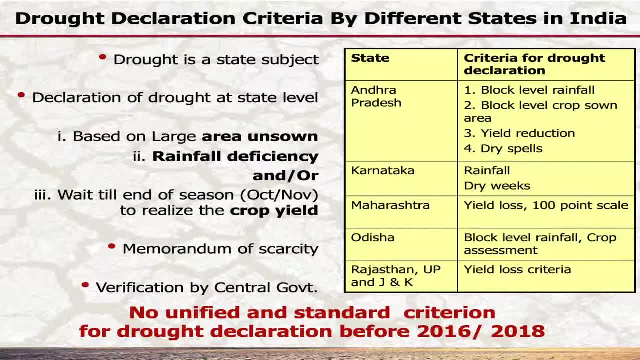 the team finds out and then submits the report And then, based upon that report and the verification process, the center releases the fund. So it used to be previously a very long drawn process, so with a large lag time for the response to take place. 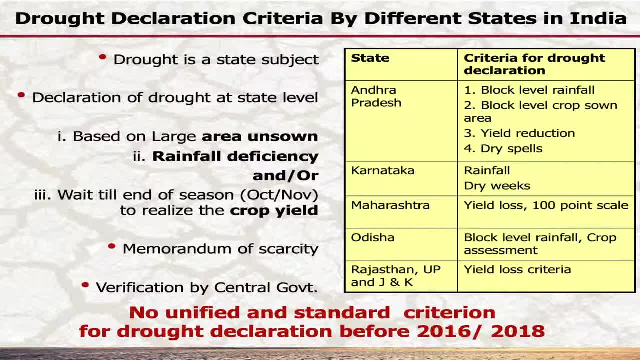 And, as I will proceed, you will see that what actually was happening on the ground, whether it was a fake drought declaration or was it a real drought declaration and things like that. So they will become clear Now. it was only after 2016. 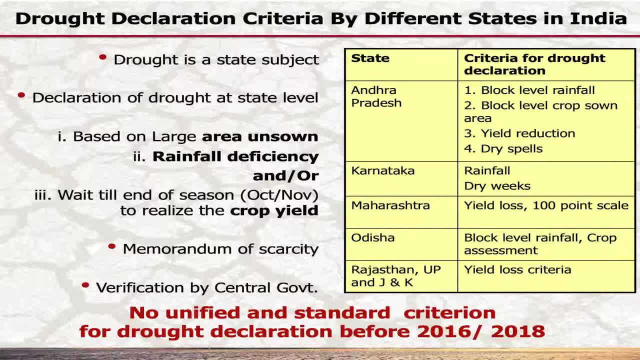 that actually the standard drought monitoring protocol. the need for that started in the year 2009,. so government started feeling we should have a standard procedure for drought declaration. So certain standard protocols were drawn but they were taken very casually by the states. 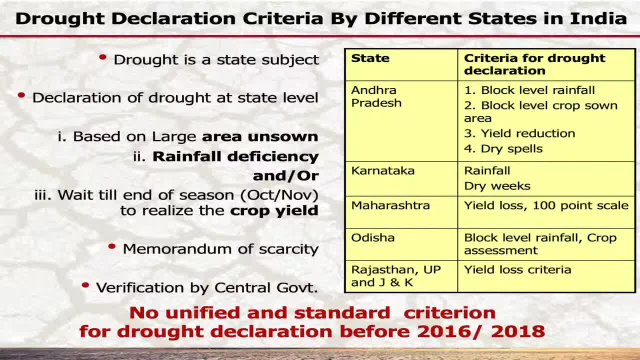 because these were not mandated to happen on ground. Then, in 2016,, a drought manual was taken out by the government of India, but still they found that the states are not following the procedure indicated in the drought manual, So a brainstorming was held. 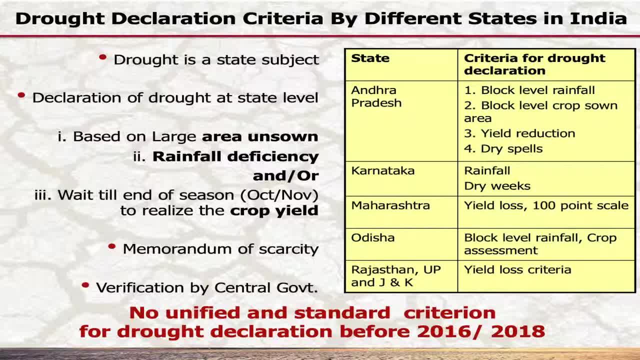 and so the stakeholders, that is, the states, which are normally the chief secretary, his principal secretary, his very senior policy makers. they indicated a lot of hitches with respect to the use of that strategy, So those hitches were removed. The protocol was revised in 2018.. 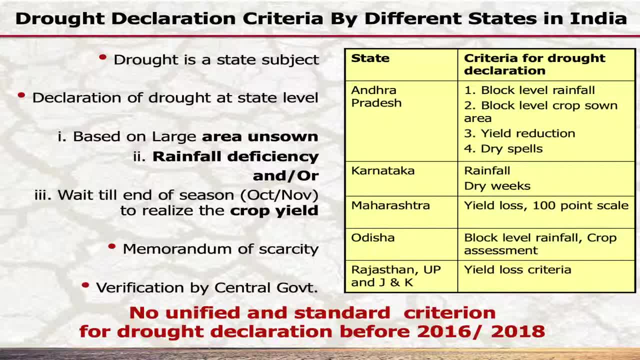 Another drought manual was brought out, but this time the government said: no, enough is enough. You have to follow this drought monitoring procedure. If you follow and you give us your memorandum- I mean declarations- then we give you funding based upon the verification. 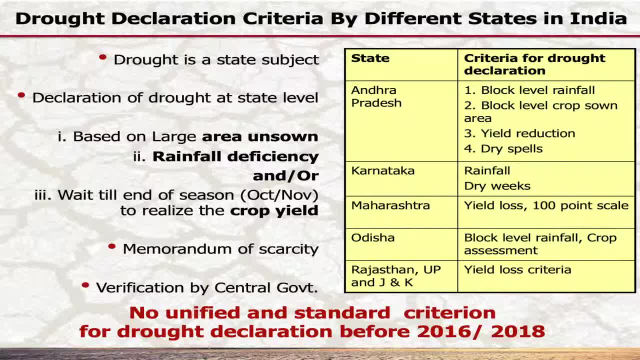 If you don't follow this procedure, we don't give you So. since 2018, which is not very far, which is a very early affair, a recent affair- that this procedure started taking place. Now, what is there in that protocol? 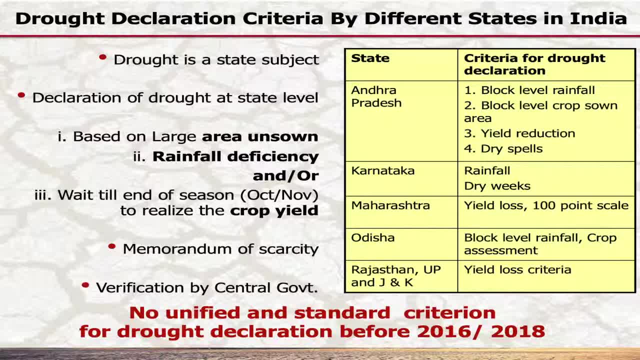 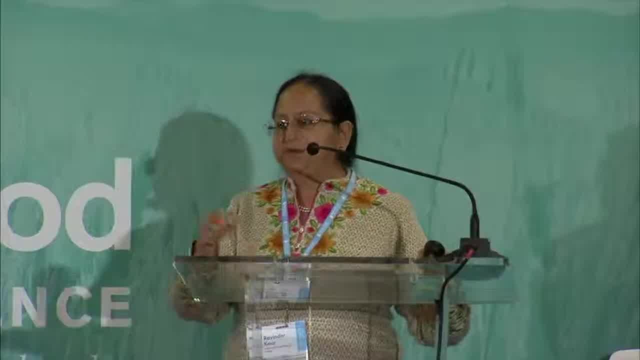 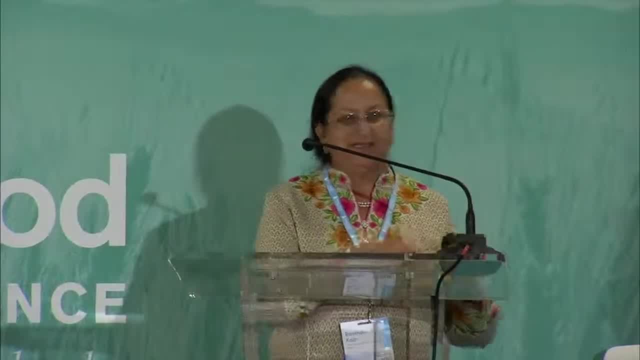 I would quickly like to mention The 2018 Drought Manual. Protocol states that each state has to first of all monitor the precipitation-based indices. There are two of them. I'll not go elaborately on them, So these precipitation-based indices. 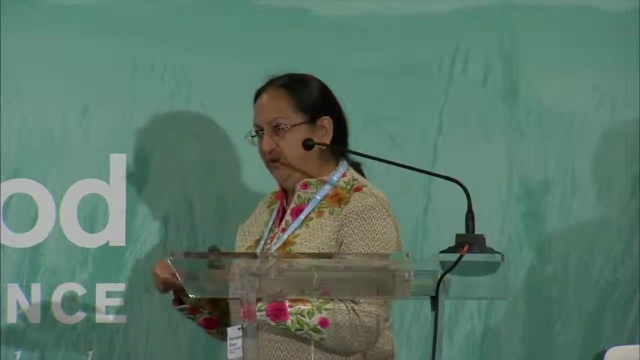 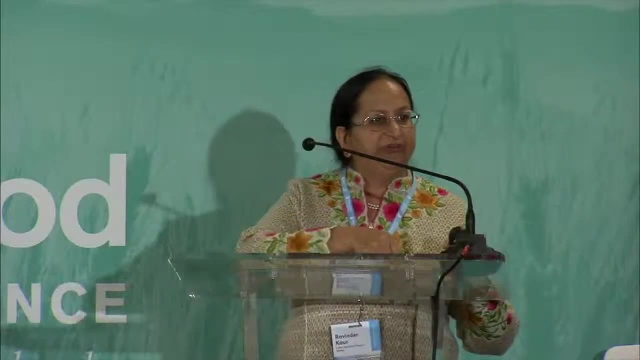 they set the trigger whether the drought is there or not, yes or no, And once the yes is there, these triggers state that yes, the drought is there. then they start monitoring the impact of that drought based upon the crop area. unsown. 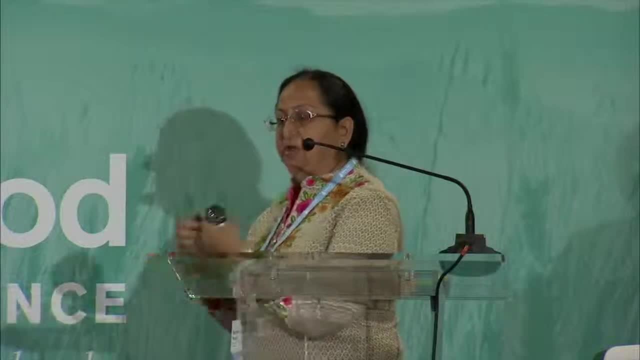 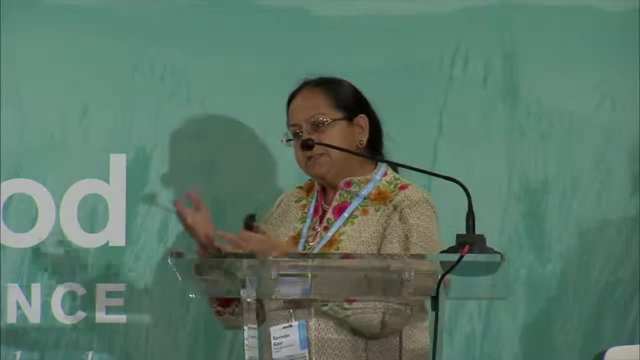 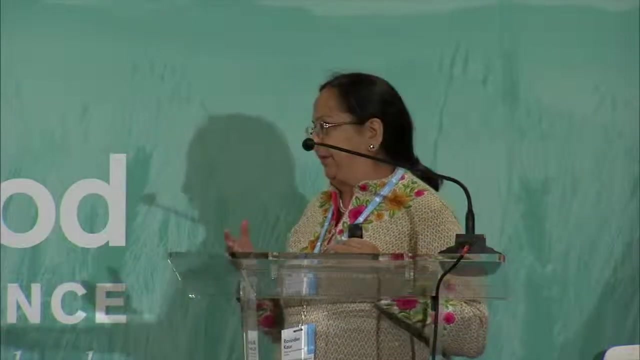 the vegetation condition, the soil moisture condition or the hydrologic conditions, depending upon what level of data is available with the states. There might be certain states where soil moisture would be monitored, which is a very hard thing to be spatio-temporally being monitored. 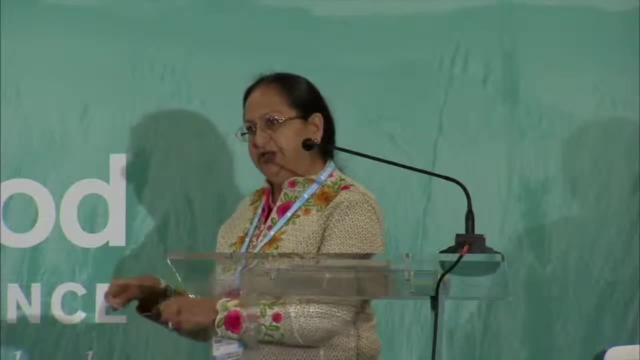 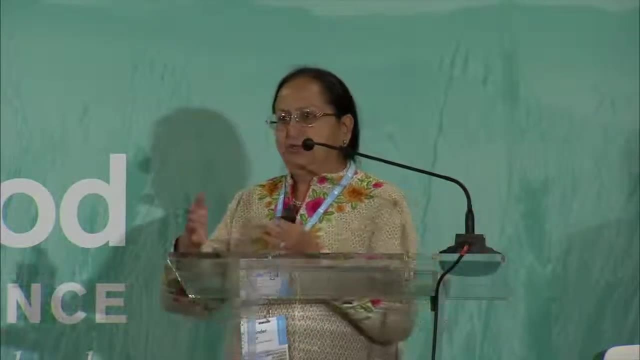 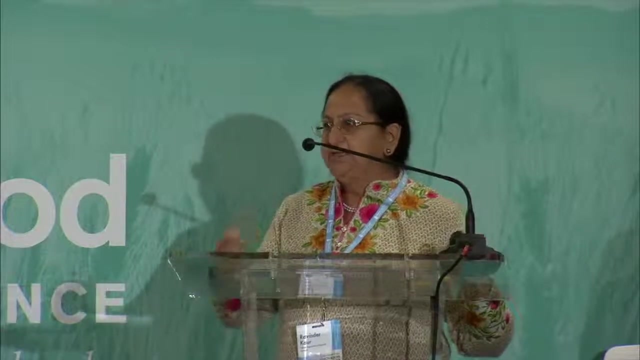 So those states they make use of that soil moisture condition index also to assess the impact. otherwise the others will stop just at the crop area unsown and the vegetation condition and things like that. So the basic if you look at this protocol. 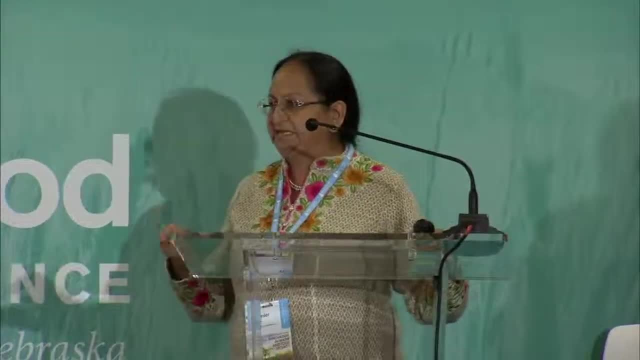 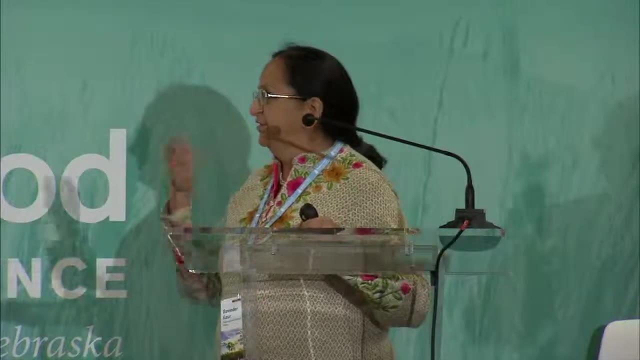 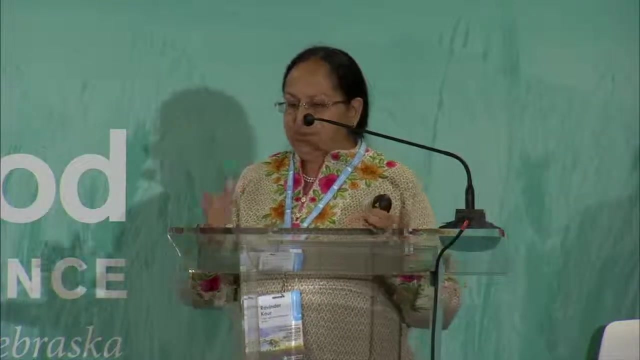 it makes use of both the remote sensing as well as the ground station-based data for setting the triggers and for assessing the impact of the drought, for declaring the drought and its magnitude and extent. Now, because it makes use of both the ground station-based data, 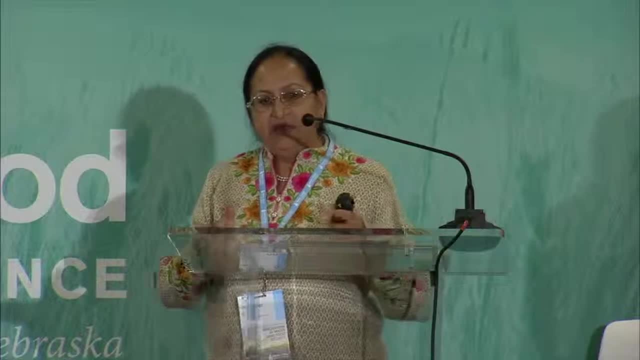 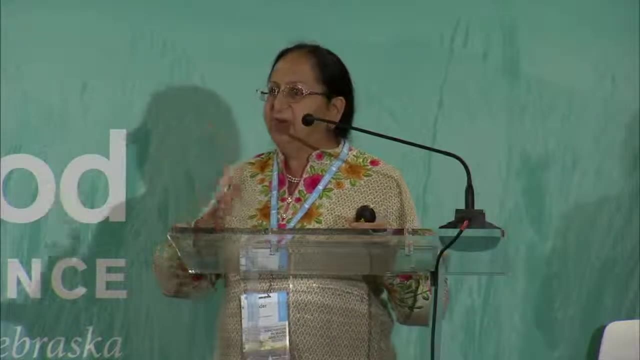 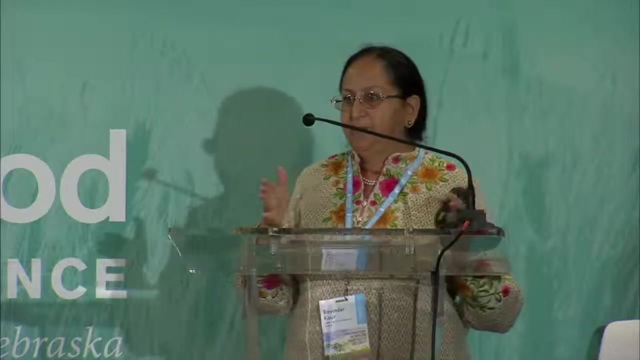 and the remote sensing-based data, and the thresholds of each of these indices, which are generated through the use of this data, are set by a means of stakeholder participation. so for the whole approach has a lot of subjectivity to it And therefore, 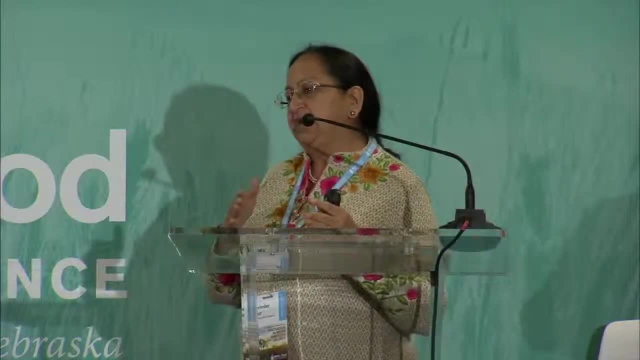 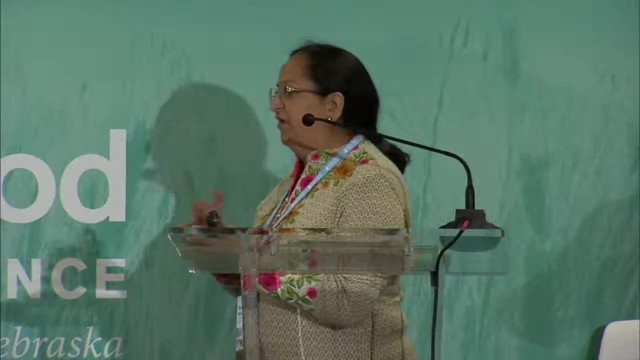 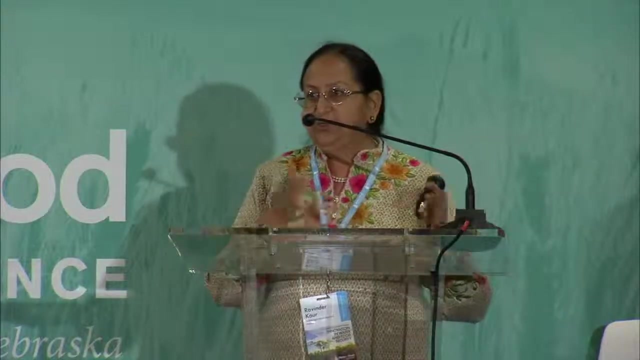 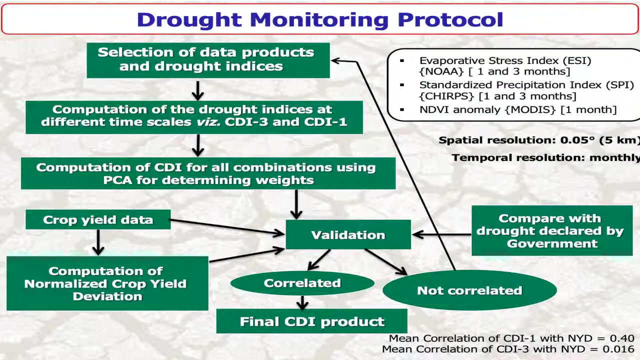 it adds to the very limited practicality and practical application of this protocol across the states with varying data gauging capabilities and as well as the data gauging interests. So therefore we decided that why not to develop an India Drought Monitor under our memorandum? 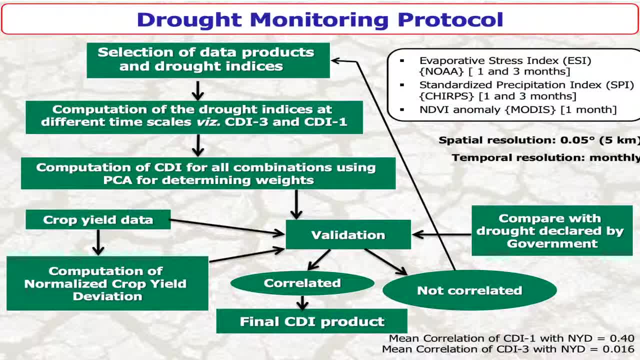 of understanding with the University of Nebraska-Lincoln and under the able leadership of the NDMC- which is, you know, the National Institute for Drought Monitoring- and develop a technology which is more objective, which makes use of the satellite-based data products. 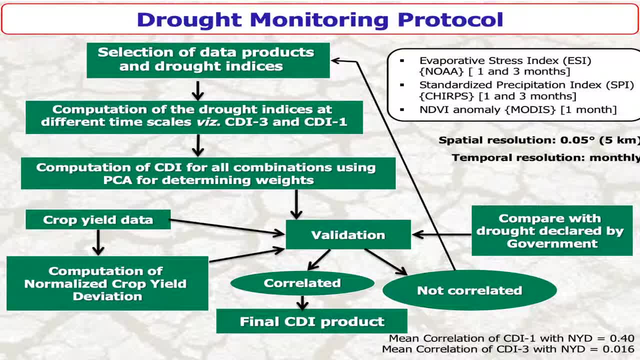 with the limited subjectivity added to them through stakeholder participation, because each time the stakeholders are invited to set the, I've myself been in many of those meetings and I've seen them, you know, dictating the values in order to tweak a worse condition of the drought. 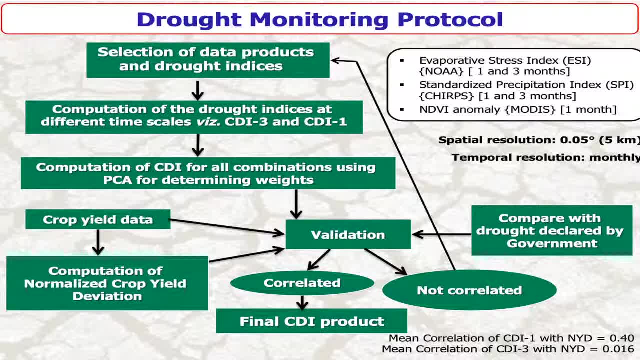 a realistic condition of the drought just to make the state look, you know, drought-hit. So we wanted to remove all these things and we came up with this protocol. I'll not be very elaborate on it. Basically it makes use of: 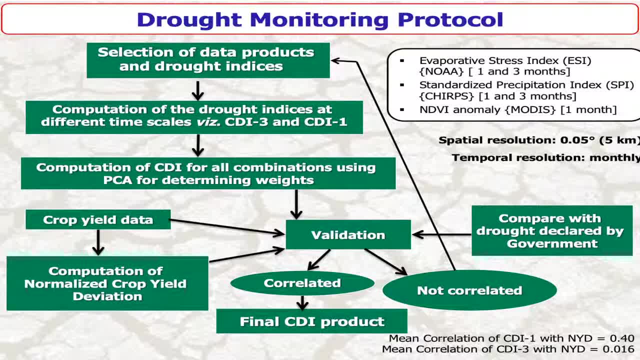 the meteorologic indicators, the biophysical indicators and the hydrologic indicators, all of which are generated through satellite-based data products, And to generate a final product called Composite Drought Monitoring Index. And what we did is basically right now. 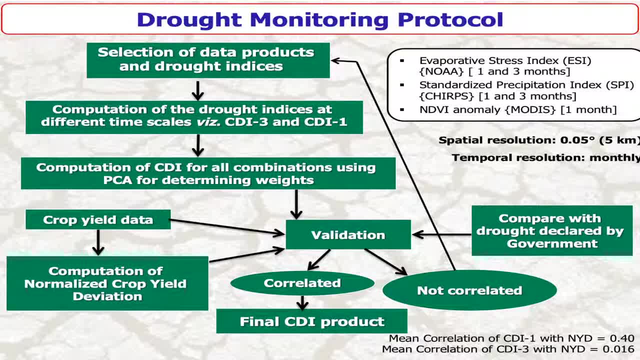 we are only making use of the Standardized Precipitation Index, the NDVI and the Evaporative Stress Index, these three of them each representing the meteorologic, agricultural and the- I mean the biophysical and the hydrologic- drought conditions. 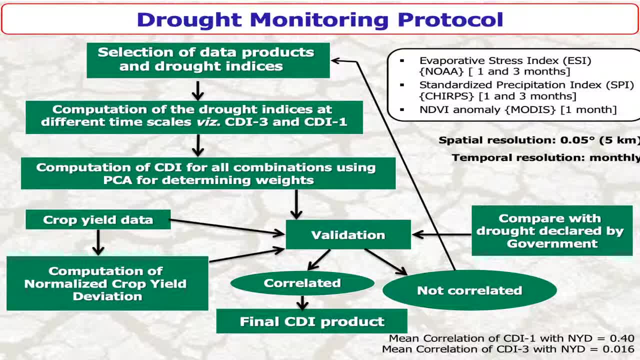 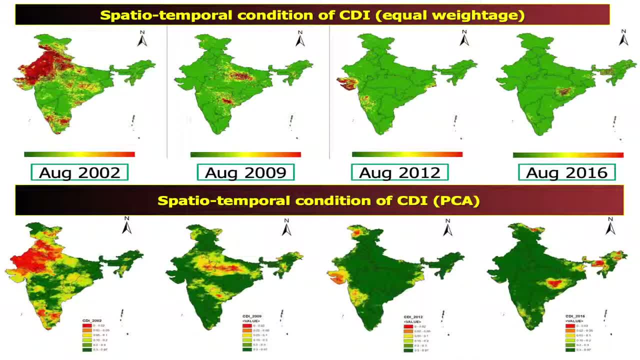 And then generating the CDI product. in order to generate the CDI product, we tried to investigate the satellite use, the satellite products at varying geospatial resolutions, Because we wanted to find out whether a 500-kilometer product or a 1-kilometer product. 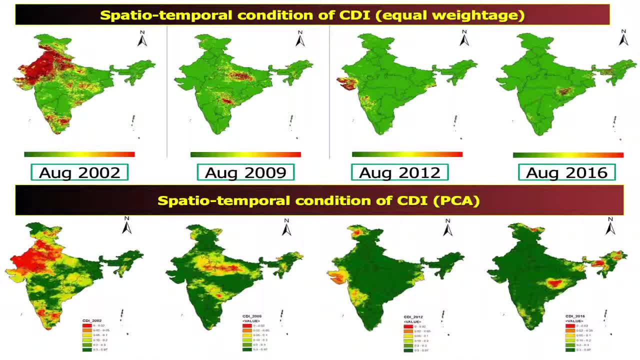 or a 5-kilometer or a 500-meter product? what should be utilized for accurate drought monitoring as far as Indian subcontinent is concerned And, besides this, what should be the cumulative drought index duration- whether we need to generate a monthly product. 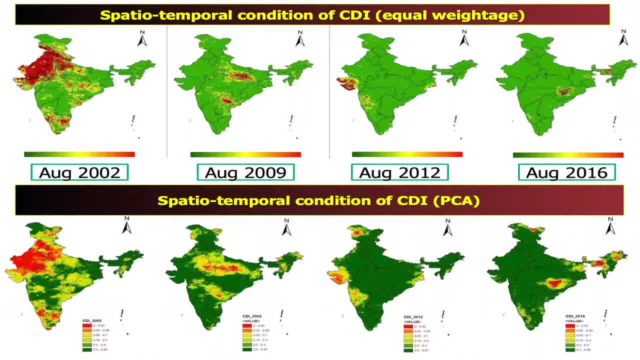 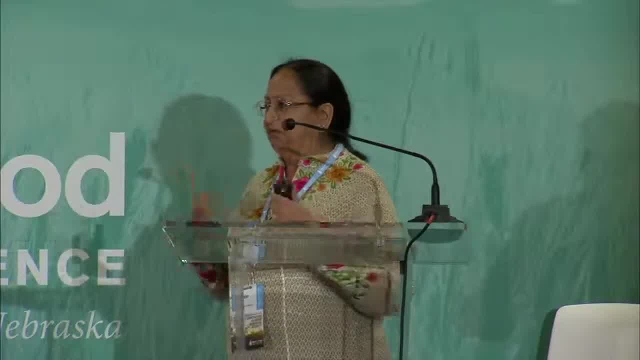 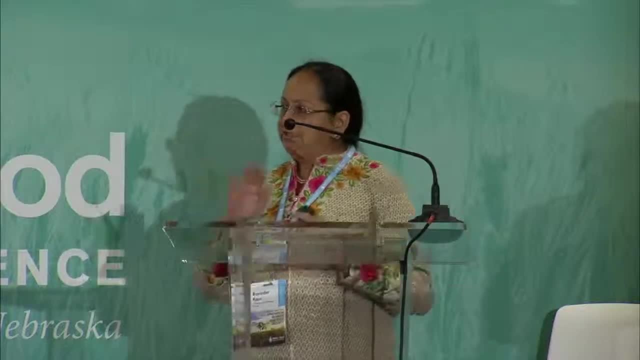 or a 30. I mean a 15-day product or a weekly product, what would be good? or a 3-month product or a 2-month product. So we tried all these, we did a lot of R&D and we found that. 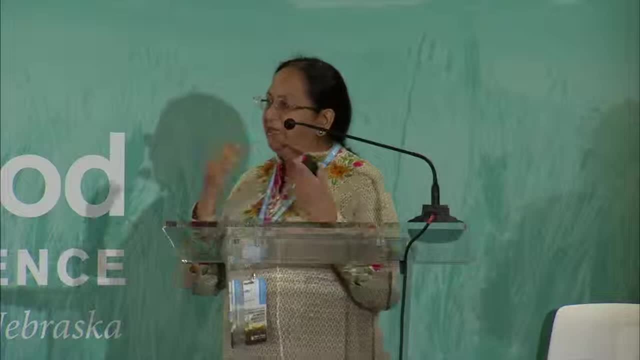 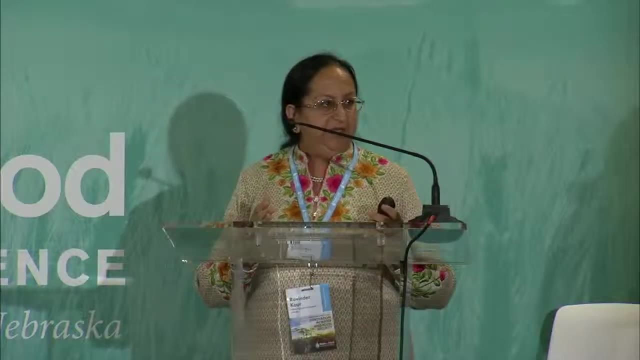 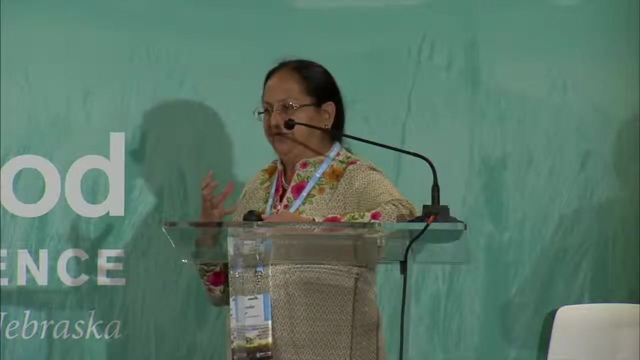 it can be applied at varying spatial resolutions. Whether I apply it at 500-meter or 5-kilometer or 1-kilometer, it gives the similar results. Only the coarseness or the fineness of the results will be different. 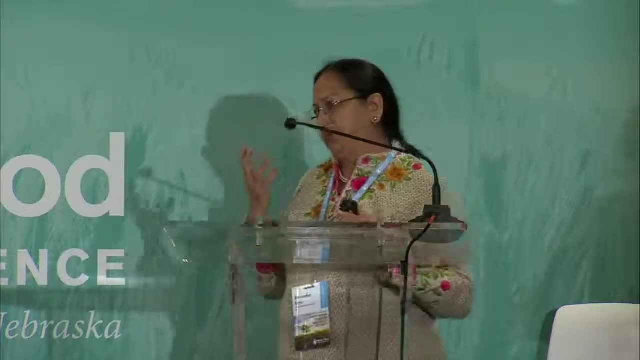 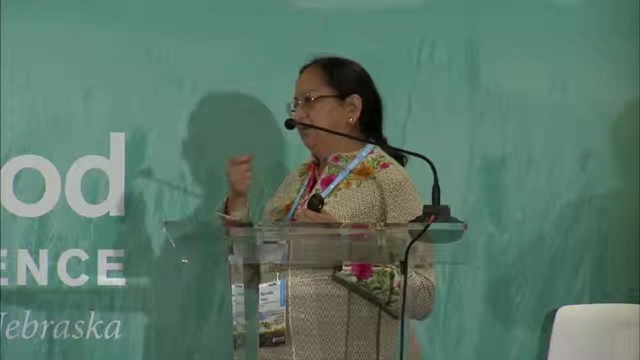 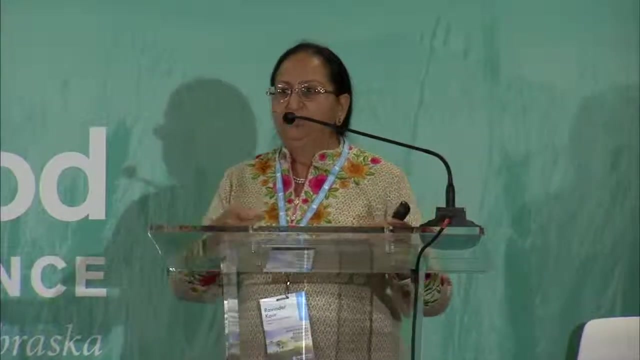 but the pattern doesn't change much, and so it has the capability to give the near real-time drought monitoring. Second outcome of this investigation is that, in comparison to the 3-month product, the 1-month product performs better, And we are quite hopeful. 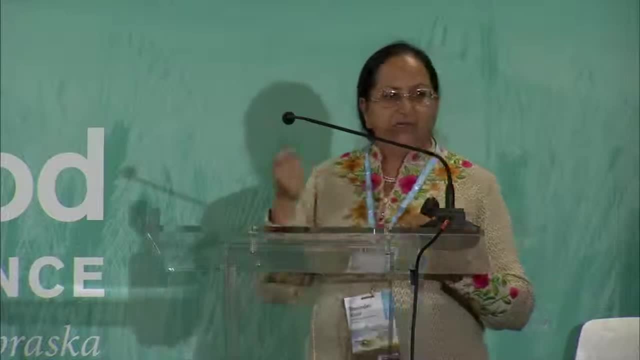 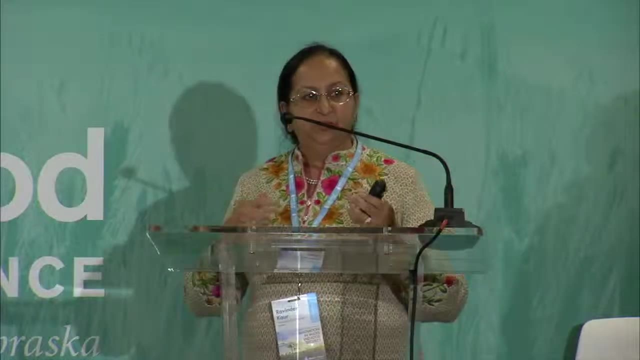 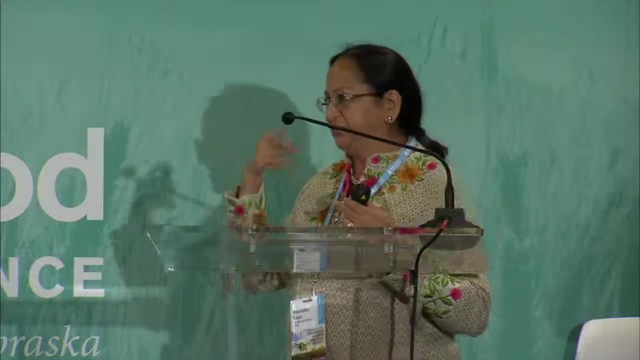 that if in future we want to do a forewarning, then we can even generate a 15-day product or a weekly product. but that means adding to more satellite-based data product availability. So time doesn't permit me to go into all those inter-cases. 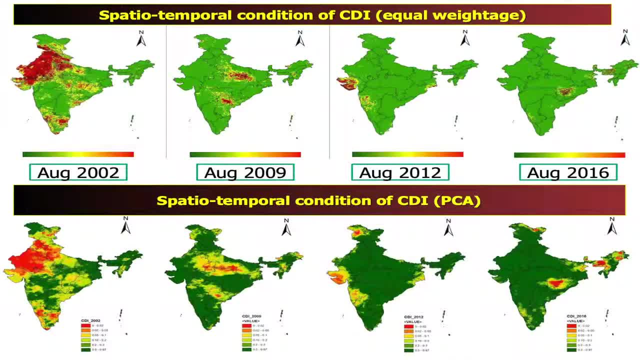 of the research, but it does permit me to see the results. So we did that and we applied. besides this, we integrated all these three indicators by giving the we didn't want to give. the weights are unknown, so we tried different methodologies. 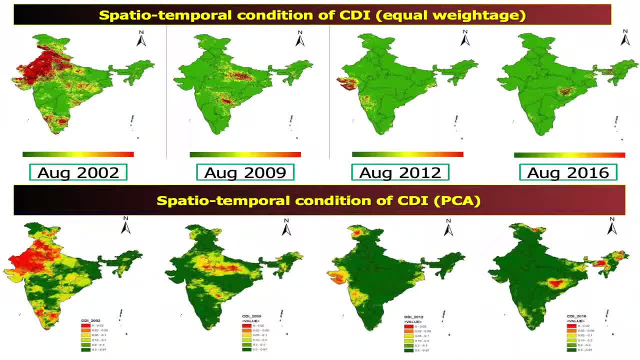 We gave equal weighting. we tried equal weighting method with the principal component analysis methodology. So if somebody runs it or somebody else runs it, the results should be same And that was a basic need for that. So we found that, as compared to the equal weightage, 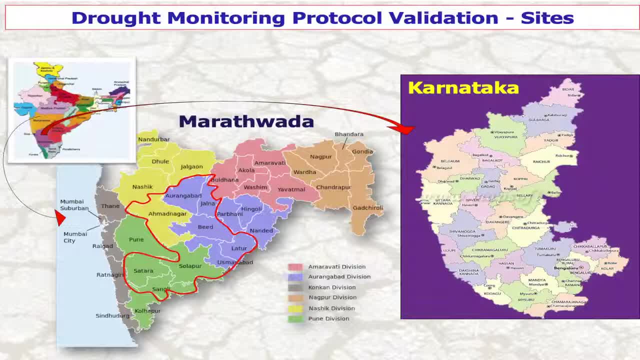 the principal component analysis methodology seems to be giving very good results, So that was a very good hope for us to go in the forward direction. So we applied the tool, as you had seen across India, and we also applied the two main indicators, the single versus the composite. 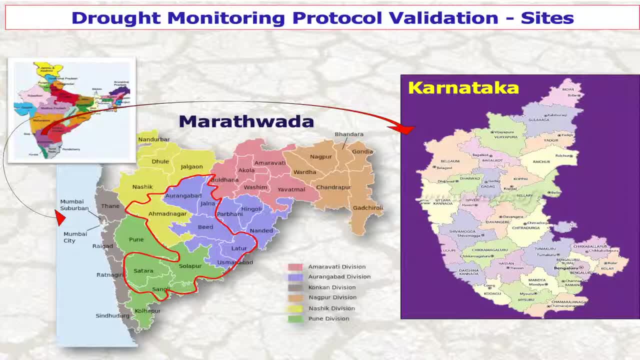 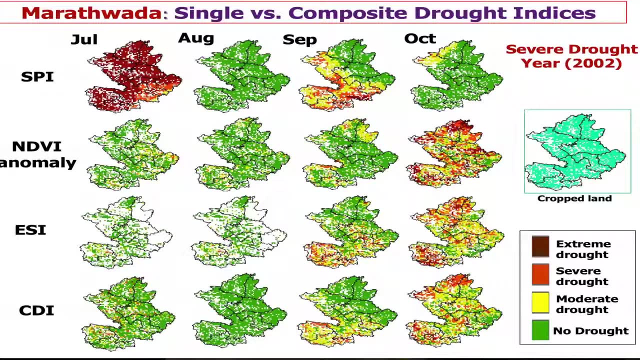 drought index, which is the one that is the most common in the country, And these are the Karnataka and the Maharashtra And, as you can see in the map, these are located right in the southwestern part of the country. So these are some of the products. 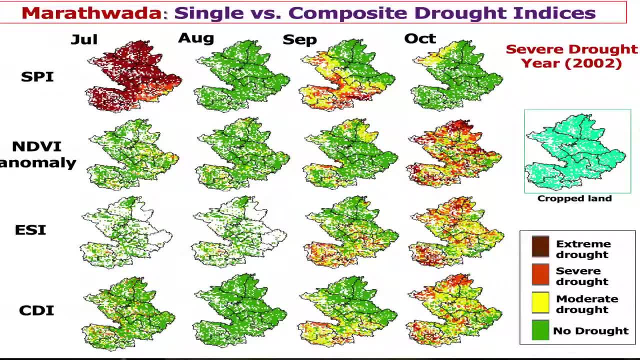 we generated for the Maharashtra or the Marathwada region, It appears as if there are no more drought-like conditions. But if you look at the agriculture biophysical indicator, NDVI, or the hydrologic indicator, ESI, and again the CDI, 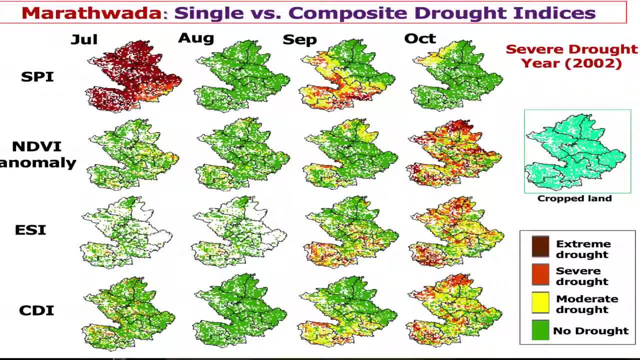 the composite drought monitoring, composite drought index. they all show that the area has already been hit by some degree of drought. So the point which I want to mark here that the single indicators are not able to really simulate the actual drought conditions on ground. so therefore, 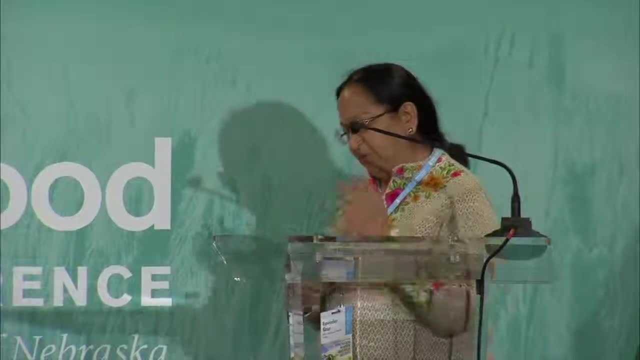 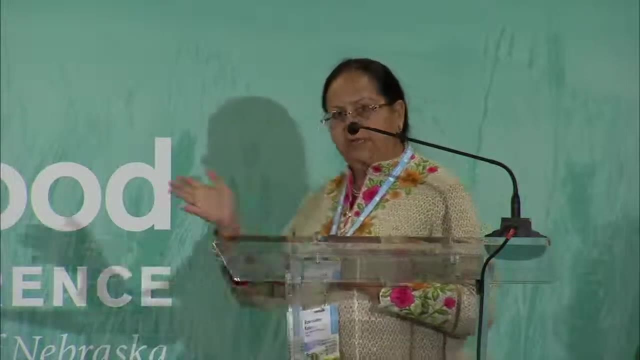 it is always better to have the composite drought indicators And if you look at, compare the single biophysical single ESI and vis-a-vis the CDI, again the pattern and the spatio-temporal distribution of the drought also varies. 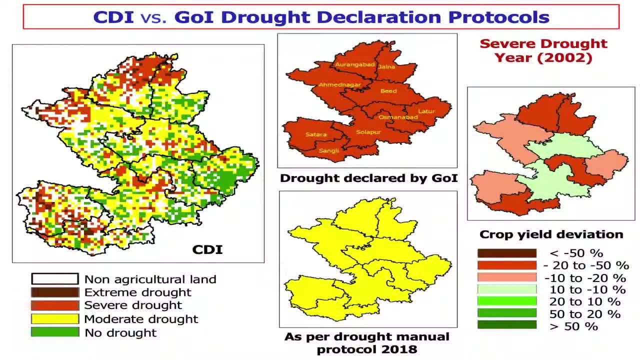 So we started comparing the CDI with the drought declarations by the government. So this processing we did for 16 months, 16 long years, across India, from 2001 to 2016.. And then we started doing validation on two of the most. 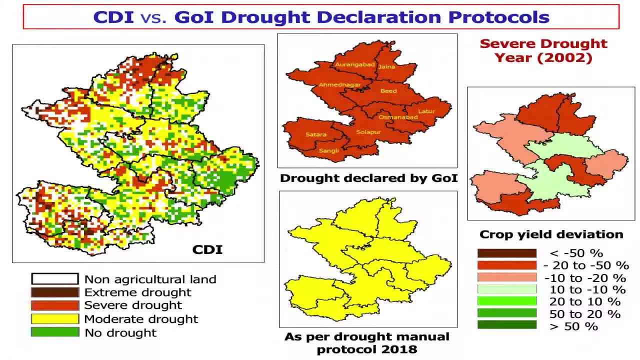 drought prone areas, to see whether this product is really able to capture the drought or not. And then the next question was: what should be the benchmark against which we have to compare its capabilities? So we said, okay, let's pull out. what were the declarations by the government of India? 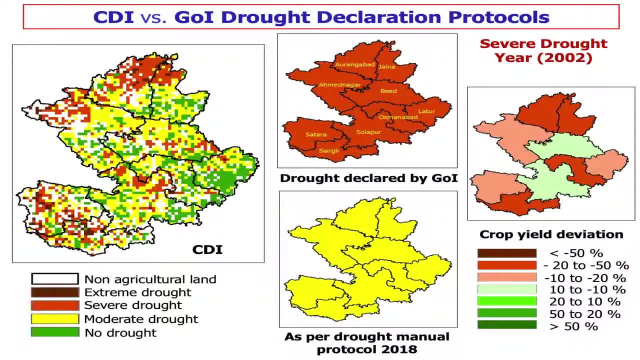 because at that point of time we were not sure whether these declarations were fake or real. So we had to assume this as real. So we pulled out the drought declarations and then we also applied the government of India's recent protocol of drought declaration. 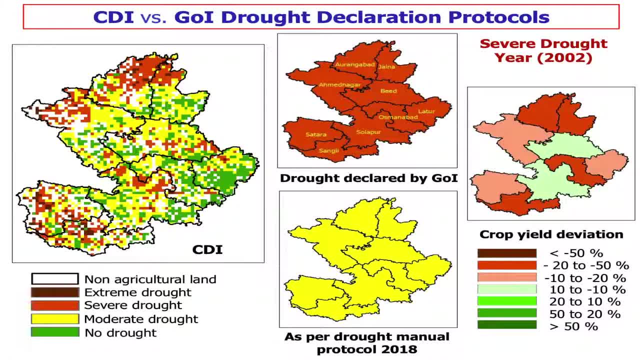 as per the 2018 manual, which is shown in the yellow map below. And then we also compared it with the yield deviations, because those are also government of India declarations. And if you look at all these three, four things and put them together, 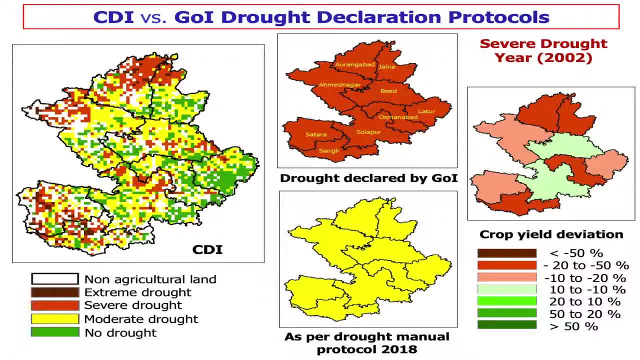 very clearly. you can see that as per the government of India declaration, the drought was widespread. They declared it as a severe drought But as per the CDI, if you see, it was like moderate to severe drought, Mostly moderate, with some pockets. 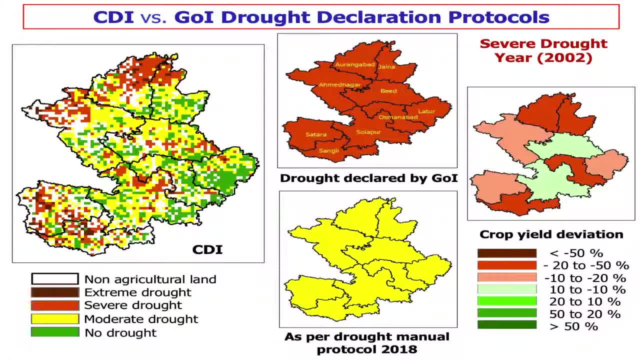 in which the severity was there. So we went ahead and compared it to the government of India protocol for 2018, according to which it was a moderate drought all across the region. But if you compare it with the yield deviations, you find that the yield deviations are quite 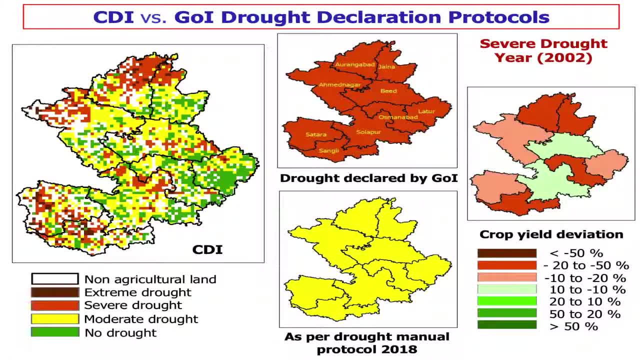 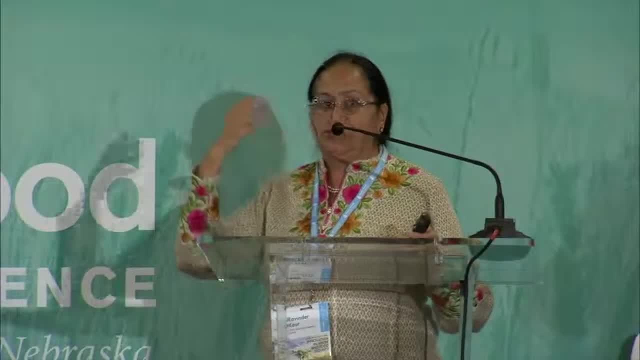 matching with the CDI observations. So not only this approach, through this approach we found that the government of India declarations of the severe drought conditions was kind of a fake, You know, because they wanted to bring more area into drought to get more quantum of funding from. 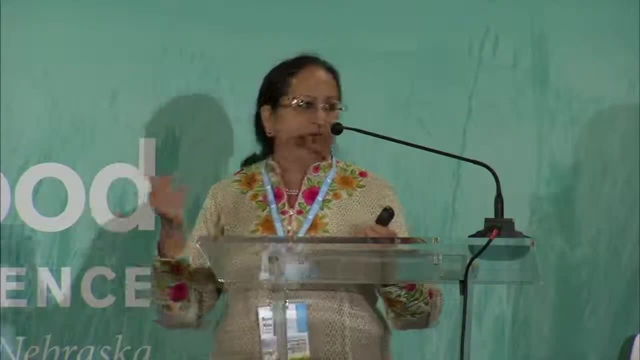 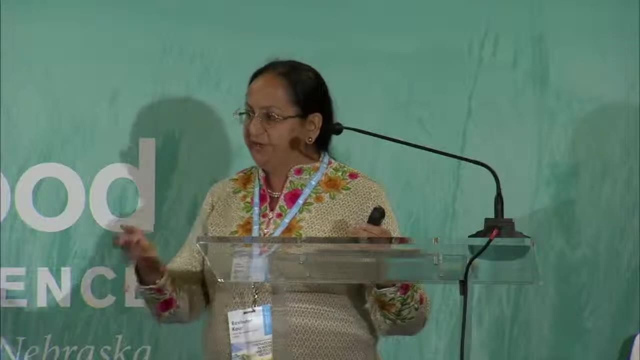 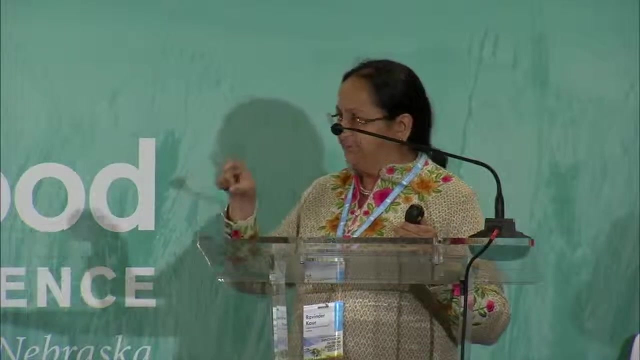 the centre. But the current protocol is also not able to capture the drought conditions. Secondly, the second problem with the current protocol: it is following the lumped approach, So it doesn't precisely tell us that within the district or within the block. 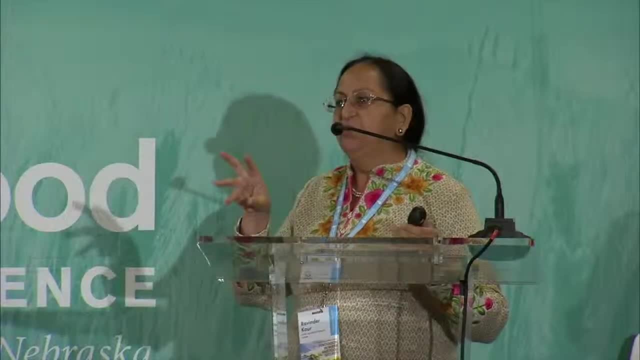 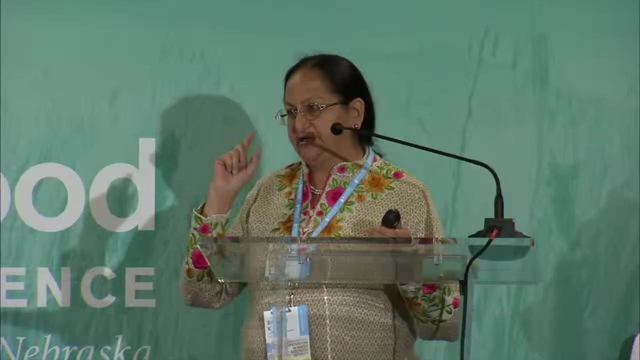 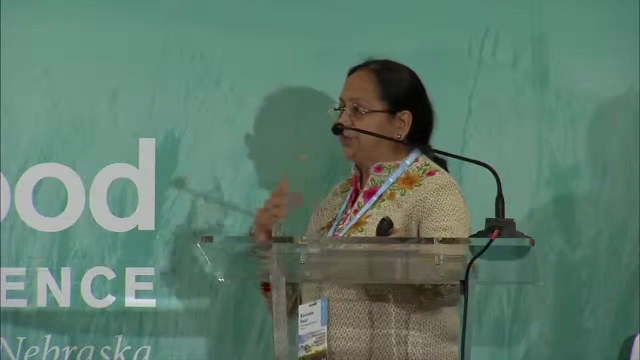 what is the spatial extent and severity of the drought. So it appears as if the whole block is under the severe condition or the whole block is under the moderate drought condition, But actually the same block is under three different categories. So by knowing if a stakeholder 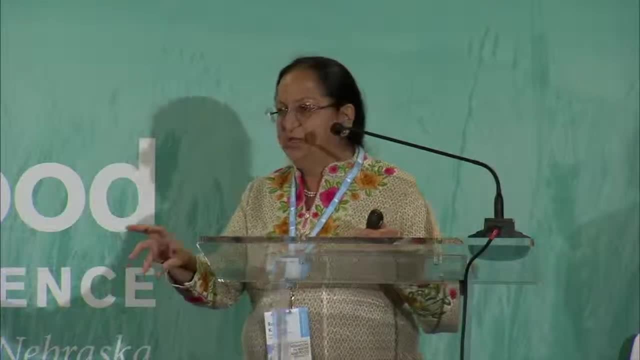 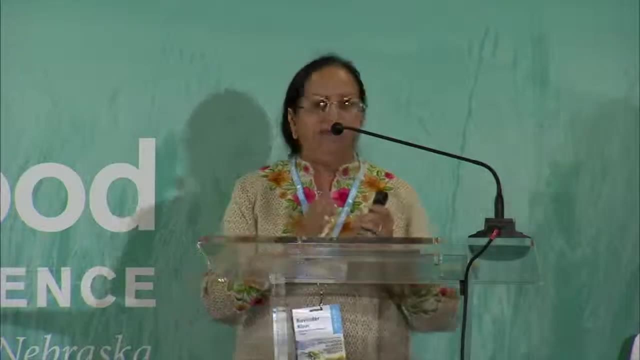 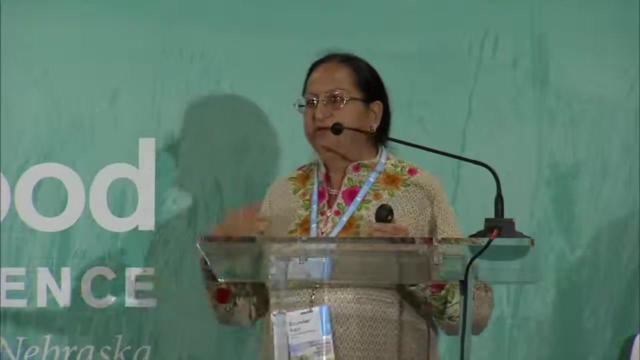 knows that what is the category of drought within the block also, then he can appropriately and proportionately distribute this centre granted funding. So because instead of distributing a hundred rupees into one one rupee to all, then some people can get fifty rupees. 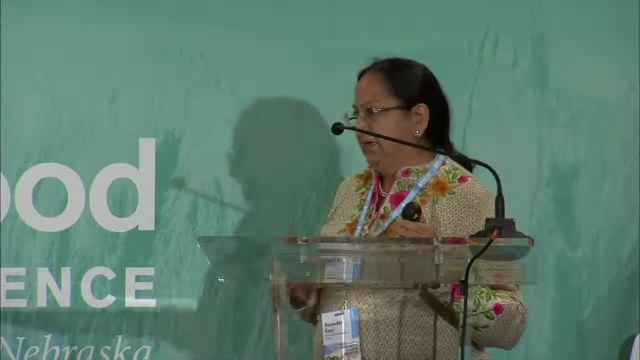 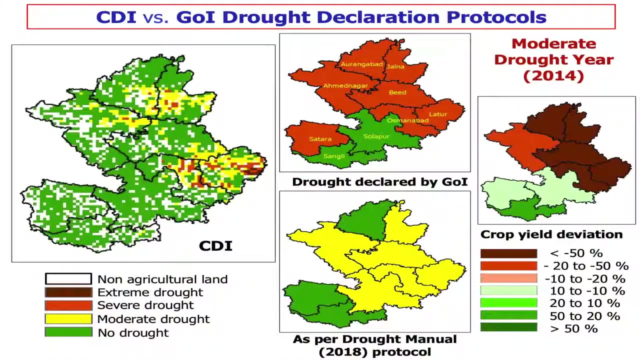 some can get twenty, some can get ten, depending upon their need, And thereby reducing the farming issues on ground. So we also try to apply this tool in one of the moderate drought years And again, as you can see very precisely if you compare. 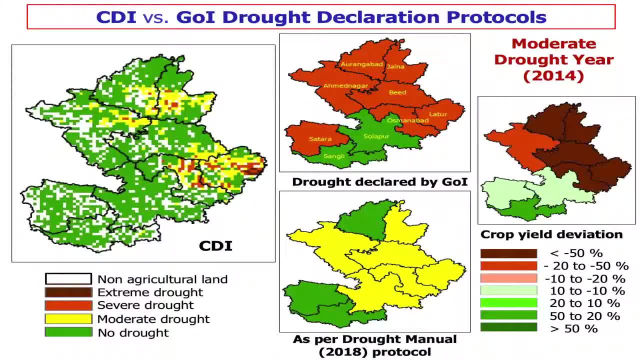 CDI product with the crop yield deviations. they are quite matching, While the drought declaration by the government were not matching their own yield deviation data And also the government of India protocol- recent 2018, was not able to capture the drought very well. 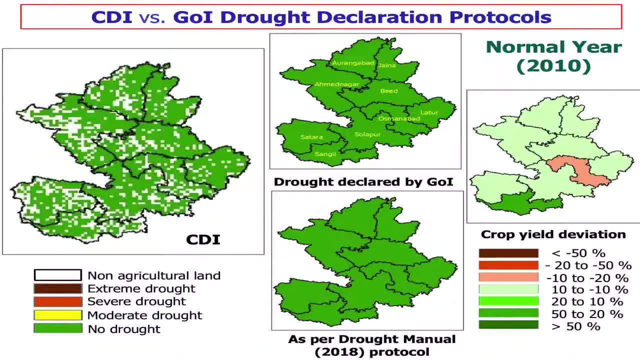 Again, we wanted to see whether this same approach is able to capture the normalcy of the normal condition also or not. Although it is only able to capture the drought conditions, So we see that it was CDI- could very realistically capture the normal. 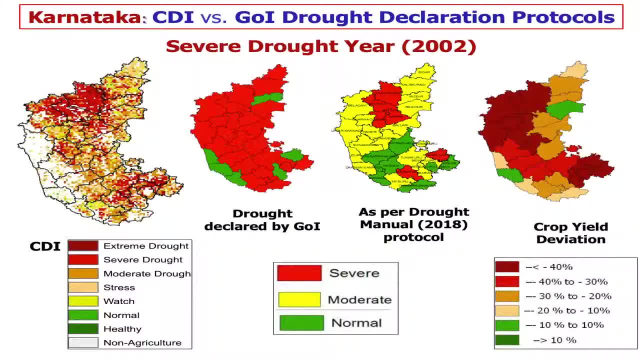 conditions also, And this was on the Marathwada and then next state on which we applied was Karnataka. It is also one of the most drought hit areas in the region And the story is the same and you can yourself see that the 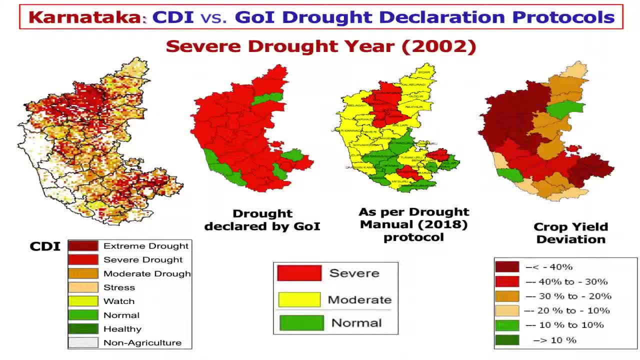 government of India declaration was severe drought for 2002 all across the state. But if you look at the CDI variations and compare them against the crop yield deviations, they are quite, you know, in sync with the crop yield deviations And the government of India. 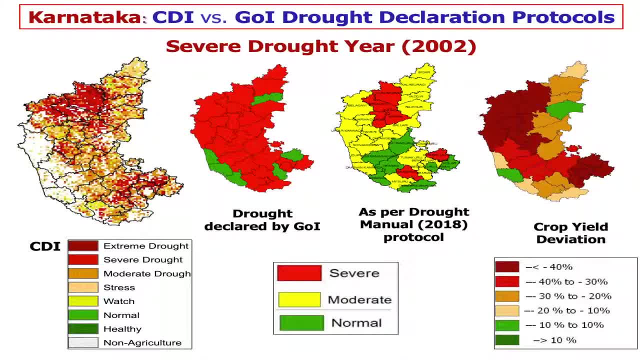 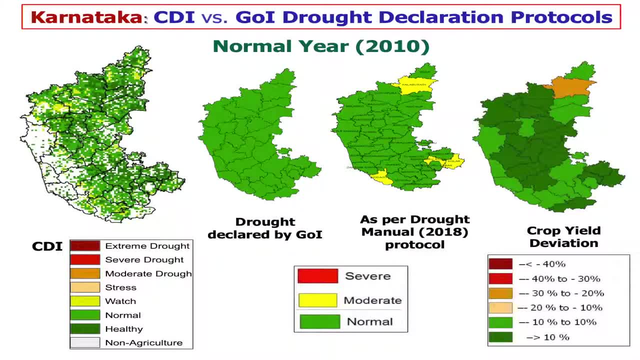 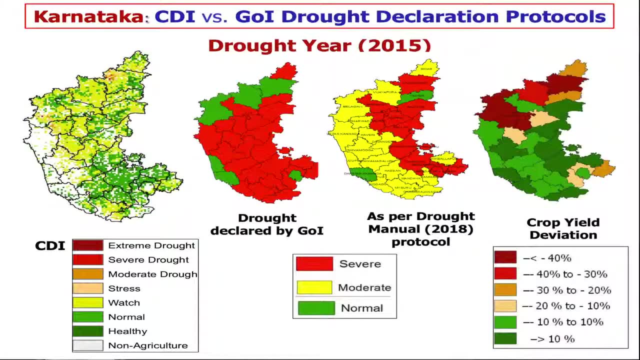 protocol, definitely 2018 protocol also was not able to correctly capture the drought and its spatial extent. Again, same for the normal year 2010.. CDI could perform very well, And again for 2015,, which was kind of a moderate. 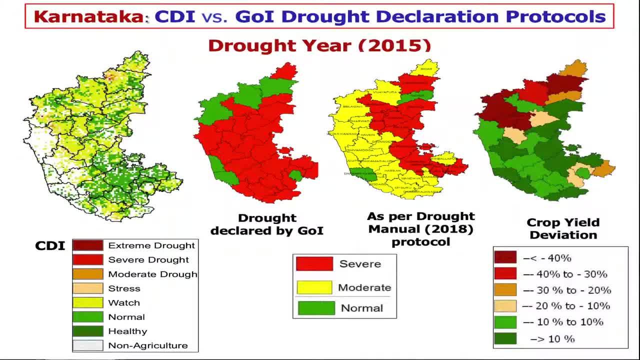 drought for the state And this also could be very nicely captured. And I would like to mention here that the CDI product which I'm showing you here is a five kilometer product. It's a coarse resolution product. We deliberately started with a coarser resolution product to see. 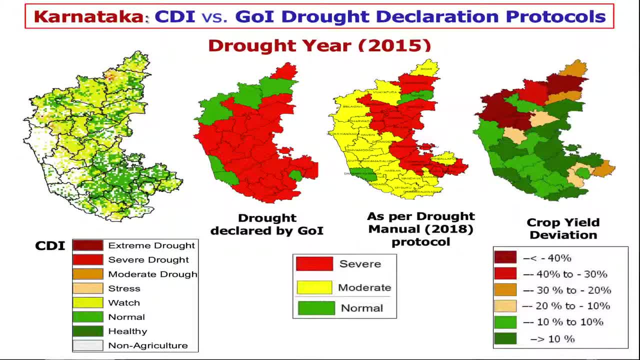 because if a coarser product is able to capture, then definitely the finer product will be able to give the finer details. So we hope now. recently we also tried to compare this with another drought monitoring methodology which is called South Asian Drought Monitoring System. the results are still. 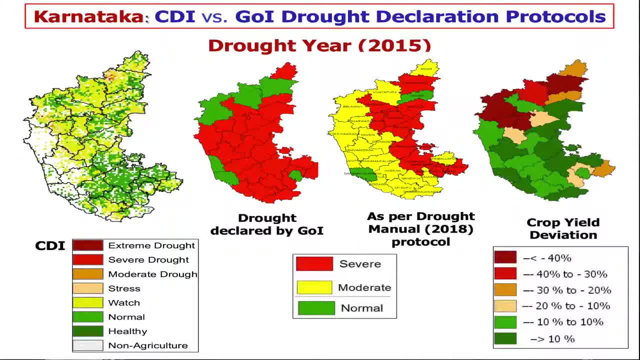 the weighted, And also we are trying to see what is that spatial resolution at which we should be giving the product to this state, Whether it has to be five kilometer or 1 kilometer or 500 meter. So our so far study and 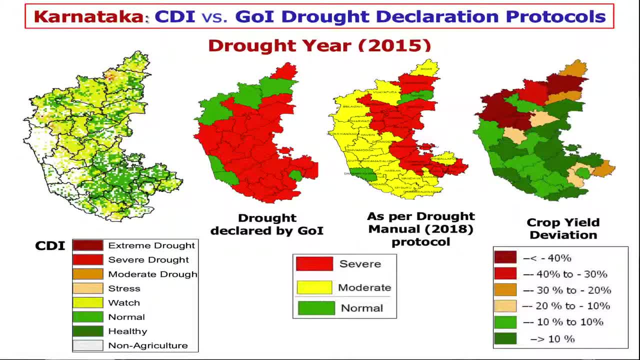 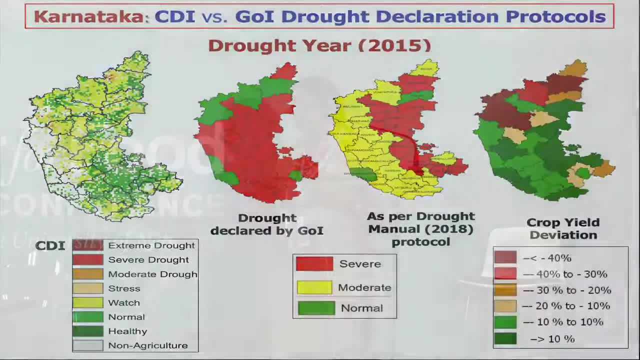 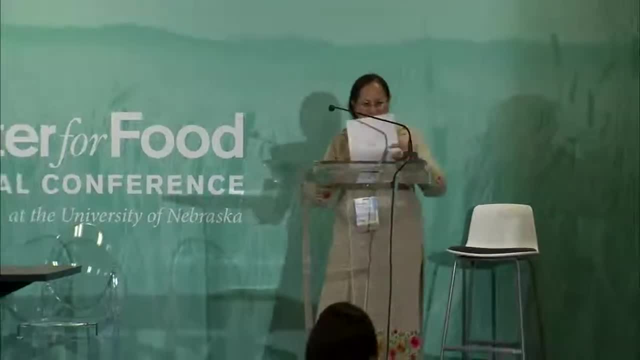 I haven't put the results here. it shows that five kilometer to one kilometer product is good enough to to and to reflect the near real-time drought conditions as far as Indian India is concerned. So with this, thank you very much for your patient hearing. 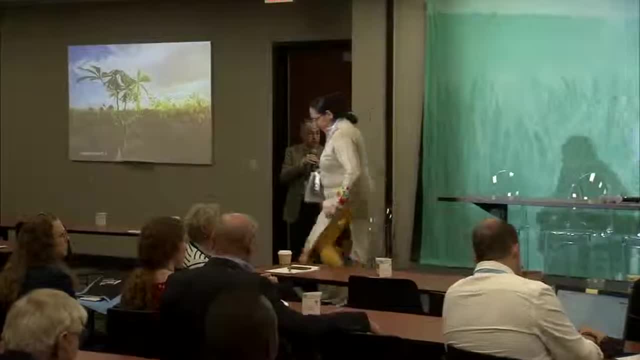 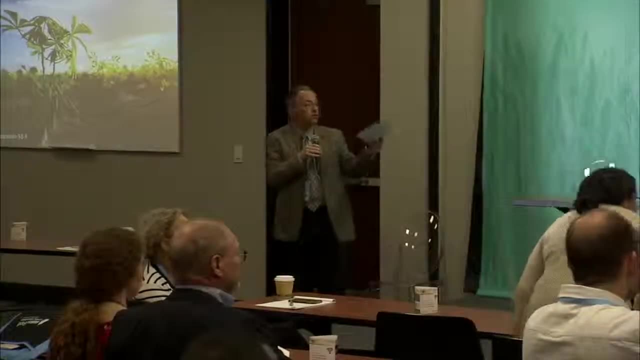 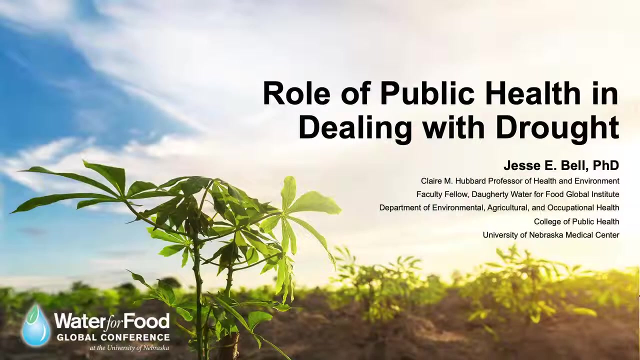 Thank you very much, Dr Carr. So our fifth presenter and last presenter this morning is Dr Jesse Bell, the Claire M Hubbard Professor of Health and Environment at the University of Nebraska Medical Center in Omaha. All right, so I'm gonna speak a little bit broadly and then kind of bring it back into some of the work that 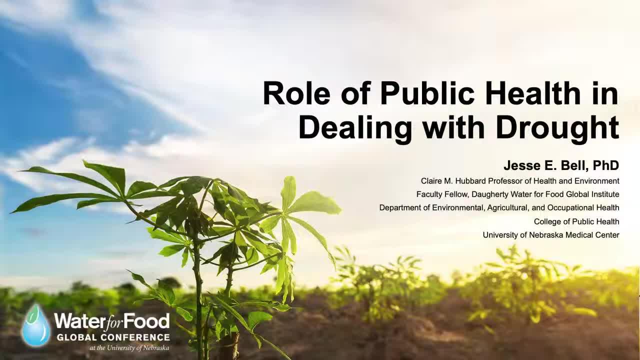 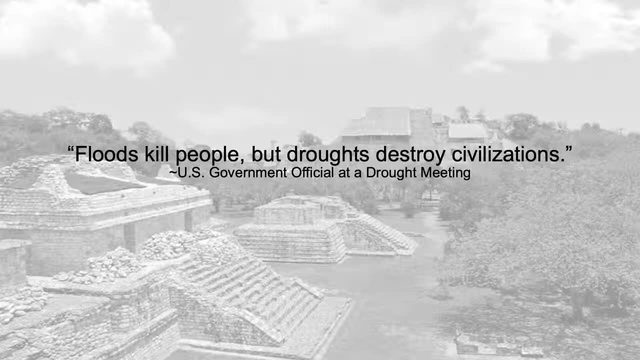 we've been doing. My goal up here is to talk about the impacts of drought on human health and how potentially public health can help with some of the intervention. with some of that, I always start off with this: floods kill people, but droughts destroy civilizations, And one of the things I really want to try. 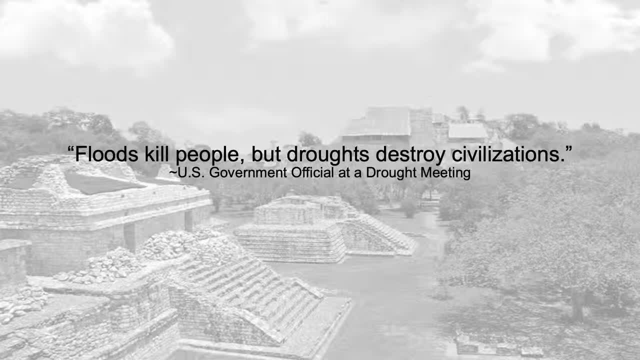 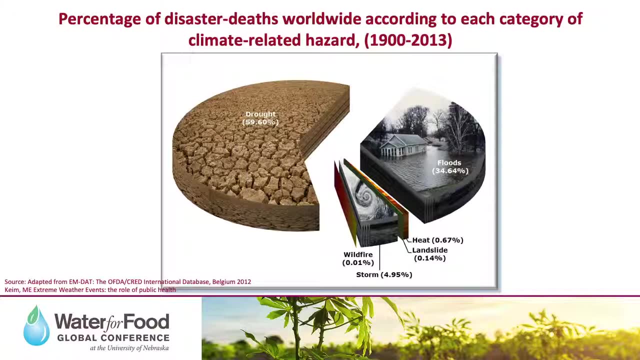 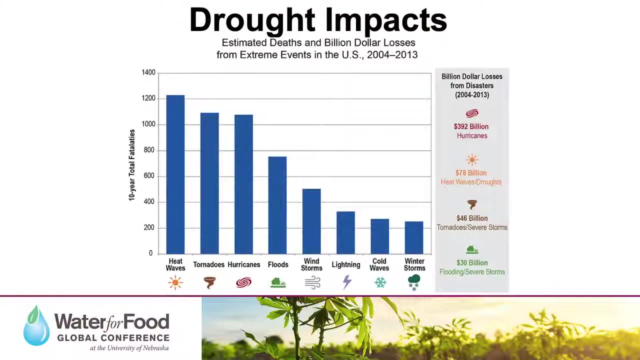 to emphasize here is that not only do droughts destroy civilizations, but they do also kill people, and as they, they move forward as well. So we know that droughts likely have killed more people internationally than any other climate or weather related disaster. and that's internationally, but here in the United States, and that's primarily due 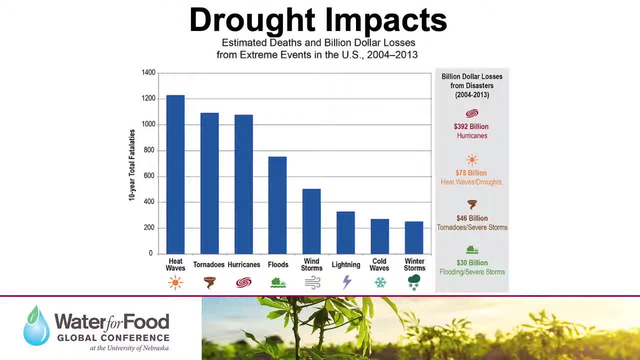 to famine and malnutrition, but here in the United States, we really don't think of drought as a human health threat in any way. So here's NOAA information gathered for different weather-related disasters across the United States, and one of the things that you'll notice is that drought is not one. 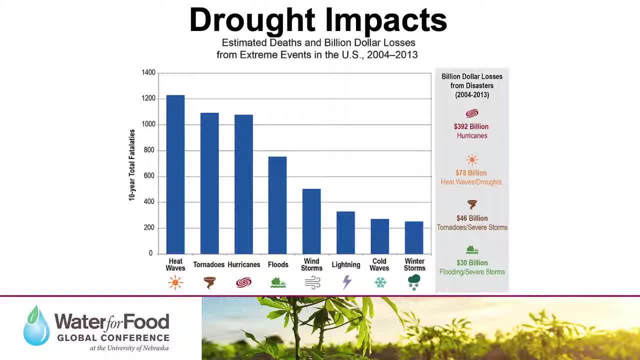 of those up there that's got a death toll associated with it. But we know drought does have severe economic impacts on our communities and our states as well. During that same time span drought and heat waves combined through. this NOAA analysis found that droughts cost about $78 billion of economic loss from 2004 to 2013.. 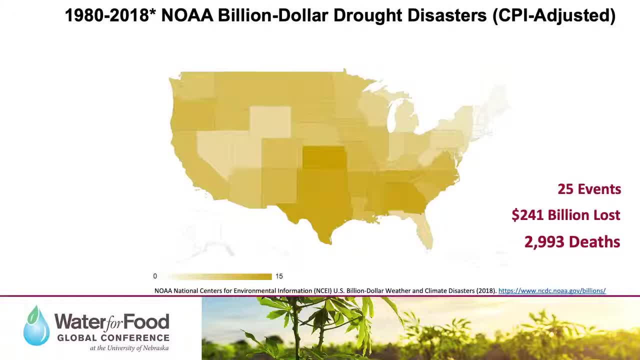 And we know that over the last roughly 30, 40 years that droughts in the United States have – we've had $25 billion disaster events that are associated with droughts here in the United States And those $25 billion disaster events have totaled $241 billion of economic loss here. 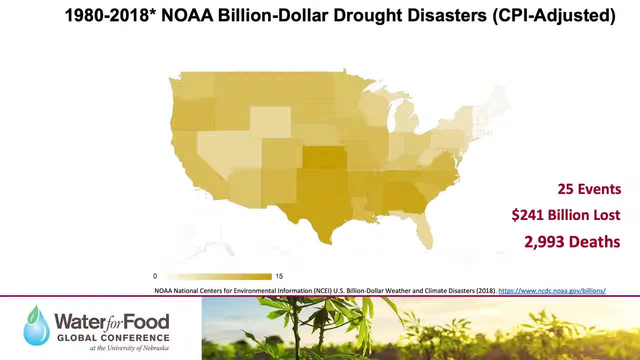 in the US And obviously these have huge impacts across the United States. But one of the things that you'll notice here – and I know I just said that droughts don't have – aren't necessarily associated with human health outcomes, But during those $25 billion disaster events, there was about 3,000 people that were associated. 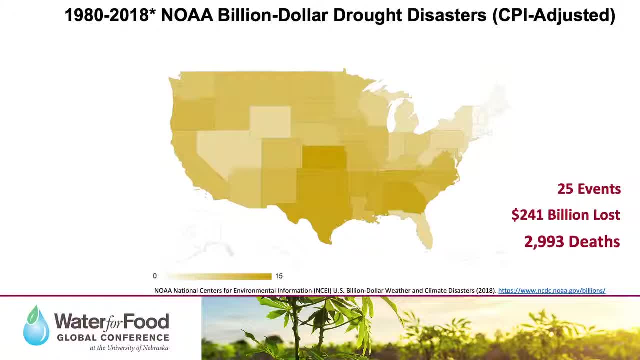 with – or associated deaths associated with those droughts, And those 3,000 deaths are actually tied to heat waves, And so, when a drought happens, typically what – or what can potentially happen is, you see, an exacerbation of a heat wave. 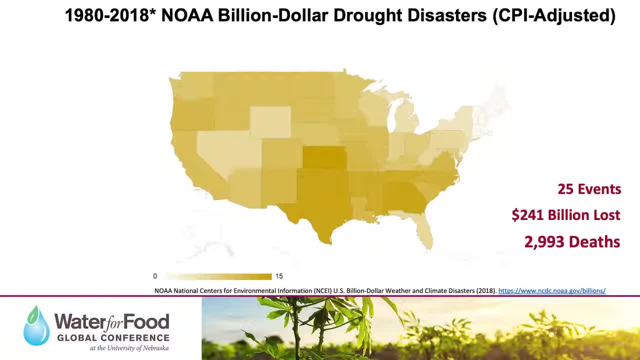 You see a more intense heat wave that happens at the exact same time, And so those 3,000 deaths are associated with the heat waves that were intensified during those drought events. But obviously that's just one component, That's just one sliver. 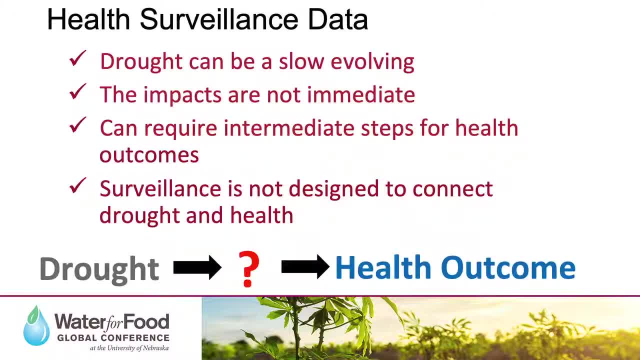 But it's also very difficult. It's very difficult to try to understand all the different health impacts that are associated with droughts. Droughts are a very slow-evolving disaster, unlike many of the other disasters I put up there before. Hurricanes, things like that. they hit and you can see the impacts immediately. 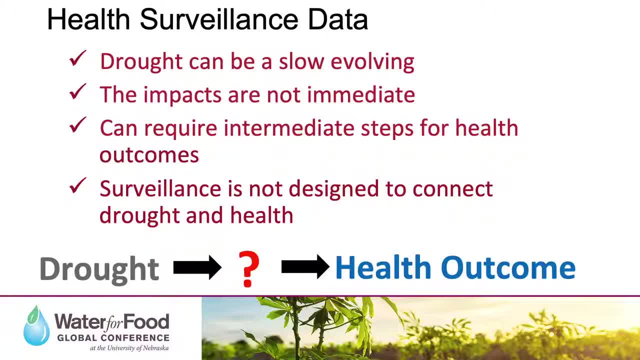 But drought kind of just rolls in slowly and the impacts can be long-lasting and have intermediate potential pathways to get to the human health outcome. And so surveillance data – health surveillance data – it really isn't designed to try and understand the relationship between drought and human health outcomes. 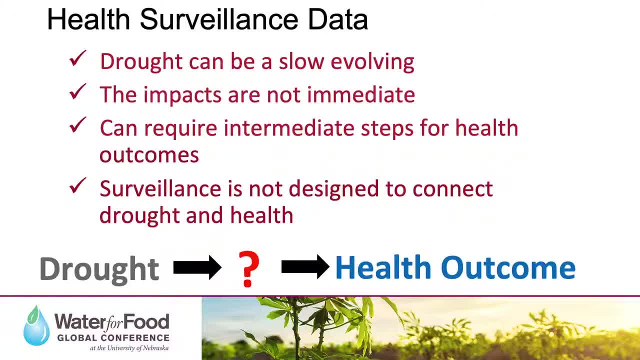 Because there's not an ICD code associated with a hospital visit that says drought, But there's all sorts of other things that are potentially coming on or happening during those drought events, And so one of the things that we're trying to do is try and understand some of those. 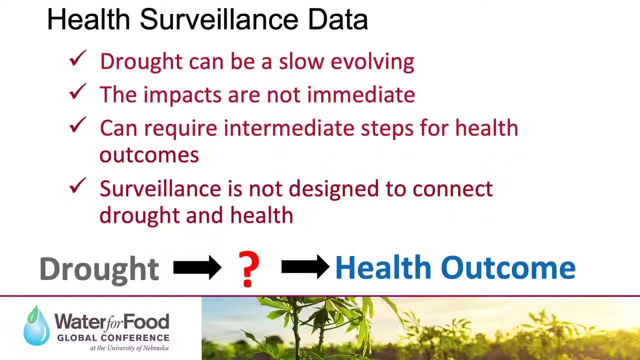 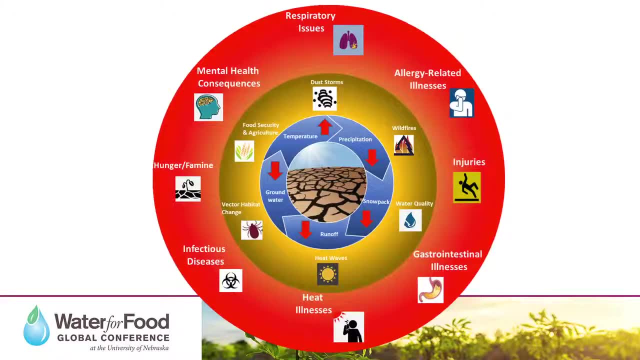 relationships and see why more people are going to the – or if more people are going to the hospital or dying associated with some of these drought events and what that actually means in terms of cost of life. And here I'm just going to try to emphasize some of those potential impacts between drought. 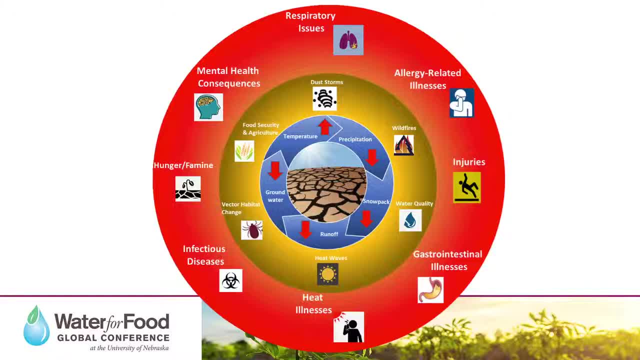 and human health outcomes and some of the pathways that we already understand and we already can kind of identify. So first off, the middle circle, that was the different drivers of potential drought. Then that second circle is changes in their environment or changes in our ecosystems around. 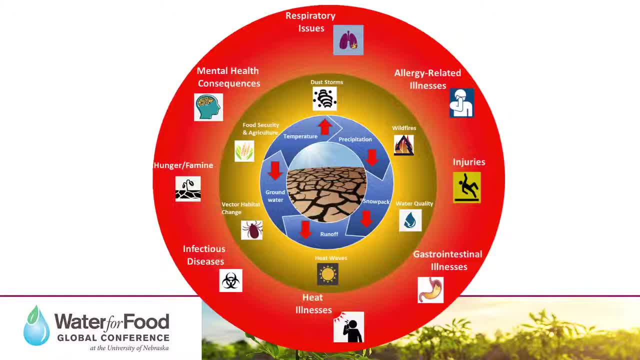 us that could potentially lead to human health outcomes. And then, last, we have the human health outcomes that are associated with those changes in the ecosystems And by the changes in the ecosystems that we see with drought – so one, like I mentioned before: an increase in the intensity and frequency of heat waves, reduction of water quality. 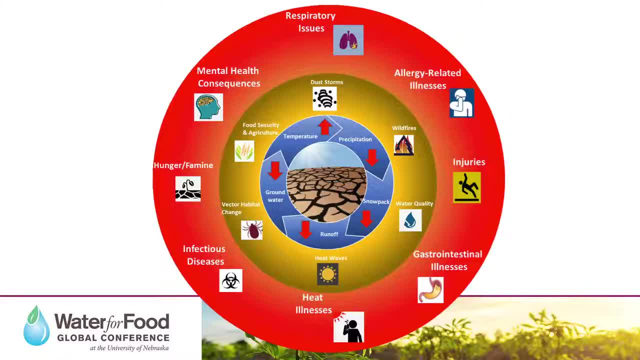 and water availability, changes in vector disease, habitat, food security issues, and then also dust, storms and wildfires that are associated with it as well, And all of those things have potential human health outcomes that are attached to them, And so this is just another way of looking at it. 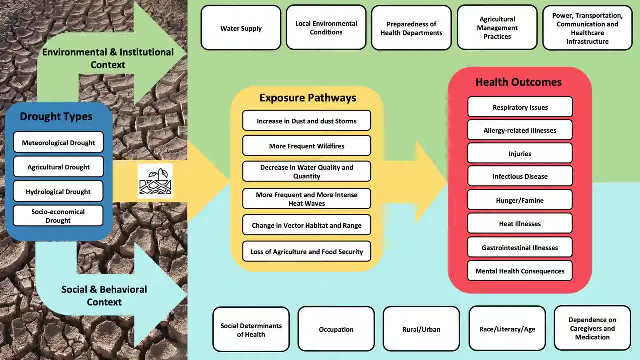 And so this is just another way of looking at it, And so this is just another way of looking at it. So, looking at that relationship, so in the far – I'm looking at the far left side- you have the drought outcomes, or the drought – or sorry, the droughts themselves. 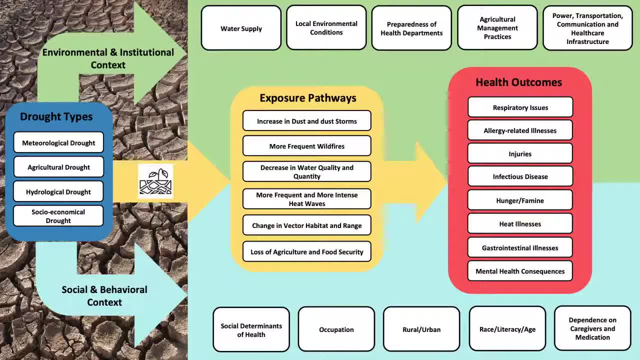 Then you have the pathway in between that gets you from the drought event to the human health outcome, And so that's the general flow of it. So that's looking at those circles that we just previously seen, But one of the things I want you to understand or point out here is the environmental and 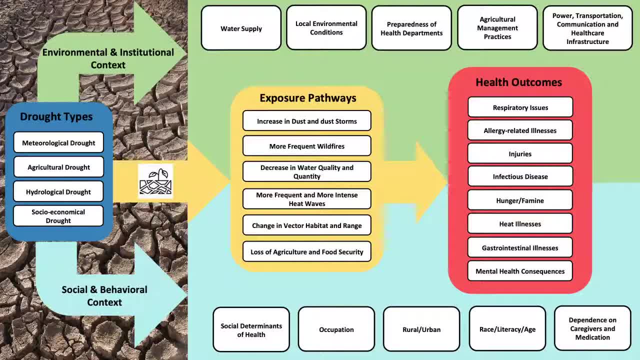 institutional context, and then also the social and behavioral context. These are the things that potentially either increase the number of deaths or hospitalizations associated with drought, or decrease the number of hospitalizations or deaths associated with drought. And so, by environmental or institutional context, we're talking about what is the actual water supply for the communities. 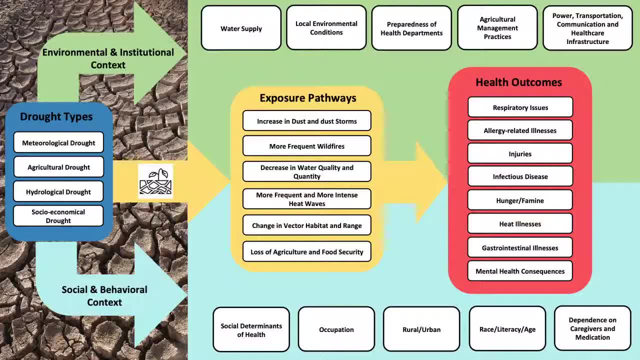 what do those communities look like? what kind of agricultural management systems are in place? what kind of utilities are in place in general, And then by social and behavioral context. that's what we're talking about. What are the people in those communities look like? 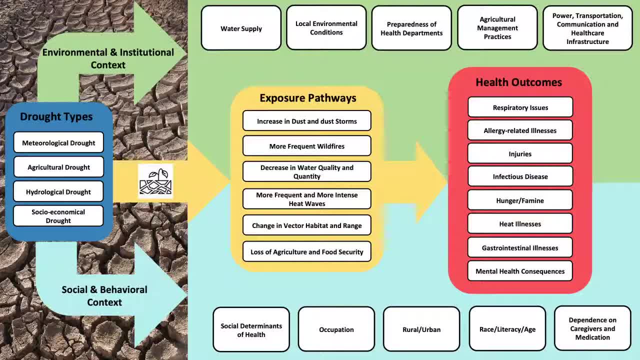 So what's the occupation? Where are they? rural versus urban? What's the race, literacy, ethnicity, What is the access to health care? And is there preparedness plans in place to make people understand the relationships between drought and human health? And so that's kind of getting back to the vulnerability, the vulnerability of the 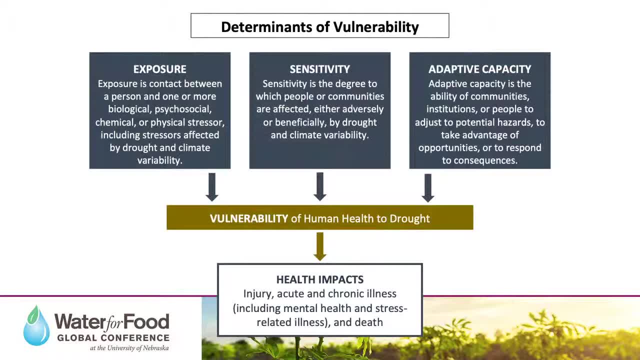 populations, And so, again, that's some of the work that we're doing- is trying to identify some of the vulnerabilities within communities that are associated with drought And by vulnerability. we calculate that using exposure sensitivity and adaptive capacity To understand those three. 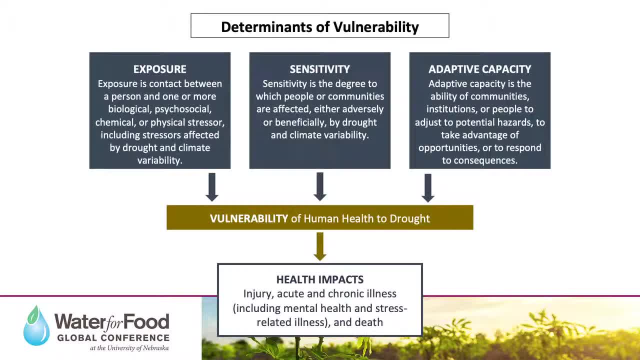 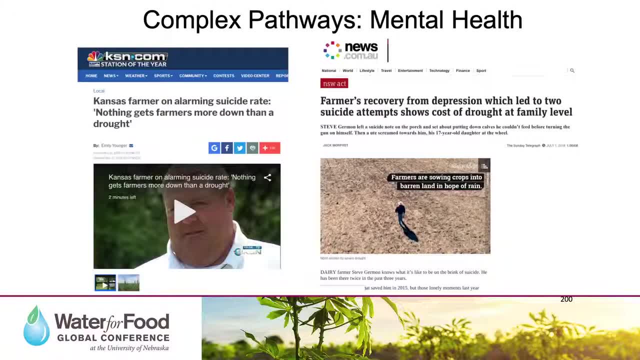 components. that gets at the vulnerability of the community and then that gets at the number of people that could potentially be impacted the next time a drought event occurs. And so, talking about some of that complexity, where we have multiple, we have intermediate steps, We have potential lags between when the drought event occurs and 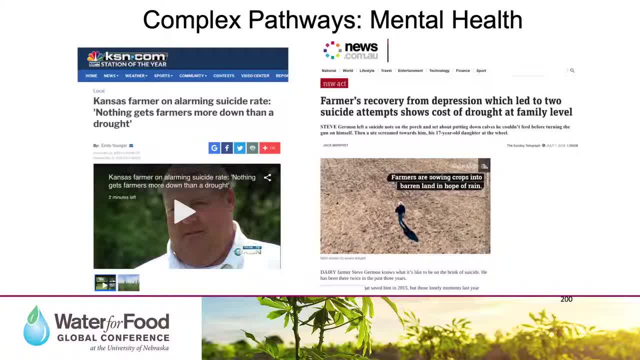 when we see potential human health outcomes. I think mental health is one of the best ways of describing some of that complexity in itself. We know that when drought events do occur, there's potential financial strain that's put on communities, either through agricultural systems. 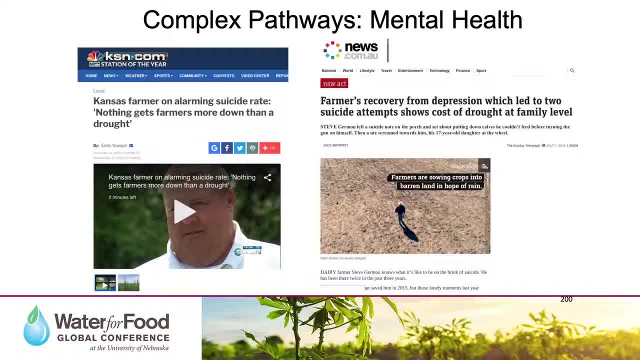 water systems, whatever it may be, And that can have a ripple down effect that could cause mental health and behavioral health issues within that community as well, And so here's some anecdotal evidence associated with that. There's a Kansas farmer that was talking about how there's an 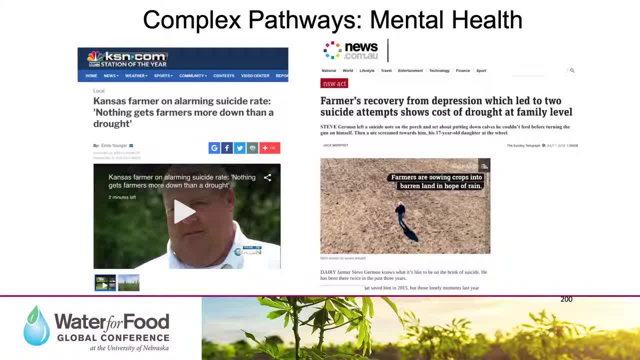 alarming. they were talking about how there's alarming suicide rates in agricultural workers across the United States. They have one of the highest suicide rates of all occupations in the US, And this farmer said that nothing gets a farmer down more than drought. And then over here we have an example in Australia where they showed that during 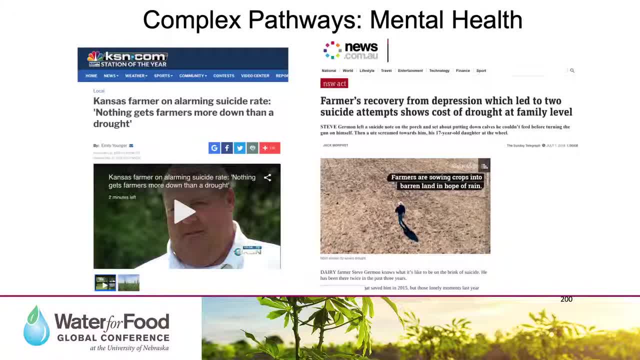 major drought events in Australia. they saw an increase in suicides in rural communities and agricultural communities across the country, And there's a number of other examples across the United States, and across international work as well, that have shown droughts and the associated impacts on mental health. Actually, some of the earliest work that I found was here in Nebraska. 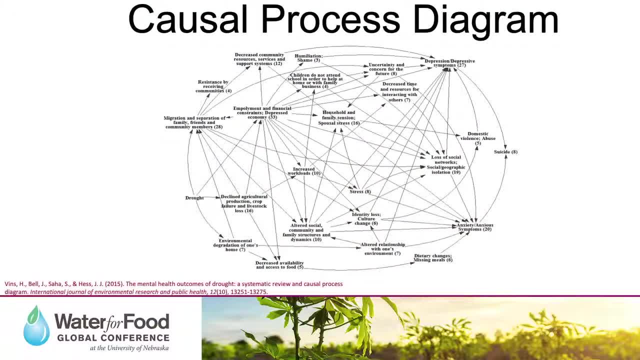 back in the 1980s with a major drought that occurred, And so this is just to illustrate the complexity of that pathway from a drought event to mental health outcomes- anxiety, depression and suicide, And this is work that I did with my colleagues. 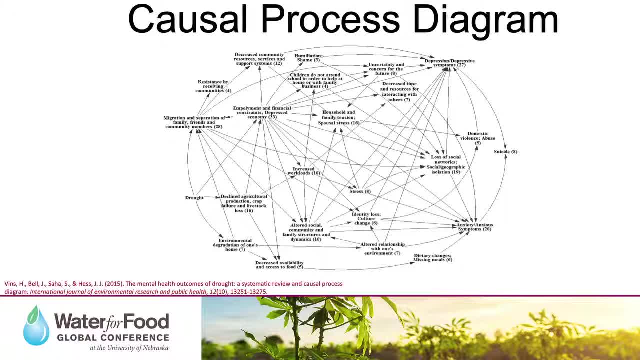 over at CDC in Emory a couple years ago. And so on the far left side of the screen we have the drought event And then what you see is the pathways getting over to the potential mental health outcomes of suicide, anxiety and depression over on the far right side And that 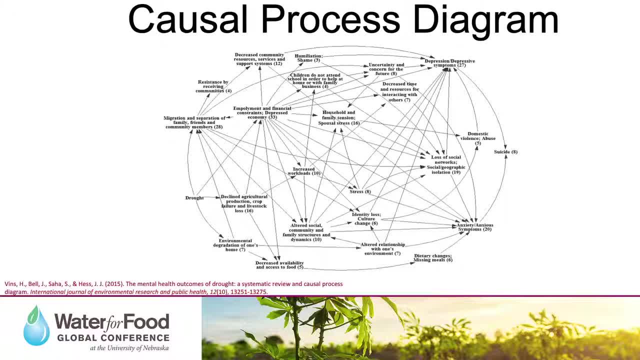 just illustrates the complexity of some of these issues and how, when you're trying to do public health interventions, you need to understand some of this complexity so that you can come in and do mitigation and come in and be able to provide assistance with some of these linkages that are potentially causing human 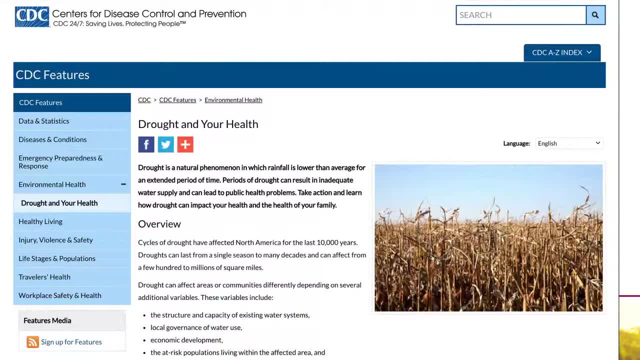 health outcomes, And so, before my previous role or my role now at the UNMC, I was working in a joint role between the Centers for Disease Control and Prevention and NOAA, the National Oceanic and Atmospheric Administration, And so I worked as a liaison between those two institutions, And one of the things that I was focused in on there was not 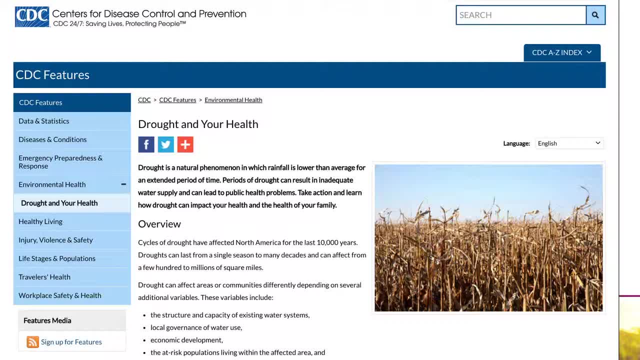 only I was focused primarily on climate impacts, but then all of a lot of my work was actually focused on the drought impacts themselves, And so we had internal funding to try and understand what are some of these potential drought impacts on health, And not only that. try to build up our 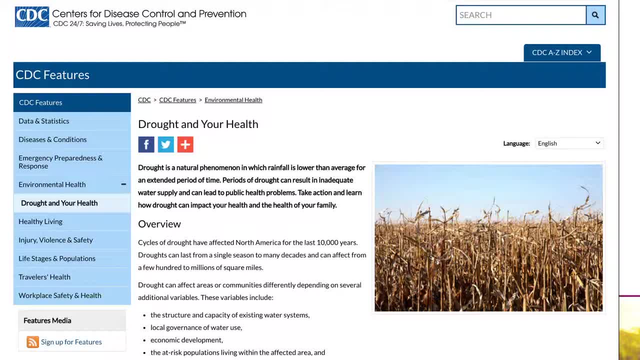 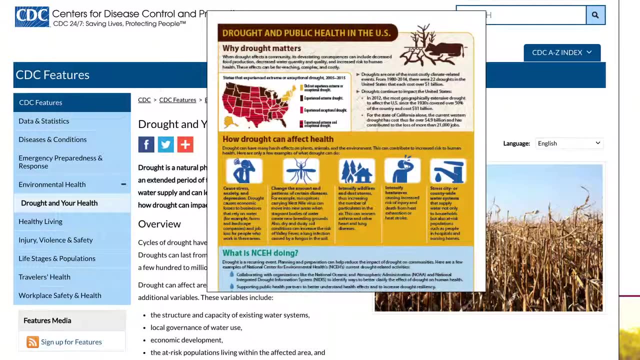 education information to public health officials so that they could help understand the potential impacts as well. So the things that we did was improve the communication efforts so that public health officials can understand the potential impacts of drought on health by improving some of the communication that we had on our website, providing fact sheets to public health officials so that they could understand. 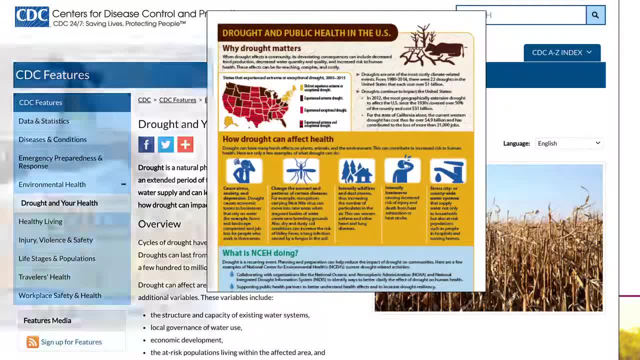 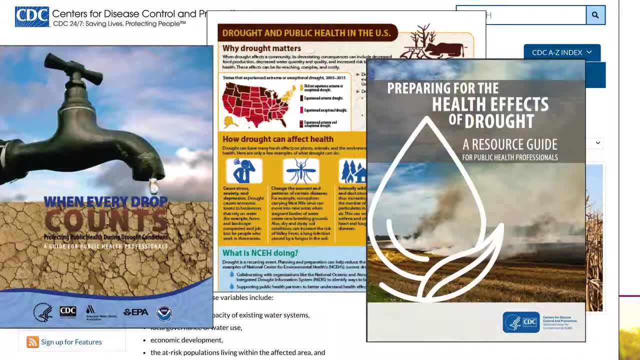 the potential impacts from drought to human health. And then the guidance document – this one was actually made before I was at CDC, but we did a followup document where we did the preparing for the health effects of drought. Dr HP, Dr. 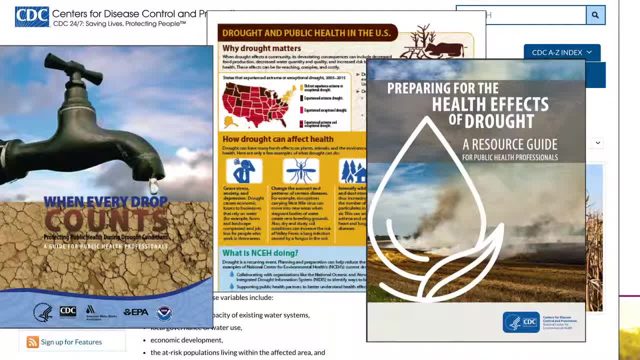 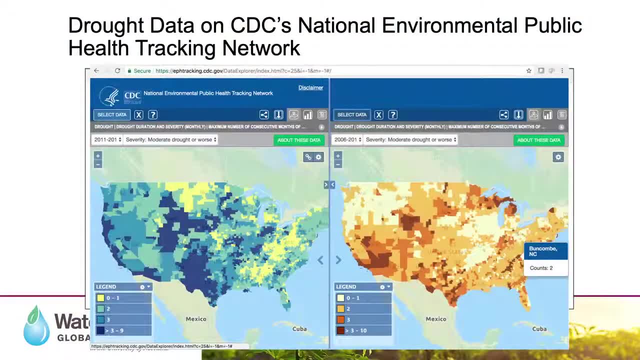 H guide to public health officials so that they could understand the potential health impacts and how to actually do mitigation at the state and local level. And the other thing that we did was we provided drought data on the CDC environmental tracking platform, And so this provided data in an easy, accessible fashion. 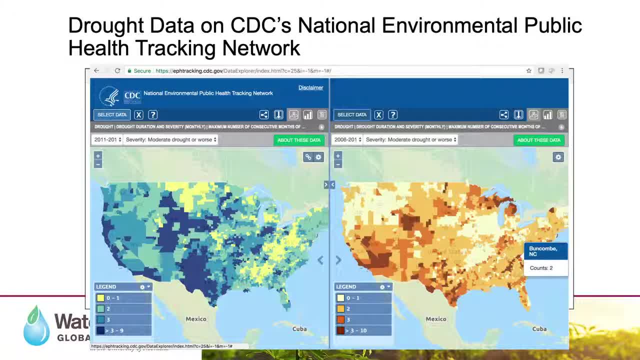 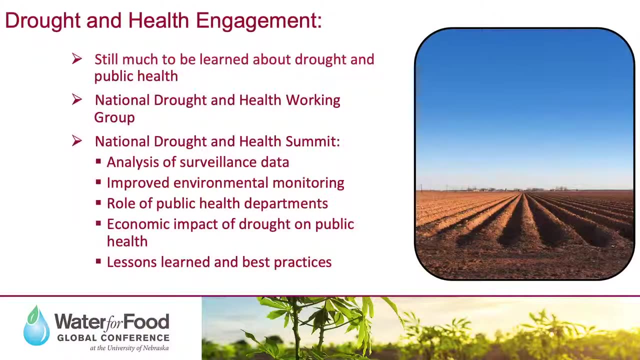 to public health officials so that they could understand the relationships of drought on human health And they could access this data and access this information and use it to do their own studies at their regional level. And so, with that, there's still a lot of work to be done on trying to understand the impacts of drought. 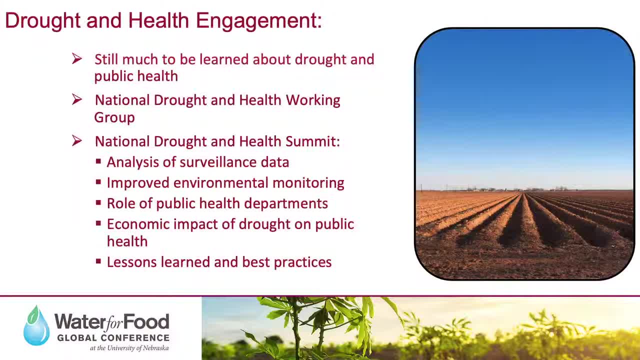 on health. That's some of the work that I'm doing with my post-doc and some of my research and my PhD students. It's trying to mine through the data and try to figure out what are some of those relationships, But also we're trying to do this and address this. 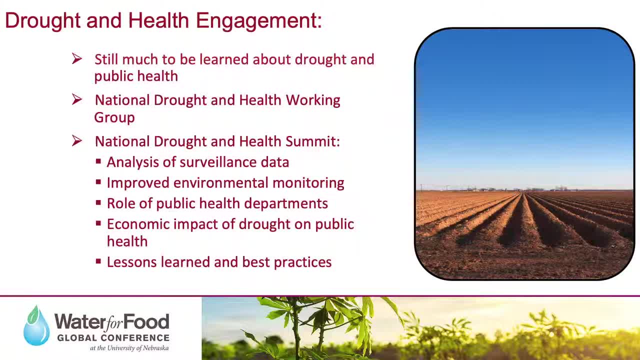 at a national level as well, And so I'm helping work and lead some of the efforts on drought and health with my CDC, NOAA and NDIS colleagues. We formed a national working group on drought and public health. We are also having a summit this summer. 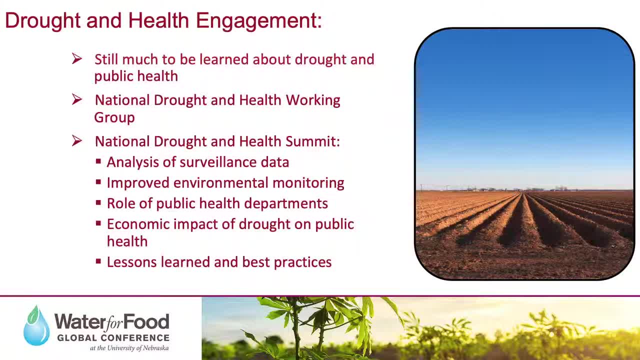 to understand the potential impacts of drought on health and try to understand what are the gaps and needs and what are some of the opportunities moving forward so we can have better information provided down to the state and local sector. And so, with that, thank you very much for your time. 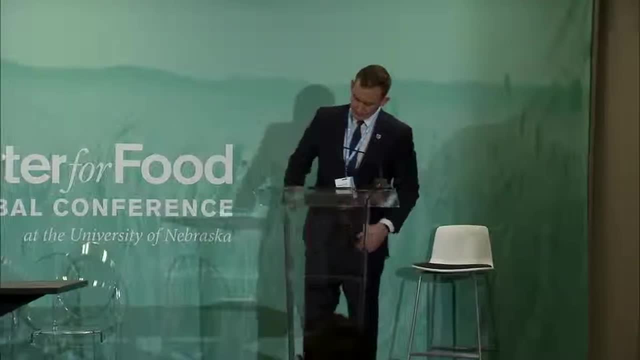 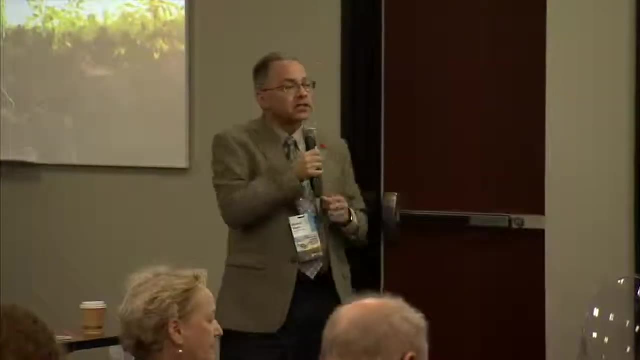 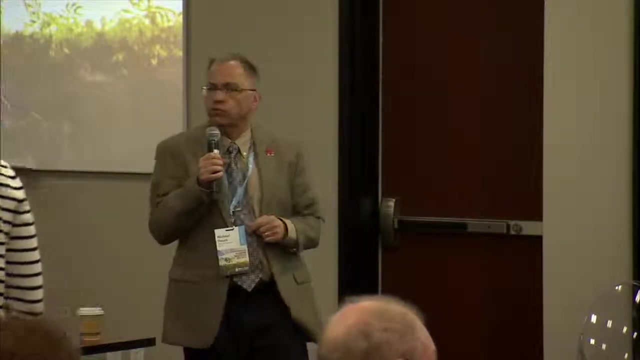 I greatly appreciate it. Excellent, Thank you, Dr Bell. yeah, if I could ask the speakers to come up to the front, And we have about 20 minutes or so for questions for the panelists. What I'd like to do is start first. 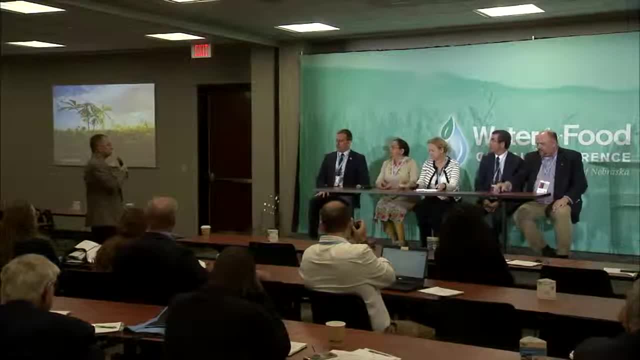 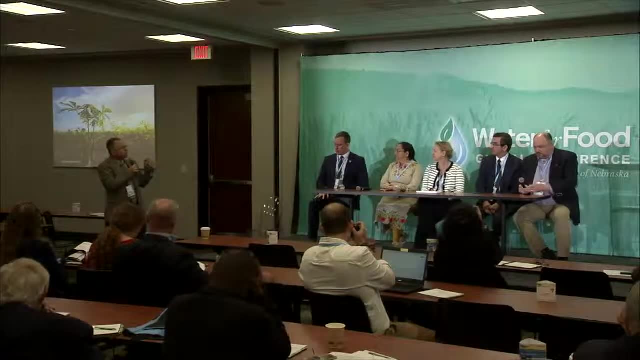 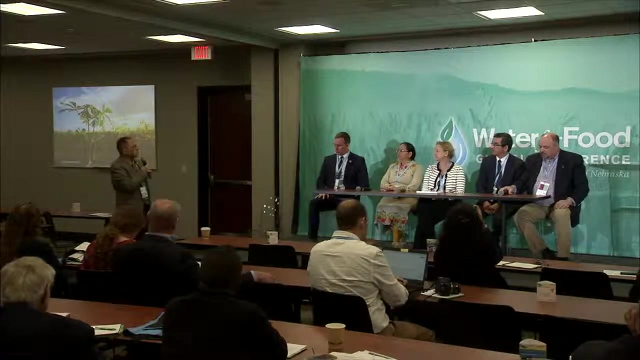 with kind of a basic question And then we'll open it up to the audience. But I'd like each of the panelists to think quickly about what's one big obstacle that you see that stands in the way to your now. what next step? 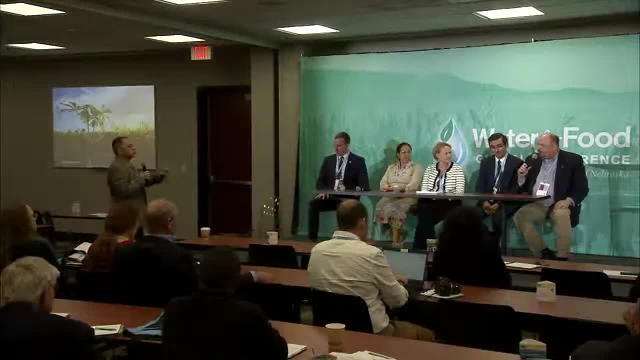 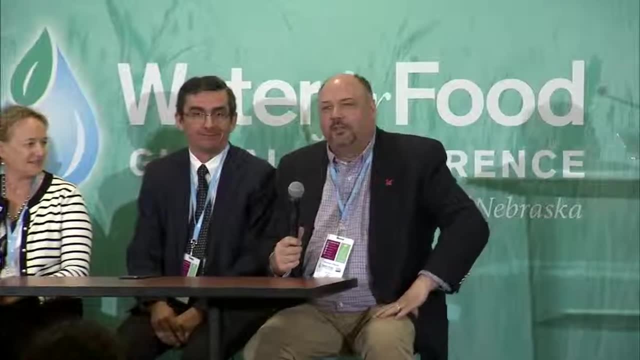 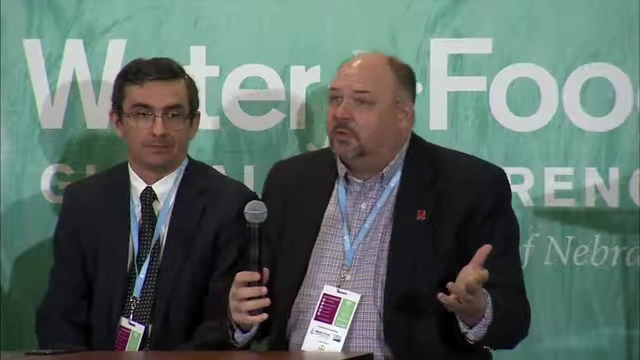 So, Mark, maybe you want to start with that And we'll move So literally. another graphic that put us on the map that Dr Rohit worked on when he first started the center was called the hydro-illogical cycle and empathy. You don't react to any hazard typically. 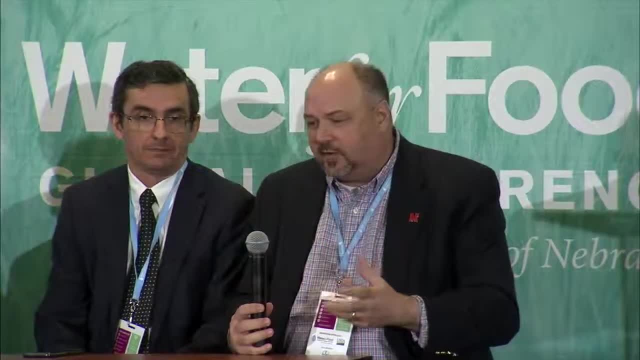 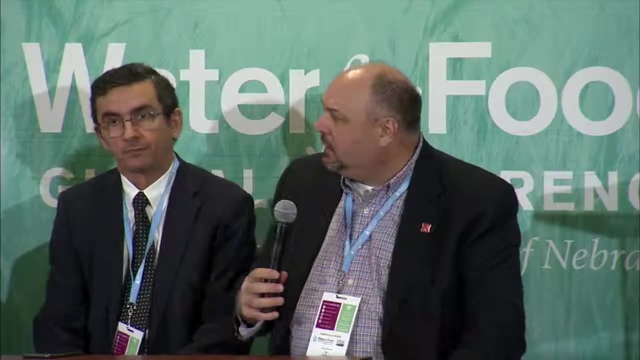 until you're in it, right, And the worst time to manage a disaster is when you're in it. So that's why we're preaching the proactive risk management approach. It's a reactive response, crisis mode response. That's my two cents. 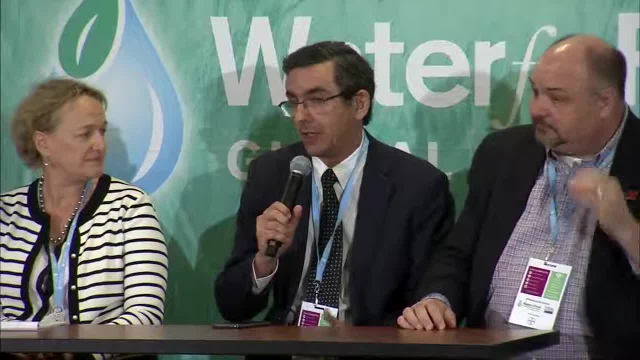 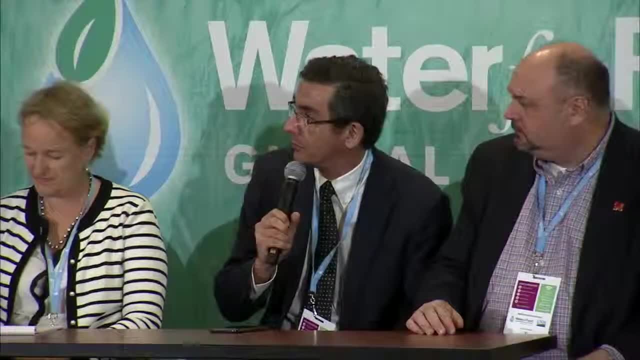 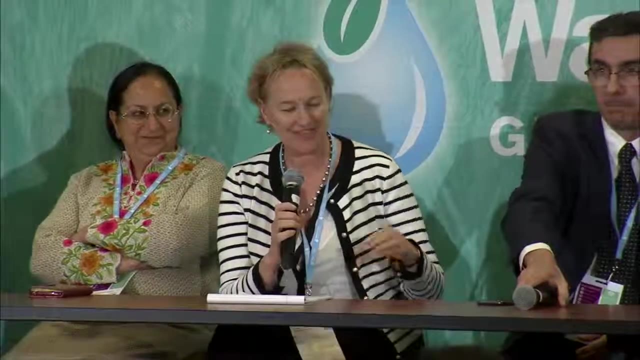 Well, in case of Brazil, I would say that it's the challenge to work in a collaborative way, share information. This has been a challenge in the monitor process, Working across political boundaries, All the ministries we work in. they have their policies. 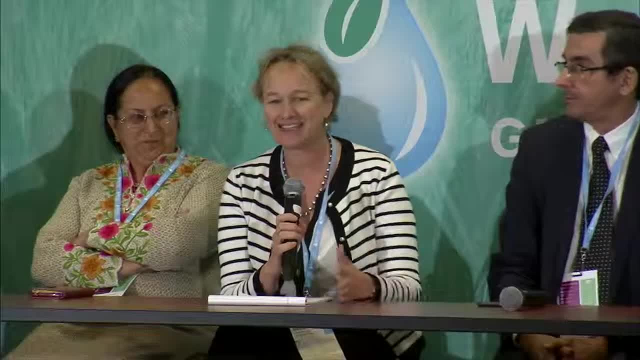 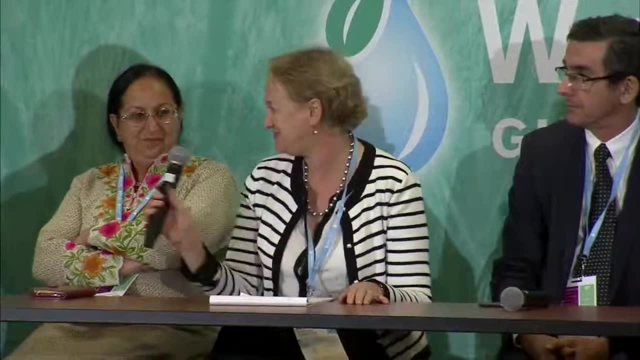 They have what they're expected to deliver onto a government And they're often against it. So I think that's the challenge, And then when a drought comes along, that's very challenging. I think, if I look at the Indian ecosystem, it's the data availability. 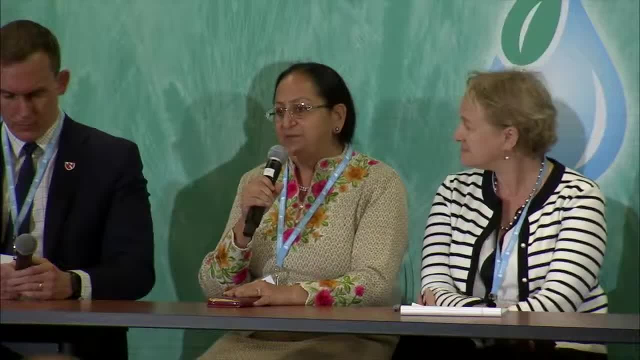 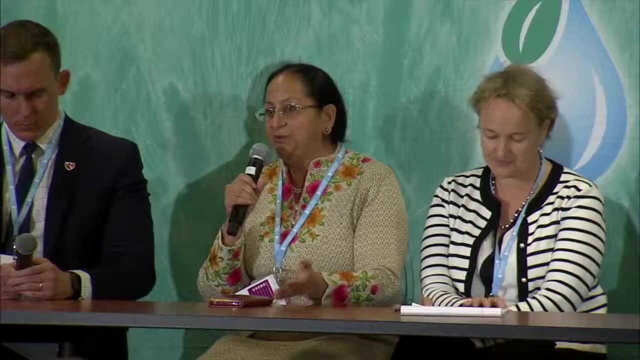 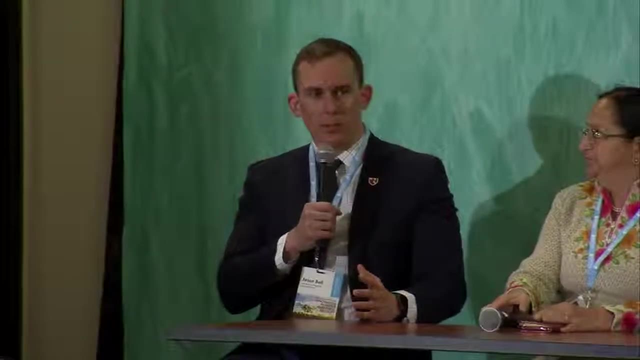 I think that's the major challenge And the reality of that data, whatever is available, if data is available, how real it is. So that, I think, is the challenge And for me I would say that it's awareness. 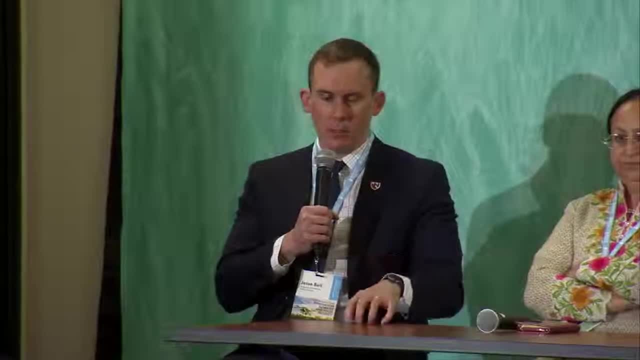 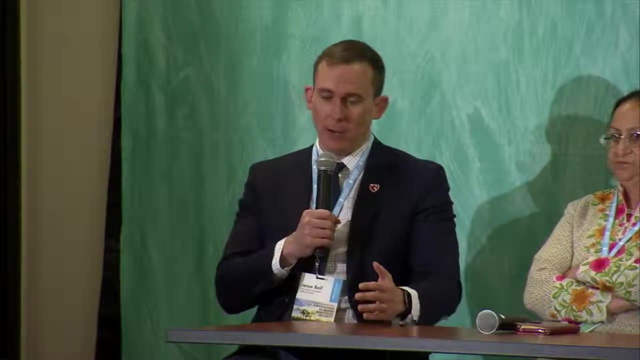 In the public health sector. we really don't think of drought as a human health threat, especially here in the United States, And so it's trying to bridge that gap and have the people that are working out on the ground understand the potential health impacts. 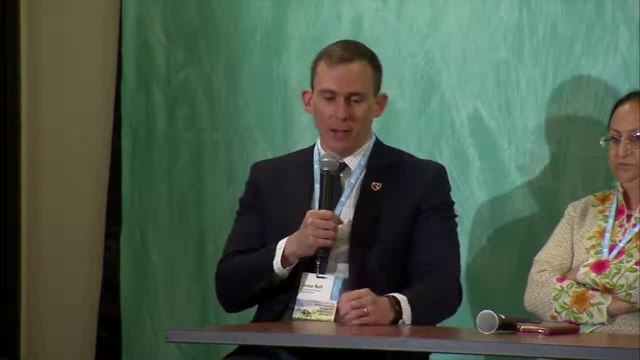 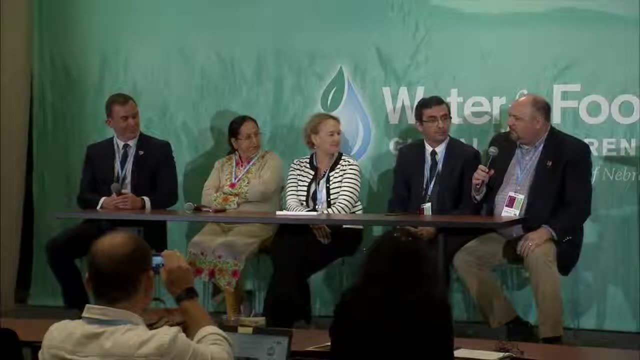 Because I think a lot of them don't even see or know that they're in drought when it's occurring around them. So I think that's probably the biggest thing. I just wanted to say that Mike didn't tell us what the questions would be, so I'm just really proud. 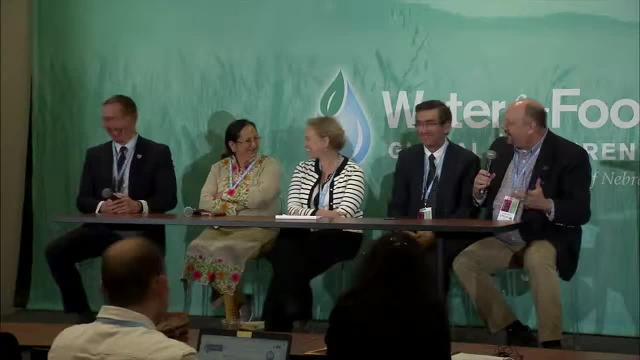 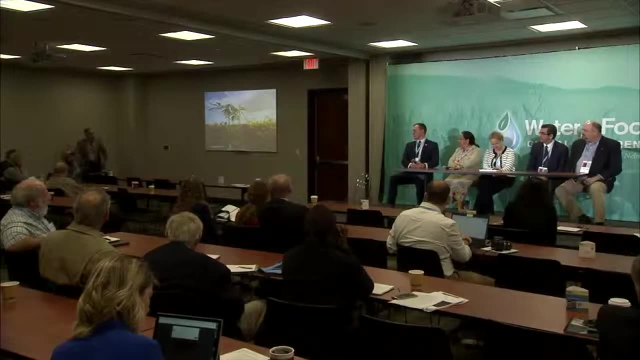 of this panel to give five different answers on the fly like that. That's awesome. So I think some of you emphasized it more than others, but all of you have indicated how important data is to making good decisions and preventing the worst outcomes when it comes to drought. 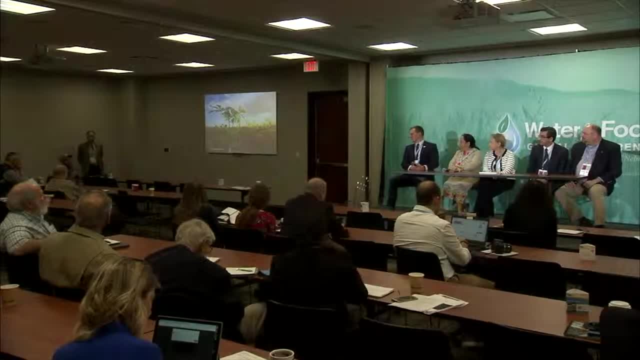 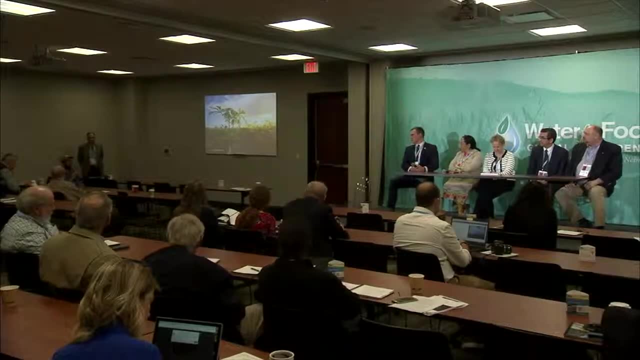 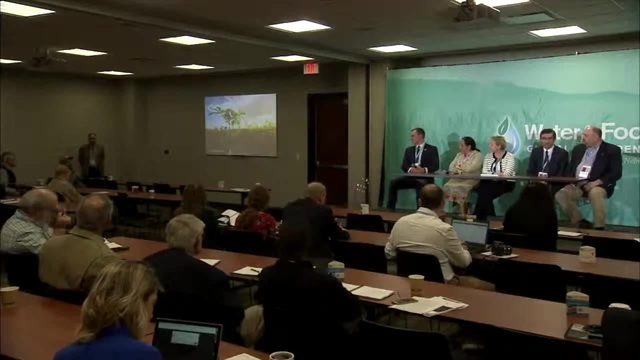 This is for anybody or all of you, but is there any sort of innovative ideas that involve people submitting data to a common platform to be used in an integrated system for prediction? That any ideas that you've had or developments that you've seen that we should look out for and think? 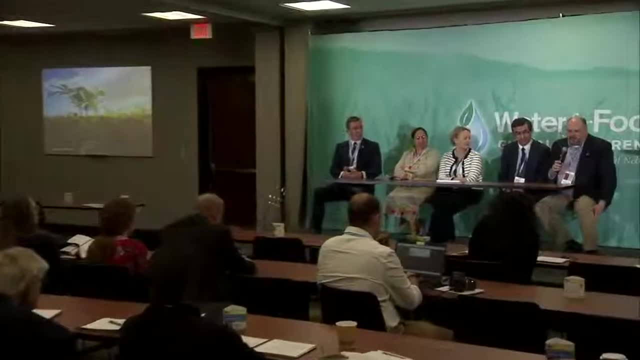 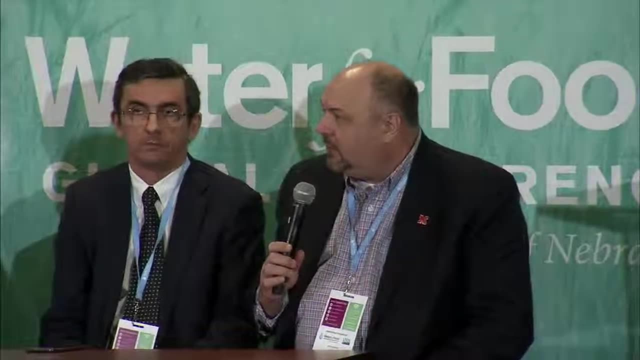 about contributing to. Let me jump in first on that quickly. I didn't cover it in my talk. Again, we only had 10 minutes, So we established what we call a drought impact reporter and a database back in 2005.. We've collected maybe around 80,000 reports to date. 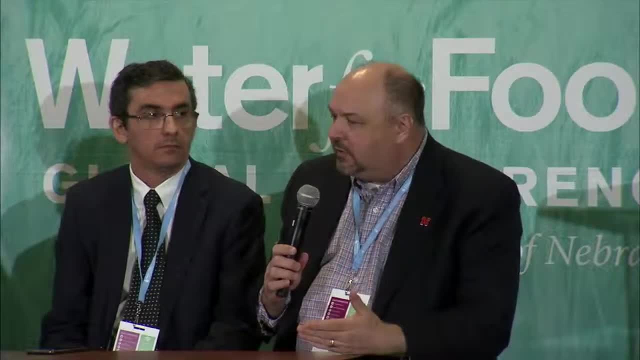 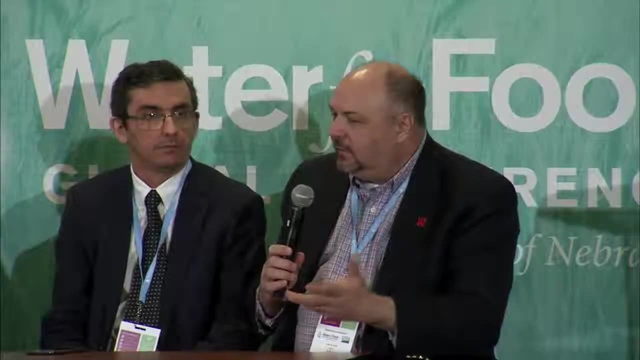 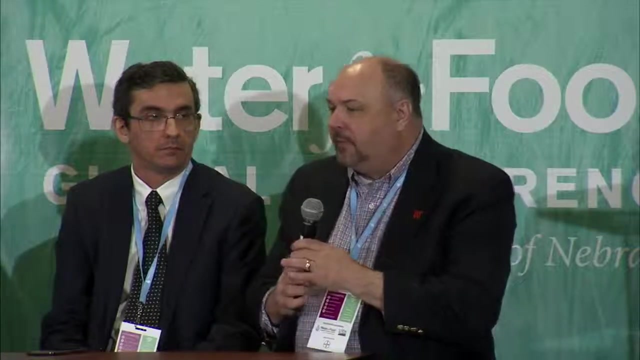 But how that's evolved. I will say that was primarily media driven. in the past We were collecting based on skimming or electronic news media through a service and through typical Google searches. But the assistant director of the Drought Mitigation Center, Kelly Smith, she's working more recently. 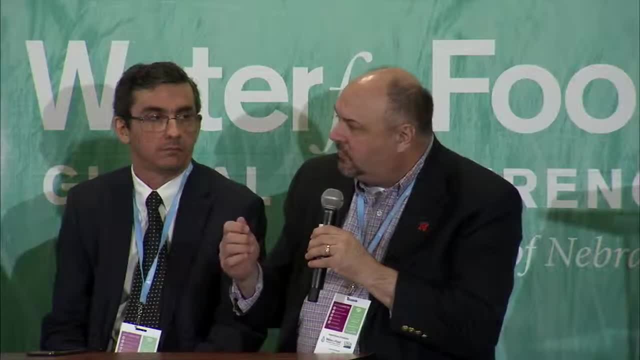 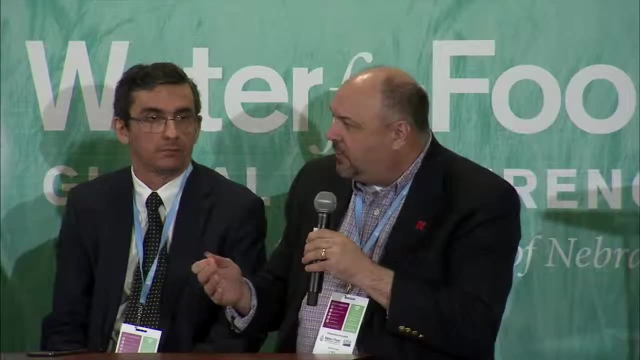 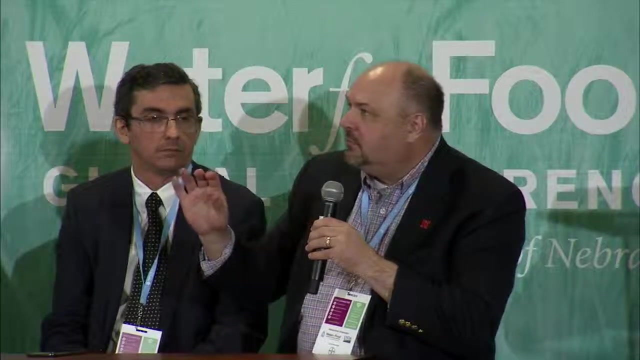 and we are as a center on, like Survey123 and other methods of collecting information in real time, sort of citizen science of condition monitoring. just tell us what's happening, We'll kind of figure out if that's drought or not And doing like hashtag, drought 17 in the Dakotas. 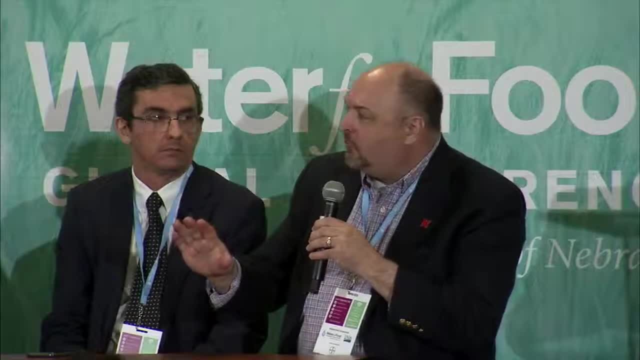 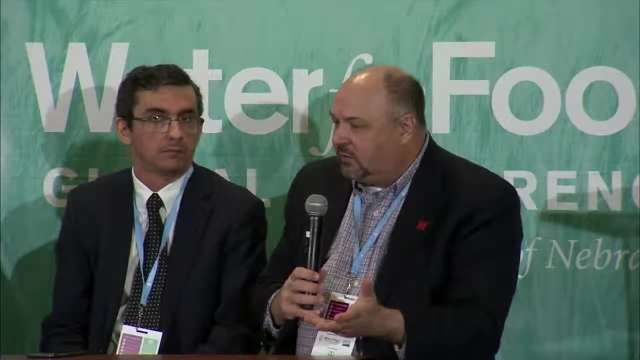 was a huge surge of people commiserating, if you will, and getting their message out and their voice out, And that's sort of a nice indirect validation of our Drought Monitor as well. So we have some current and she's doing research now. 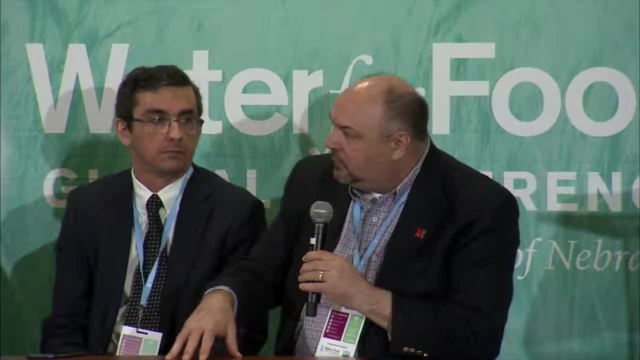 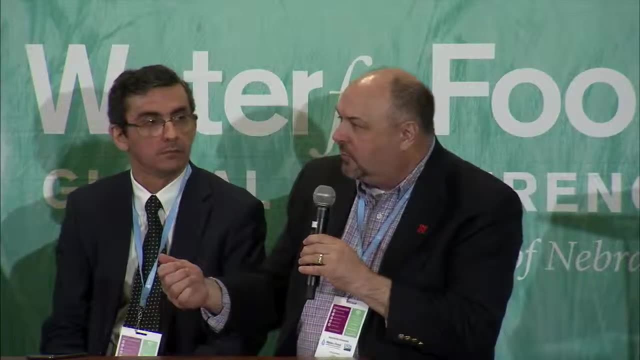 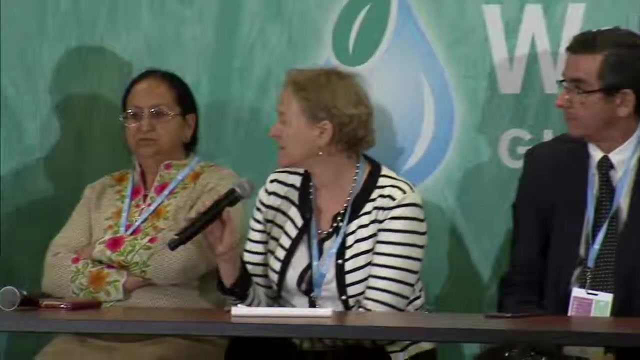 on her dissertation that looks at tweet, tweets and Twitter feeds and the survey activities and mobile phone collecting photos sort of in a longitudinal way to look at conditions over time. So that's my example. One of the areas that we've been looking at is data. 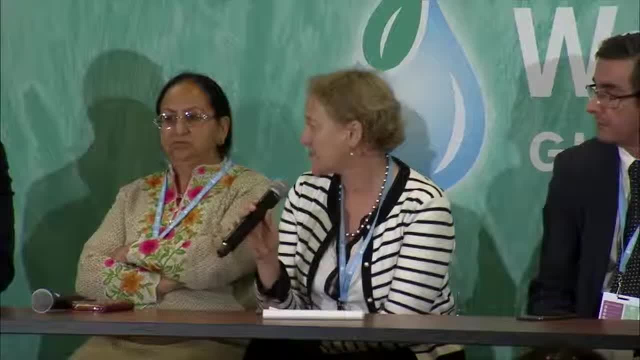 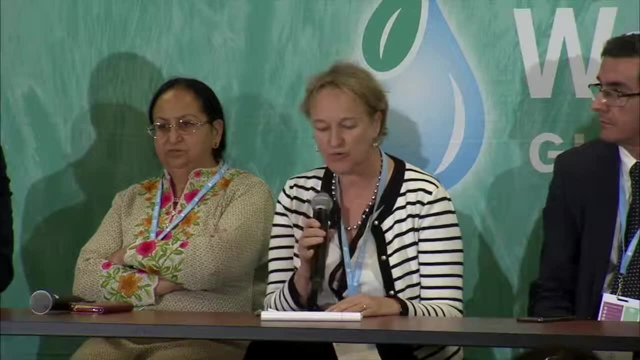 that we can support insurance companies Because at the moment, the great liability of drought comes along. it's expected that the government will pay, And so what we've been doing is we've been working with some insurance companies looking at how can we take some of this data but make it in a form. 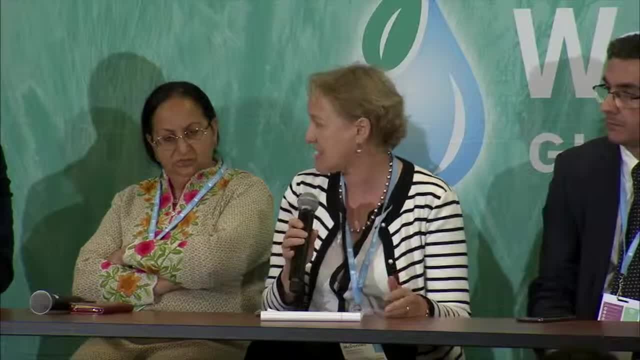 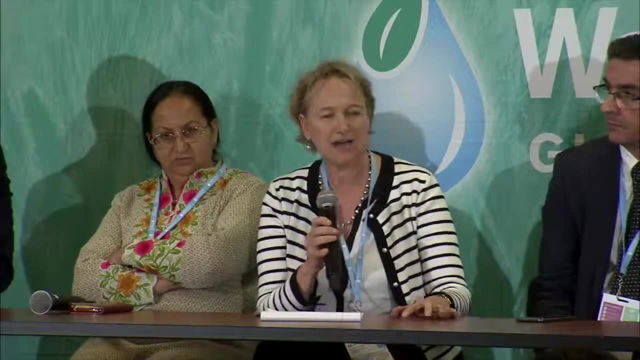 that insurance companies can use to then make payouts. For example, in Lebanon, when a drought comes along. it's called the National Crisis Center And this group of people. they go out and assess what has been the impact. How many goats have you lost? 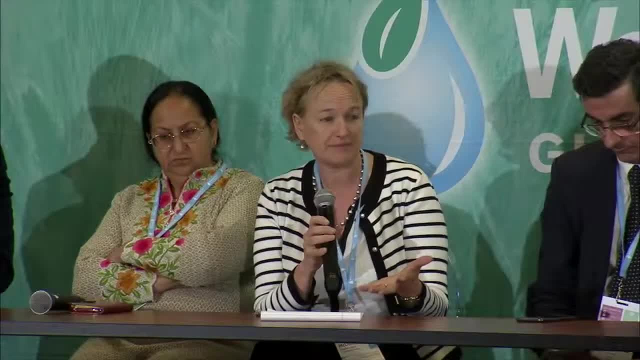 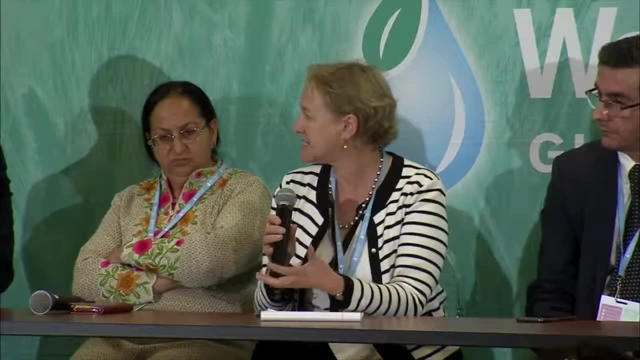 How much has been your yield. But the people doing that are from the army. Now their ability to make this assessment is there's not the training there, So it's like trying to go. how can we get different data to support crisis funds or insurance? 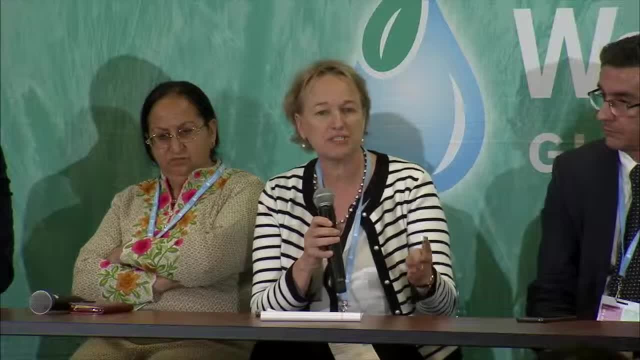 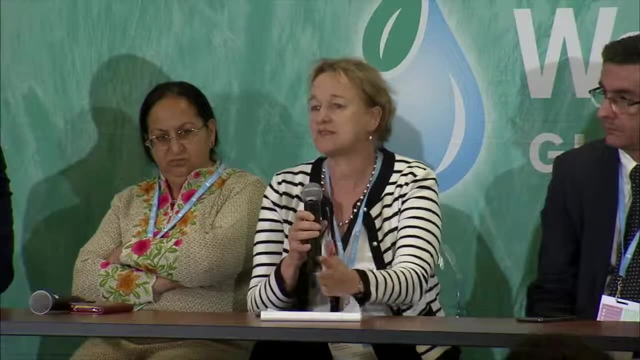 companies, whoever it is, to make it a much more, Because what's important is not just the impact of the drought on this season. If we can get that funding out quickly, the farmers can then buy the seeds and the fertilizers for the next season. 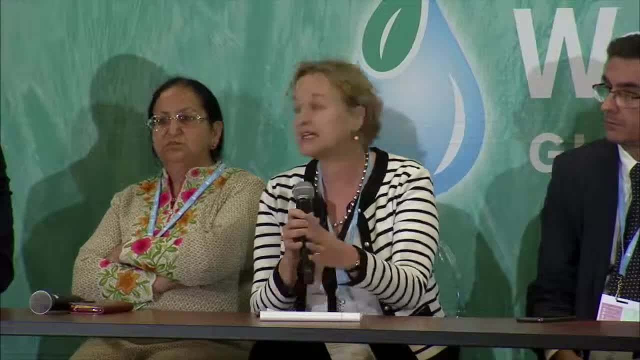 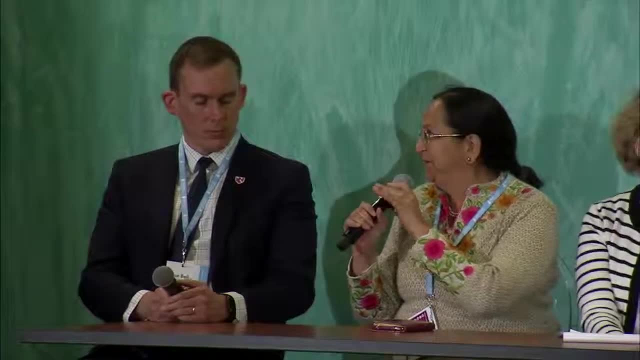 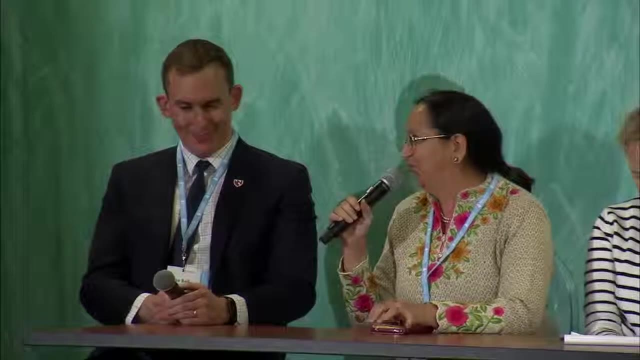 So the drought doesn't impact the next time as well, So we can limit those impacts. It's a very good question, I mean. I would say it's like a dream which one would like to have. How can we innovate in having better data and consolidated 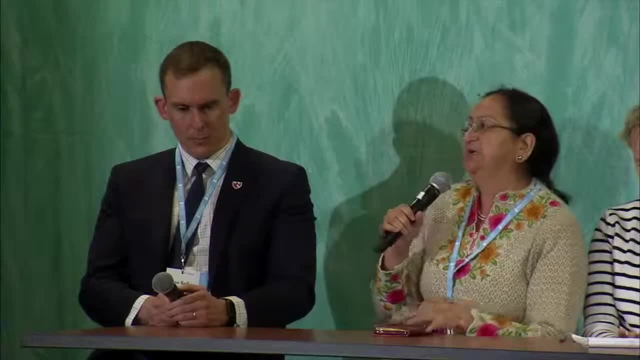 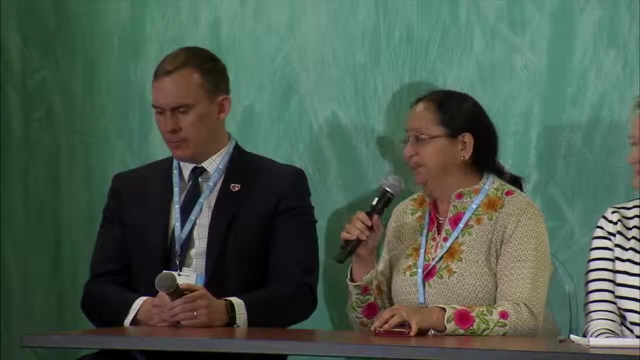 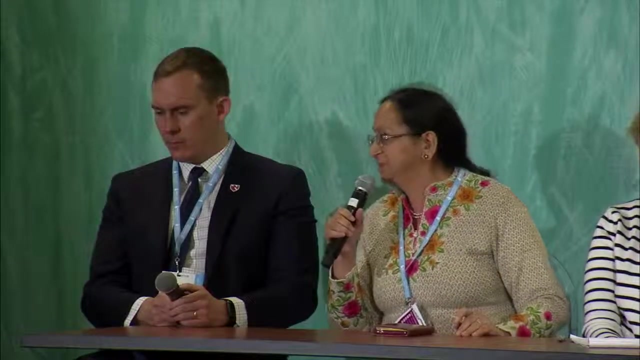 data under one umbrella. So this thought has been going on even in the Indian ministries and in the mind of the Indian government. But before saying anything- because it's always very easy to say But very difficult to operate it on ground, If you look at the Indian canvas, 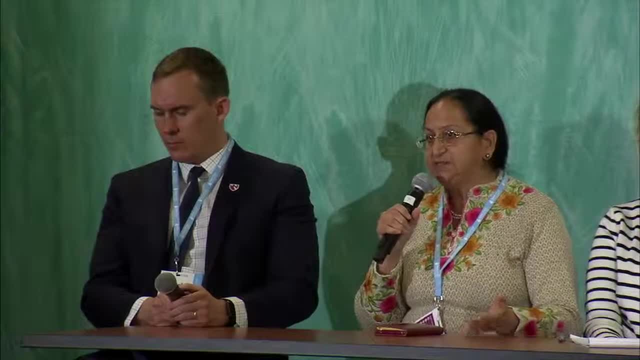 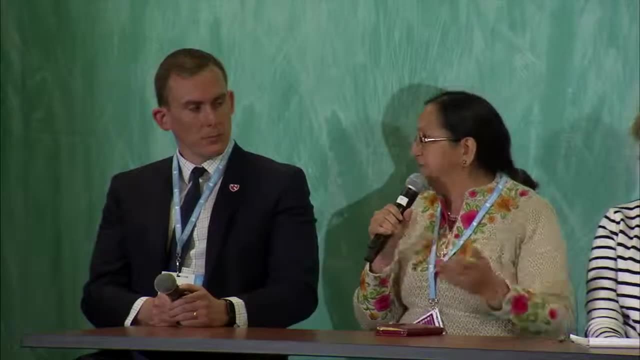 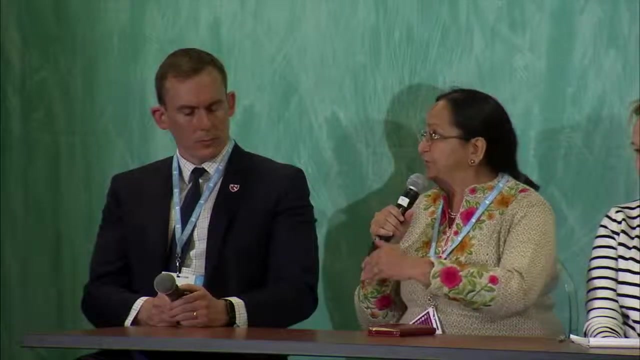 it's not like one country, It's like a subcontinent. Each state is like one country, And then within the country, there is so much of geospatial diversity, And there are diversity in terms of what are all operations are going on, but also diversity. 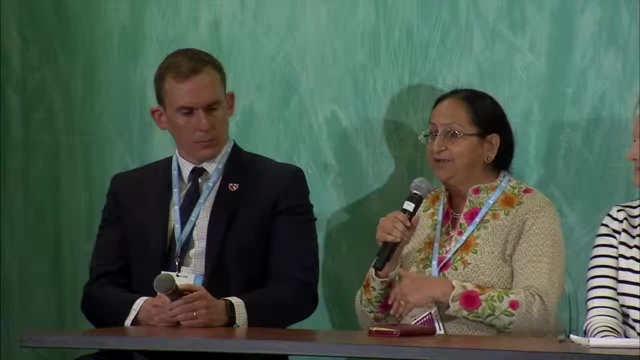 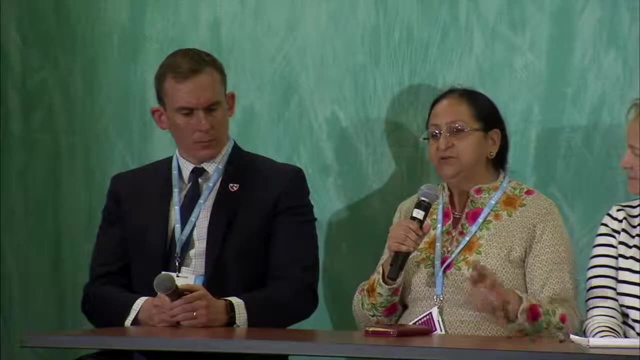 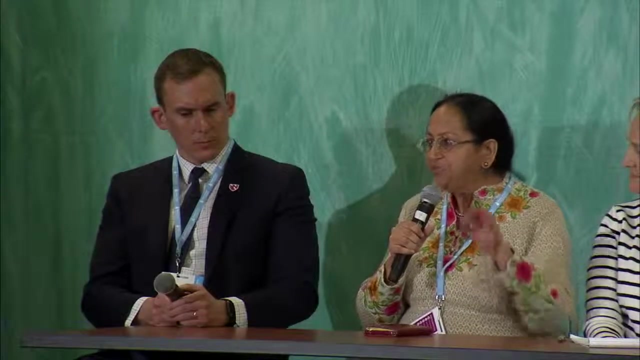 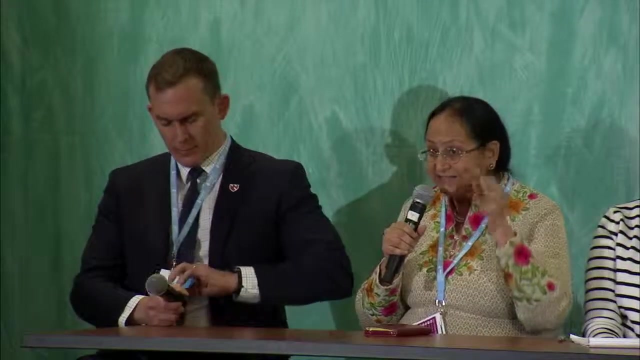 amongst the actors who are taking care of those operations on ground. But having said all that, I would say that, in spite of all that diversity and the vastness of the country, we have an exceptionally good structure, organizational structure which actually exists even as of now. 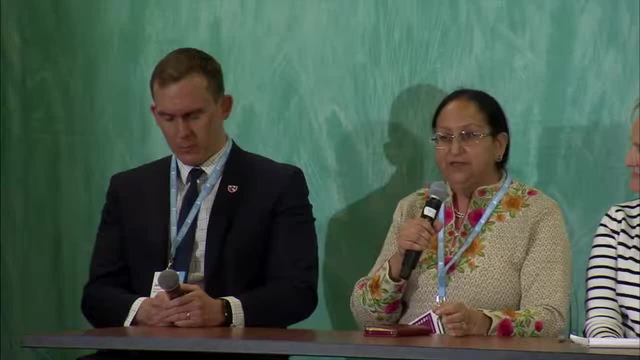 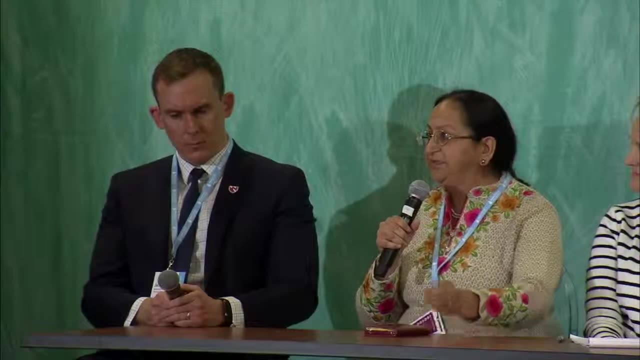 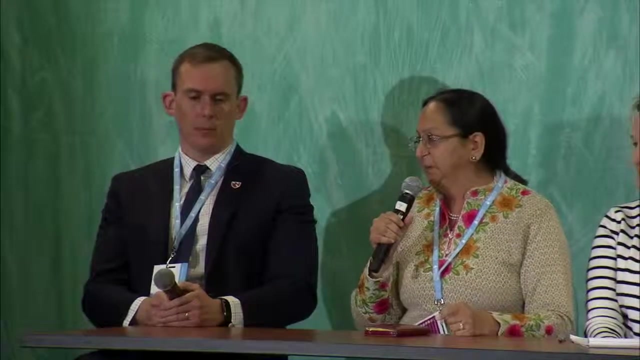 The only problem, as Mark said, it's the people. With what level of integrity and truthness you really go down and dig that data and put it in the repository. If you look at the data like I did- a study for national capital- 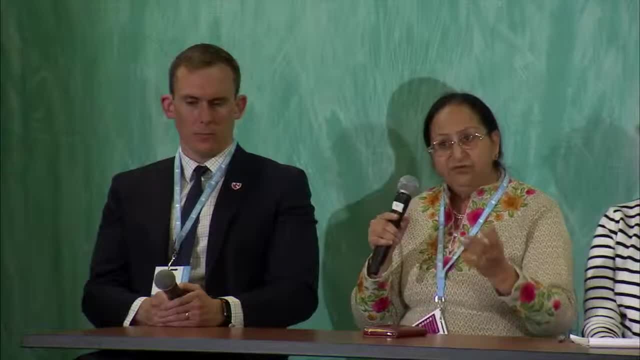 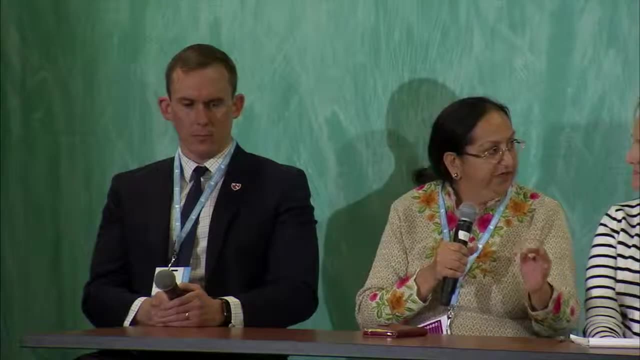 region, which is a region, not a state. It comprises of three, four states And I could clearly see that, if I look at the data before 1980s, it was beautiful data And you can make out that it is correct, real, because it was. 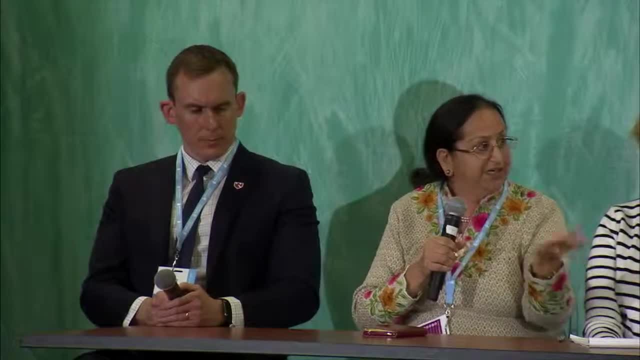 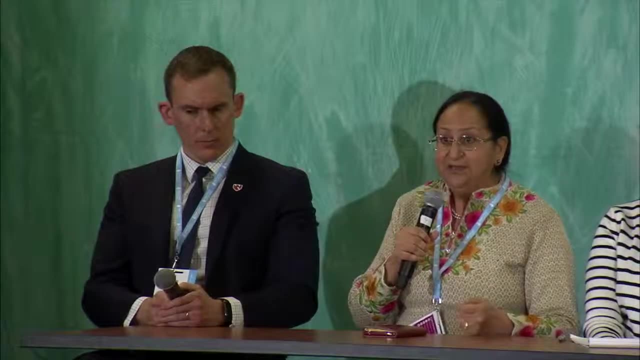 in sync with various other phenomena. So I could cross-check it against this, that and everything Like. if a person is sick, then you can check his BP and then also check other health parameters And then you are very sure whether one is healthy or not. 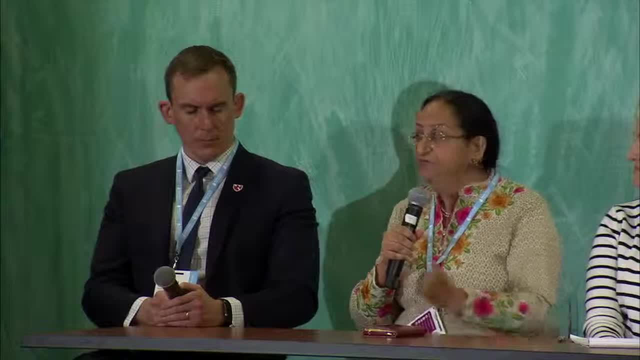 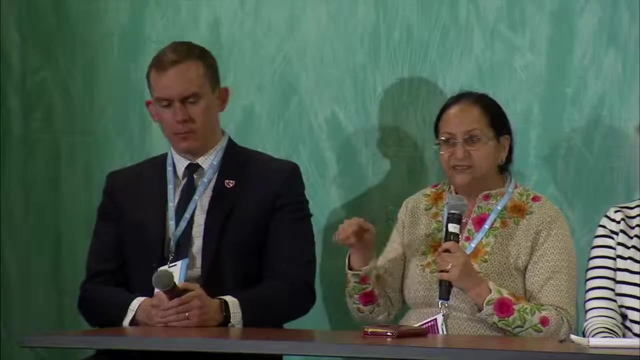 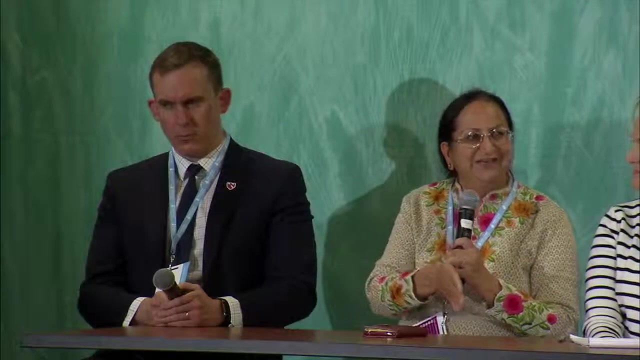 So similar exercise was done on this data, But after 1980, I could find that there were many glitches in that data. So it only goes to state that the ethics and the integrity of the people who are there responsible for monitoring that data is not 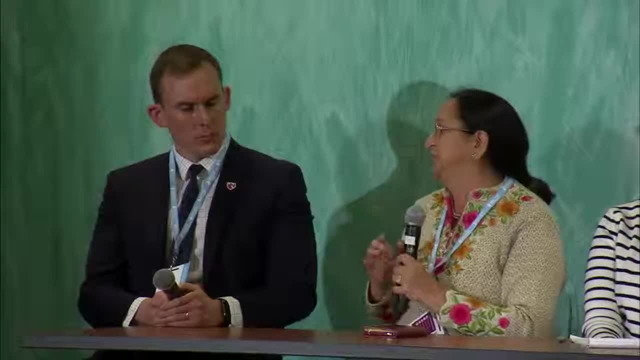 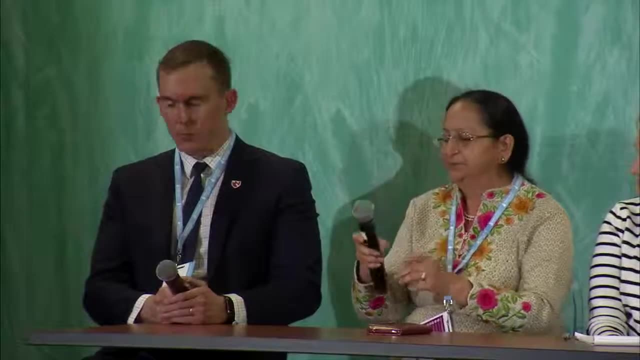 there, but the infrastructure, structure, organization, everything is there And it's a beautiful organization. If somebody takes good care of that, we can have excellent data generated, And I just want to quickly jump in on that as well. Any time you're doing anything that's health-related, 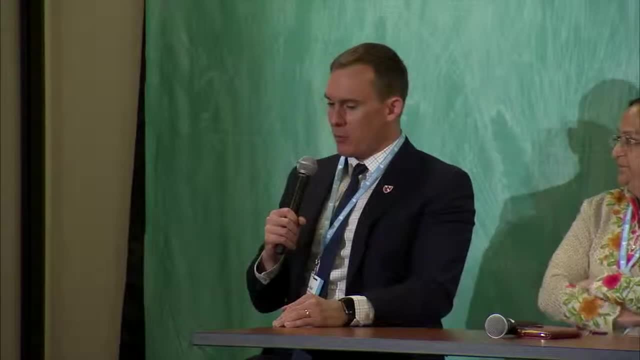 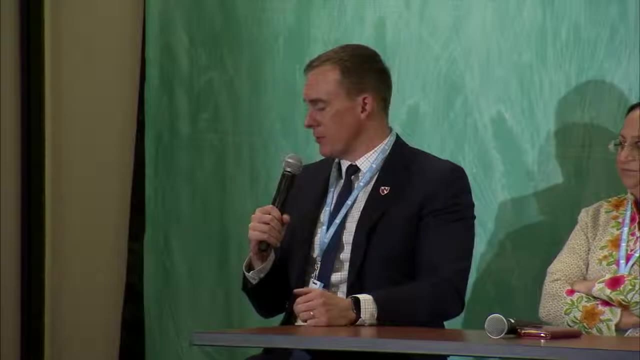 access to data is a huge issue. Trying to find large data sets that are health-related is almost next to impossible, And if they are available, there's a lot of suppression issues with them, especially here in the United States, And so one of the things that we're doing- 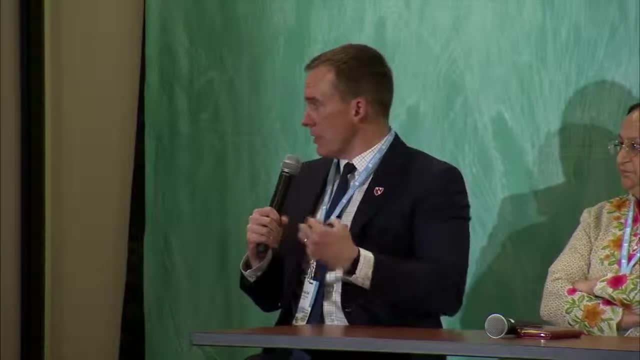 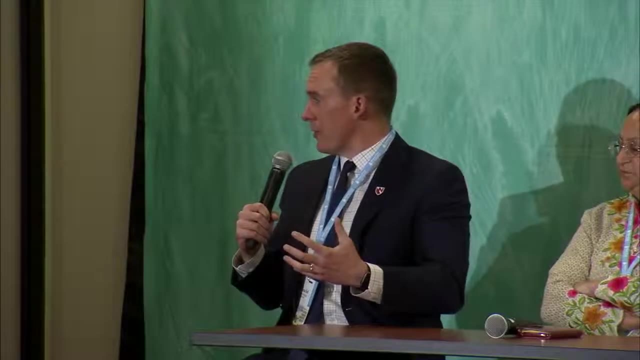 is trying to address that by doing some data mining techniques to try to pull out some of those relationships, Because it's already so complex just trying to deal with the complexity of drought on human health- And then you try to add in some of the data limitation stuff. 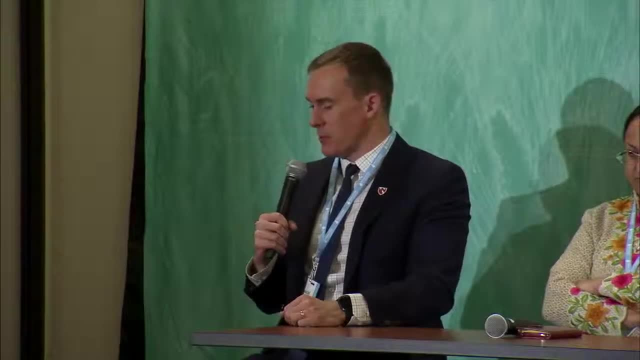 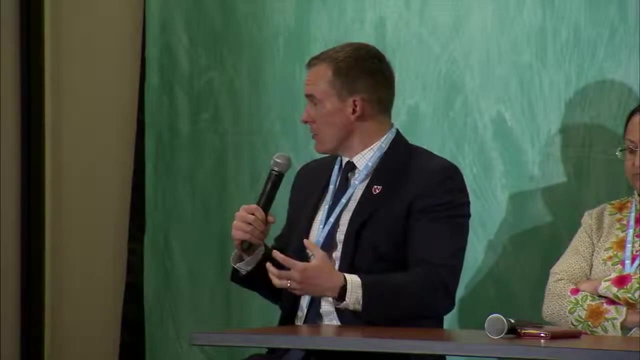 that we have here in the United States when we're trying to understand some of these relationships. But then one of the things that we've been looking at is how to get a hold of maybe other data sets that can show you some of those relationships as well. 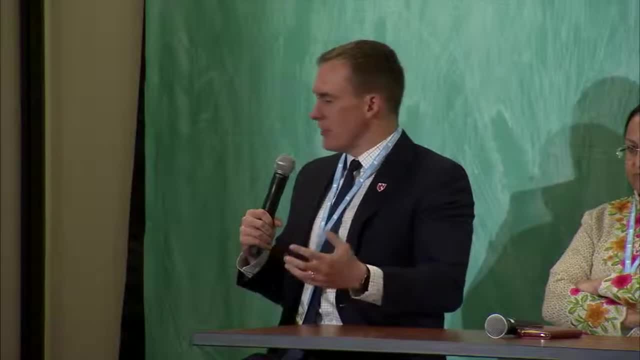 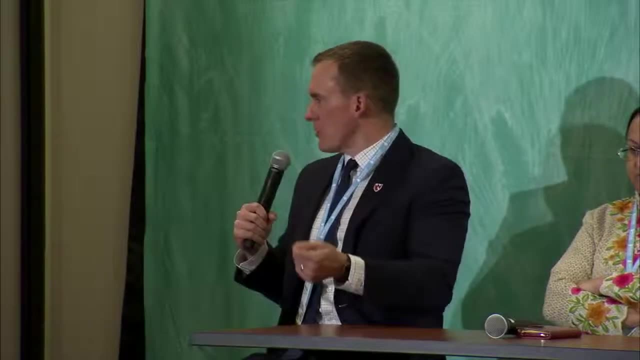 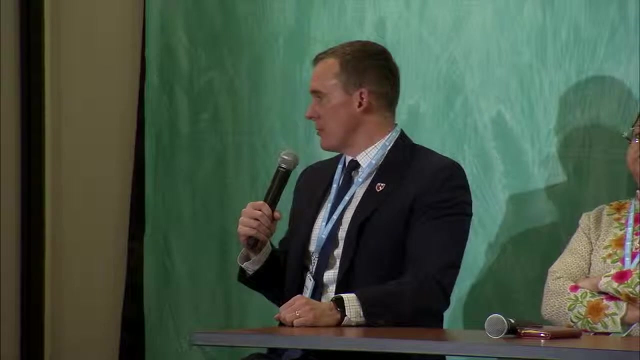 So things like WIC or those types of data sets that maybe can give you some understanding of community stress in some capacity. And also when we were at CDC, we also provided surveys out to the state and local public health officials, And I thought that that was a wonderful way. 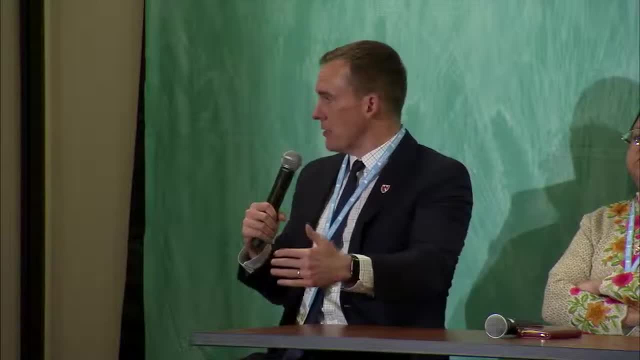 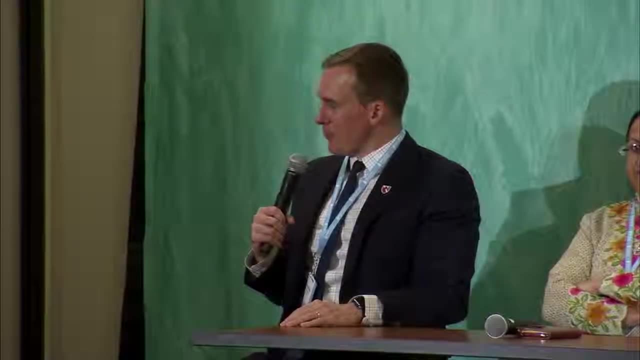 because then you hear directly from the people on what they're facing And you're not necessarily trying to mine that out of the data itself. Now that doesn't really get to the point of how do you forecast that moving forward, But we'll try to tackle that at some point as well. 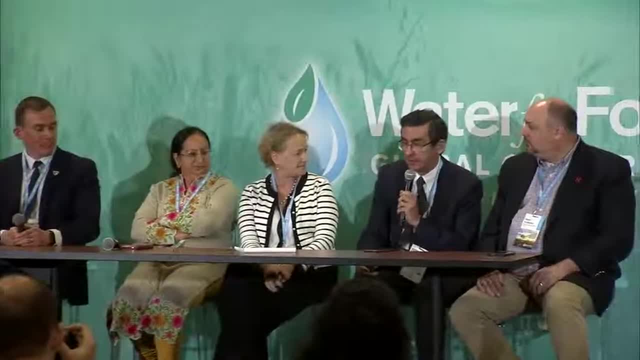 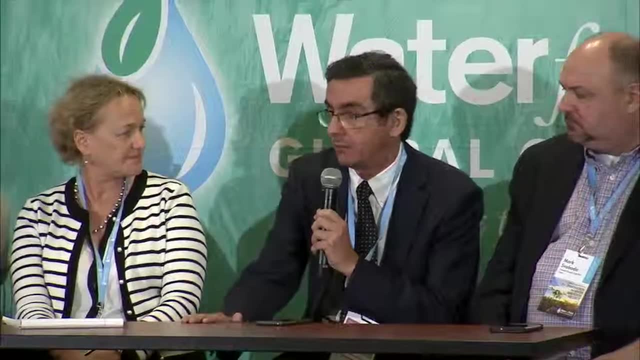 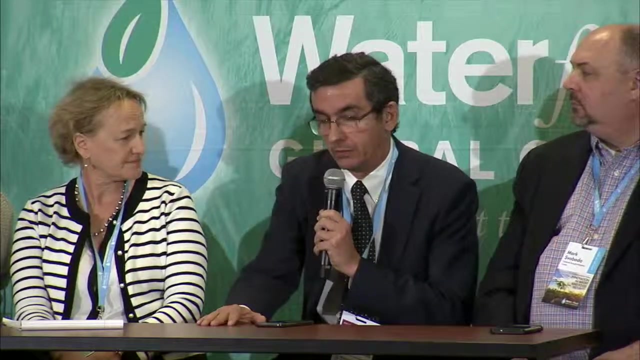 I think one of the great results of the monitor process was the integration of all database that we have available in the country, So we have access to the federal networks and the state networks as well, And along with that we were trying to look at the network with the end farmers. 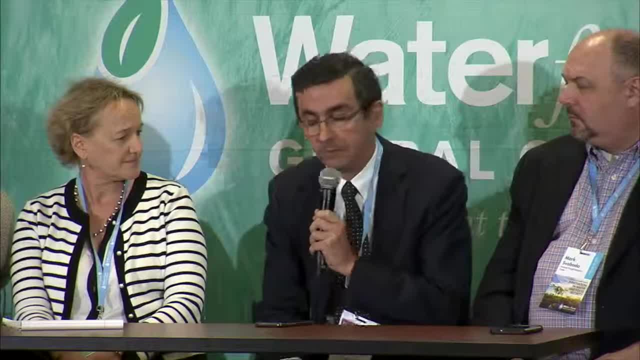 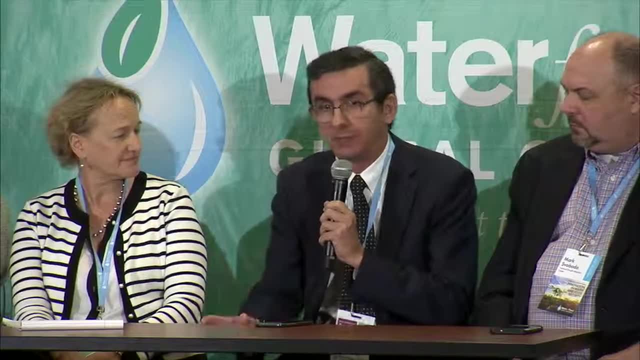 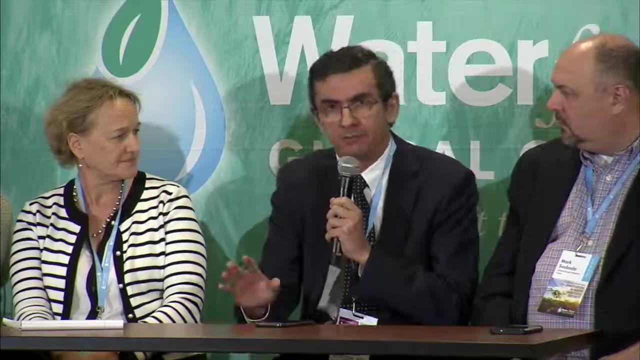 As well, so get the data from them as well. It's not easy task. We were trying to do a pilot in state that we have some experience with volunteer work on rainfall monitoring. We have like 550 gauze stations, rainfall gauze stations. 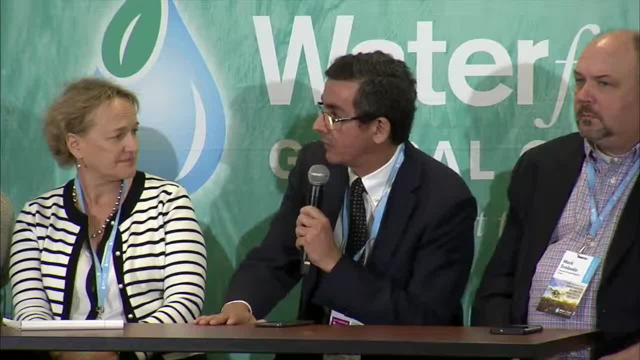 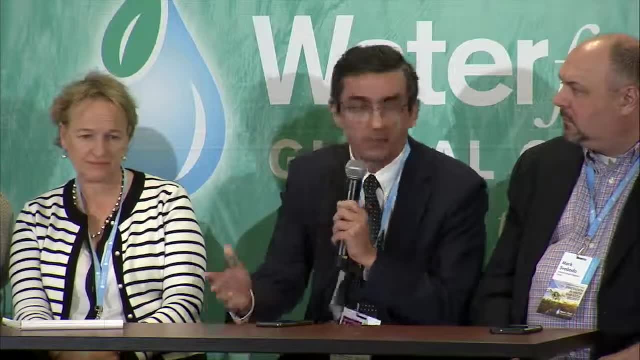 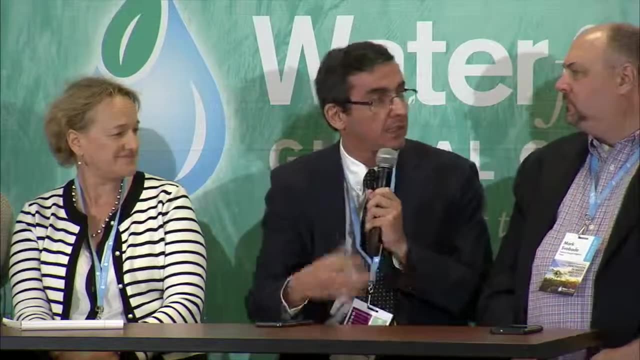 Basically, volunteers provide this information to us And this complements the automatic weather station. So we have a lot of data that we can use to monitor the weather stations network that we have. So we have to be innovative. Also, we are looking at some text mining, if you will. 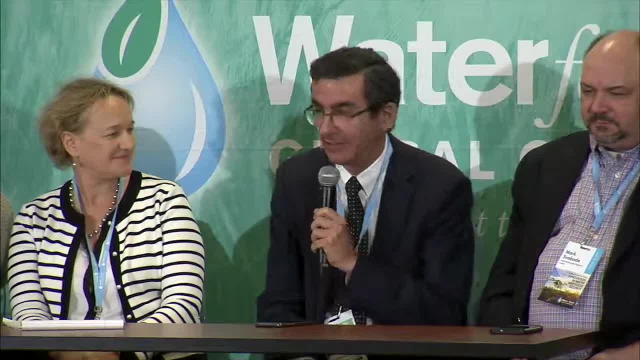 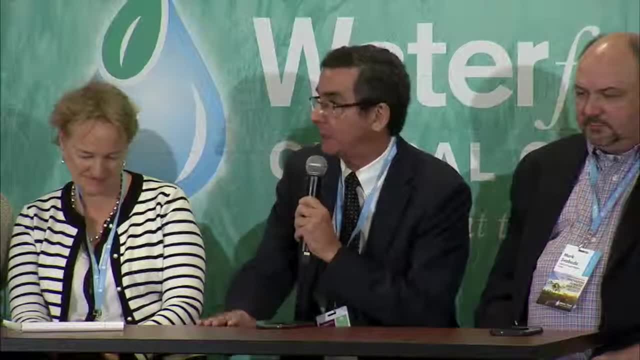 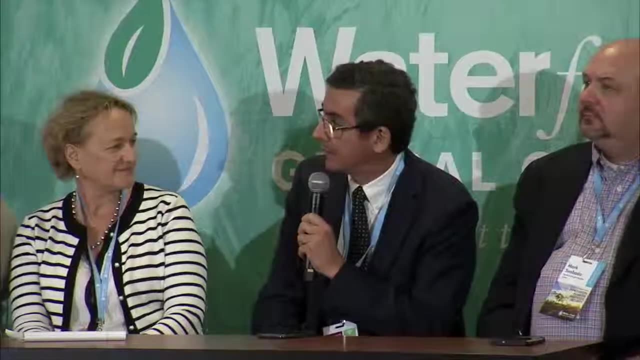 in those media, But there is a lot of gray documents there. We have to really look careful if it's really a drought or some I don't know misinformed reporter that's trying to raise attention to that particular region. So there's a lot of work to do in this area as well. 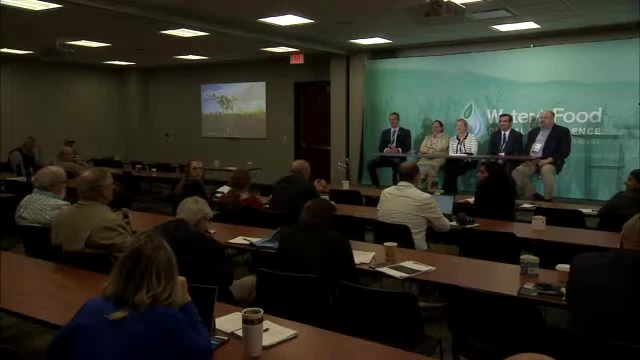 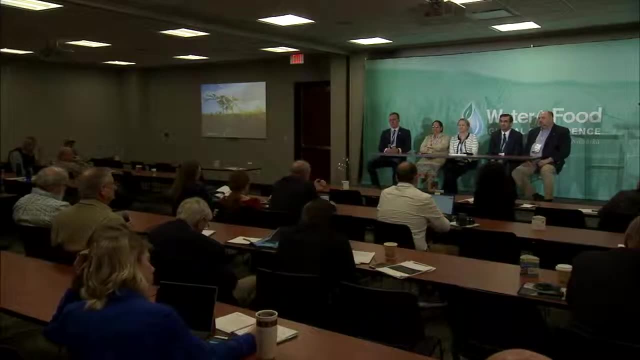 I would just like to say I think human nature really is a major, major issue when we talk about water at almost any level And, of course, the whole question of climate change is a huge human nature discussion And it seems to me that the data that you're collecting 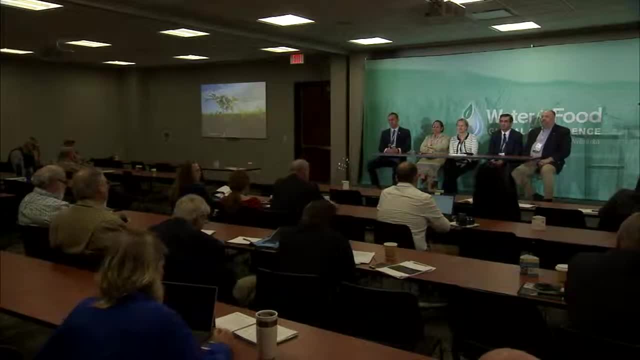 and the tools that you're establishing could be very useful for helping us Understand what's happened in the past and maybe even help make projections into the future, And it seems to me that the issue of making projections into the future is very, very important. 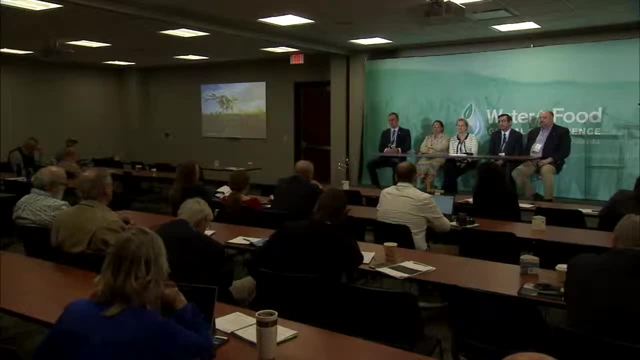 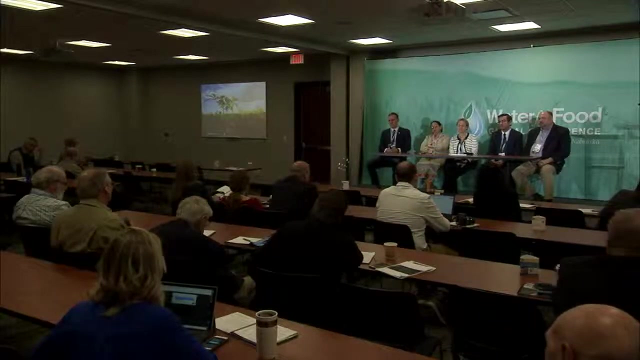 It's also very difficult, as one of the speakers alluded to. So looking at all the evidence for a changing climate that we've seen in recent years- the fires- tremendous fires last year, And floods that we've heard about here today- 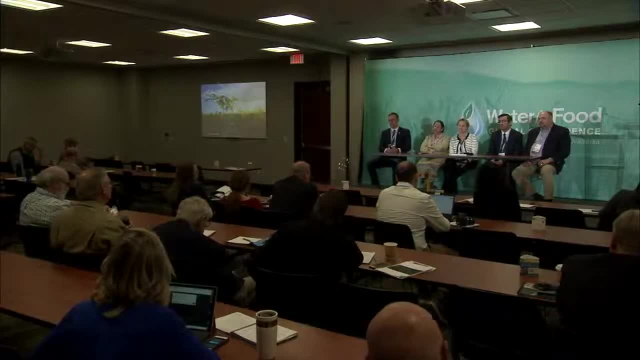 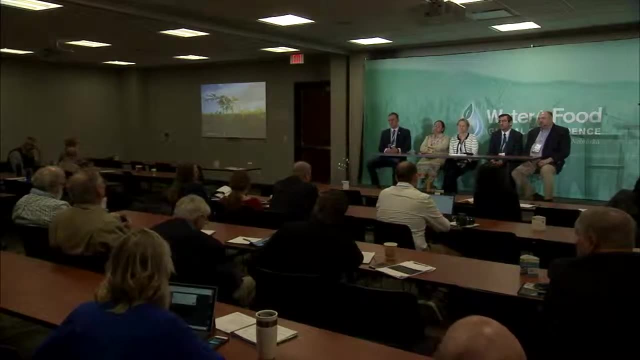 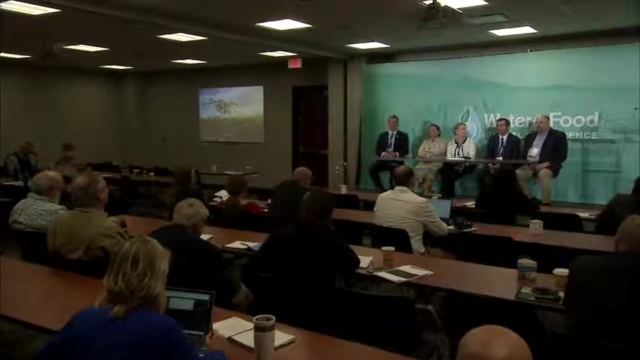 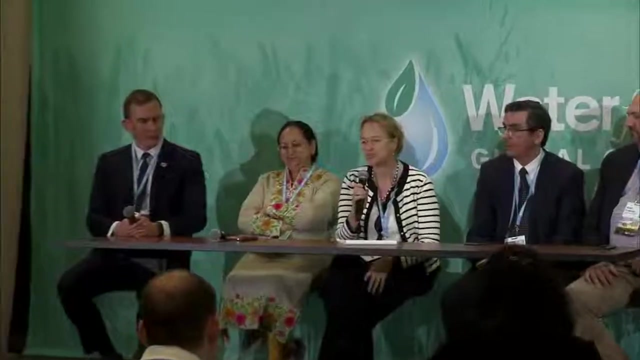 Insect infestations in eastern United States that are developing right now. How do we make projections into the future, Or is that even possible? So under phase one of our USAID funded drought project at ICWA, we have been doing that. 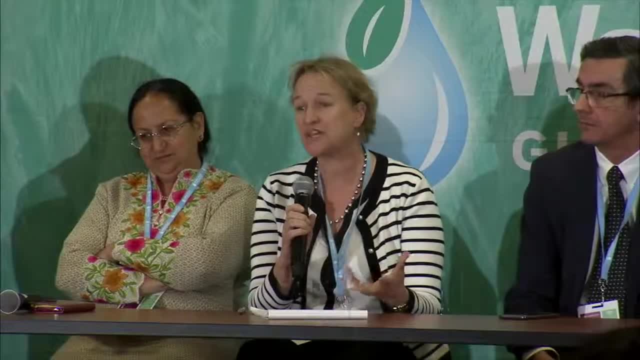 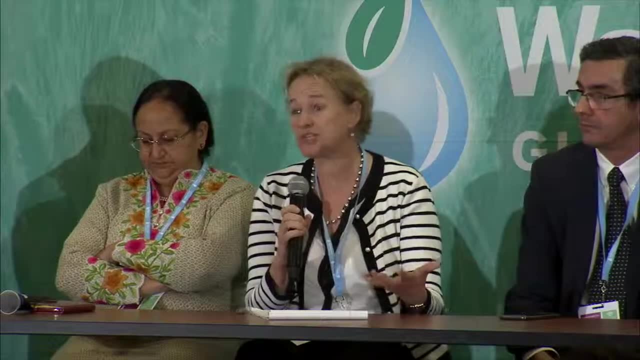 We've downscaled the climate change data And we're now looking at changes in the indexes called consecutive dry days, So we're trying to see how that's going to change. We know that the whole Mediterranean basin, the area that we're working in, is 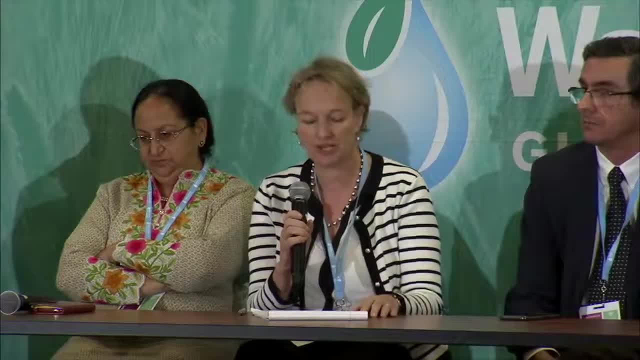 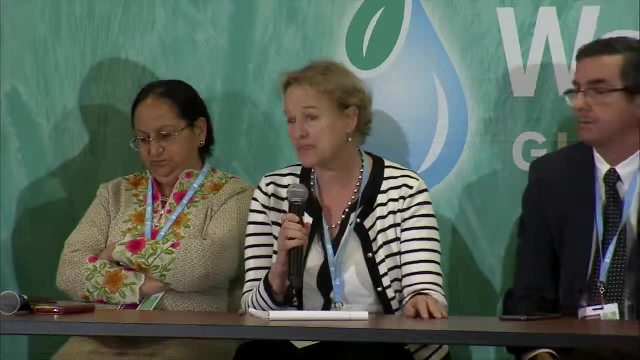 going to be one of those most affected. It's a hot spot for climate change, But what we're also looking at it isn't just the climate data we want to look at. So what we're looking at is we are modeling river basins. 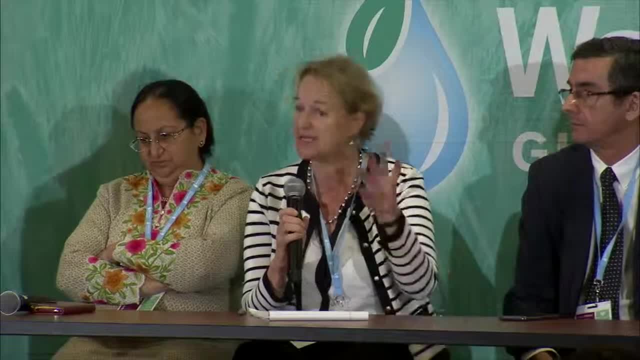 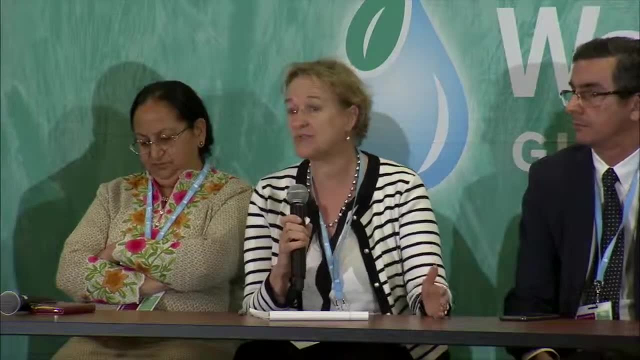 to look at how will groundwater, how will surface water, be impacted. We're taking eight model outputs. We're also running them through crop models, Because what we are interested in is the impact on water and food security And what we're trying to do as we're developing. 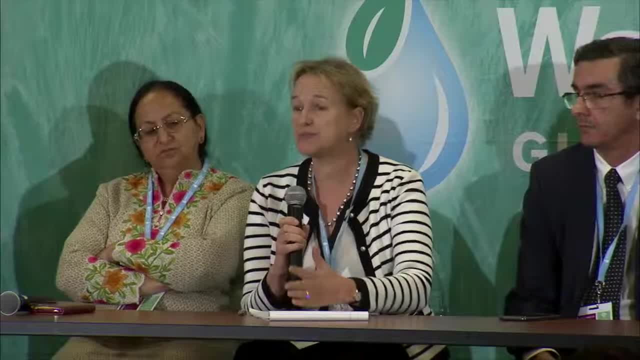 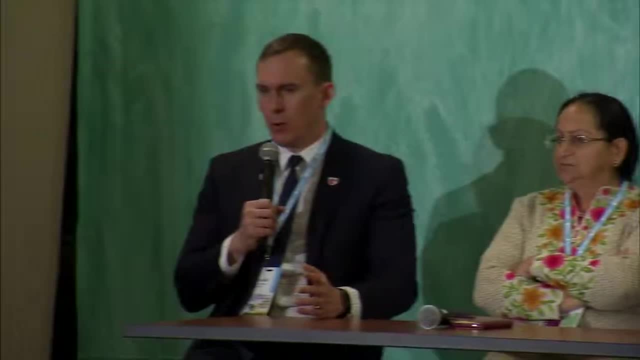 these reactive plans, proactive plans, trying to build in the resilience that will not only get us through the droughts today but also in 10 or 15 years' time. The health impacts are definitely harder to project forward and trying to figure out what some of those relationships are. 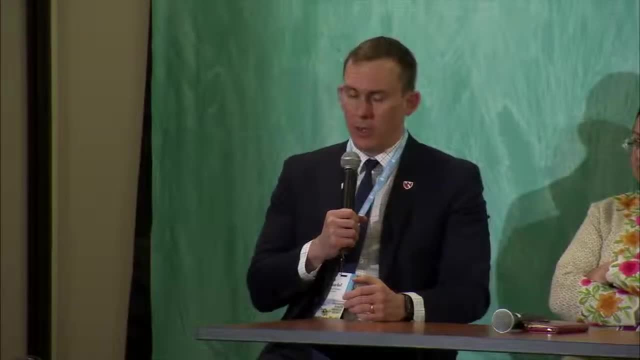 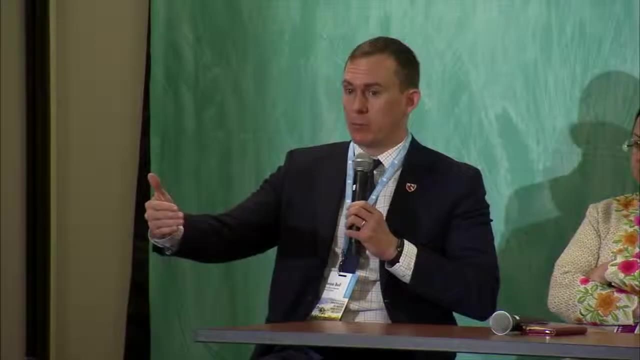 But I definitely think that it's something that we need to focus more on, And some of my colleagues at EPA have been doing a number of studies where they've been trying to project some of these health impacts. They haven't necessarily looked at drought yet. 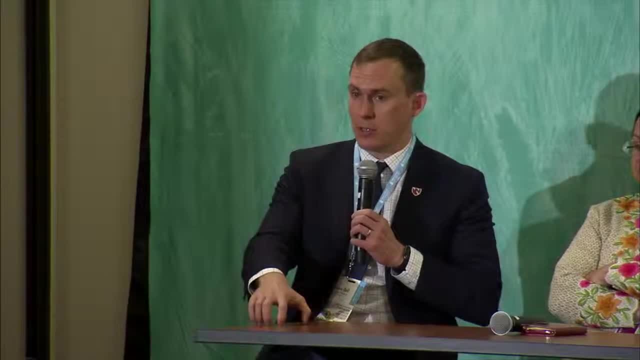 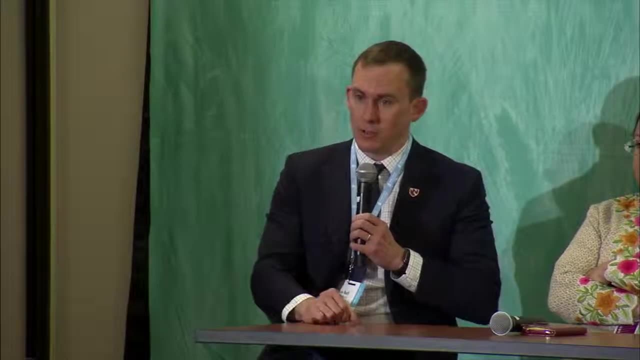 And that's actually one of the things that we've been talking about is how we potentially project some of these health impacts moving forward in looking at drought. But they have done things like wildfire and dust, which are obviously associated with drought in some capacity. 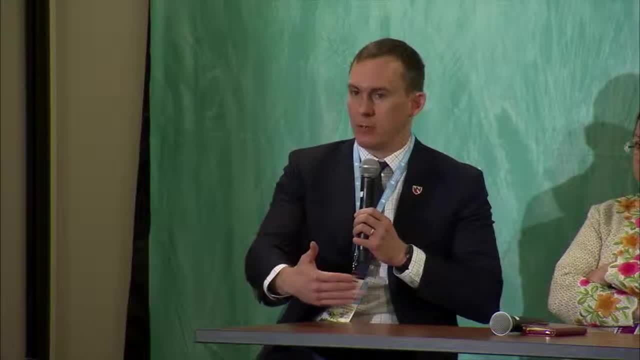 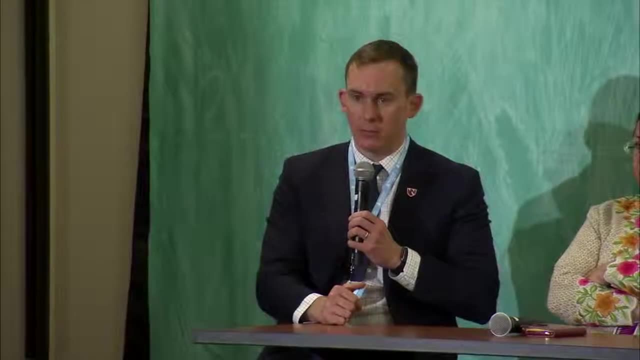 And so there's- There's already opportunities to make some of this work available, And there's already some movement in this area. So I'm kind of excited to see where it could potentially go. Actually, we've been doing some studies, The previous technical assistance of the world. 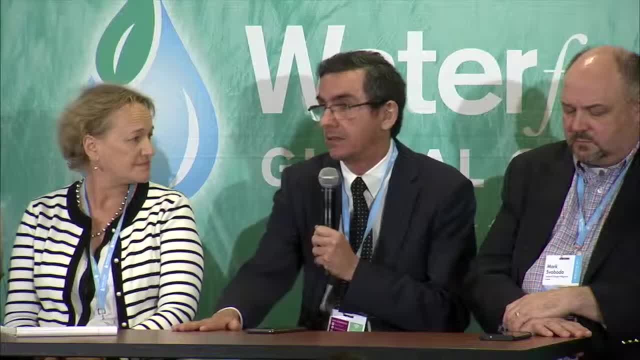 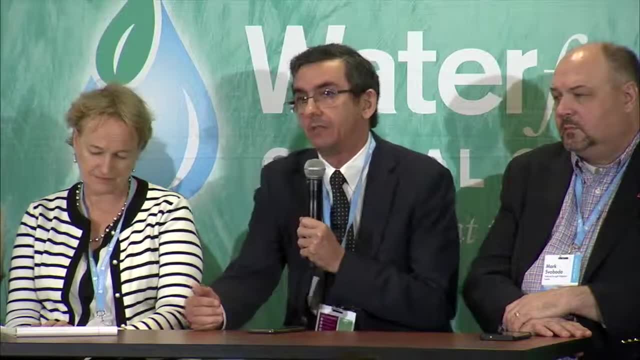 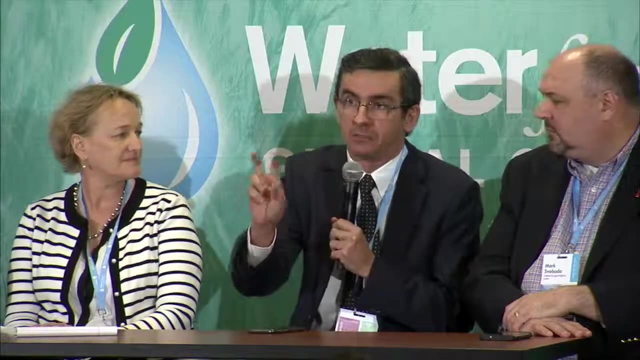 backings in my region was on climate change impacts on the water and agriculture sector And we've tried to make projections, but really not on drought, because we don't do prediction and drought with those models. We try to depict some characteristics of drought. 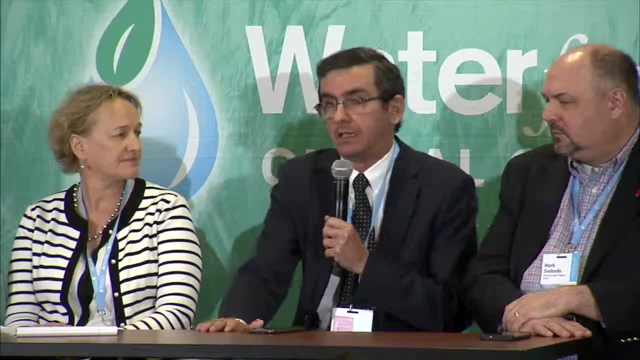 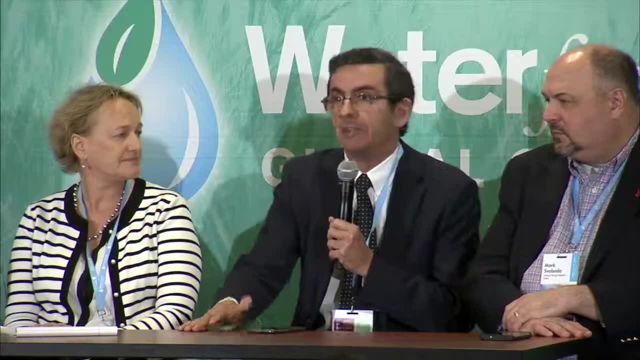 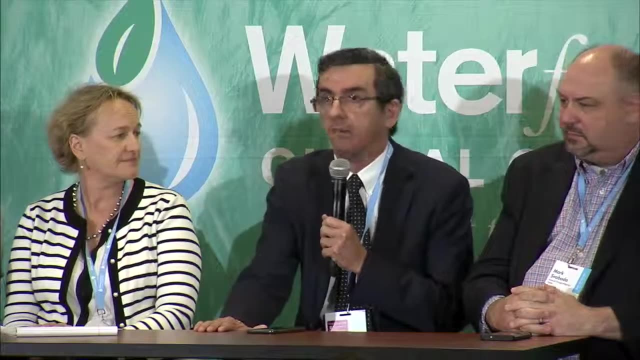 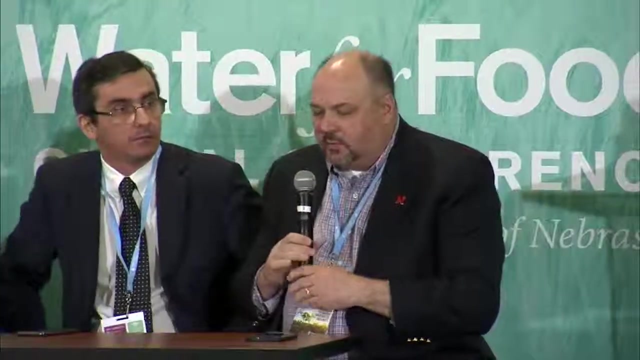 that these models can provide And for north of our region, most of the area would be increasing, for example, the number of dry days, consecutive dry days. That for sure will impact the rain-fed agriculture. I'll just add one thought to what you just said there. 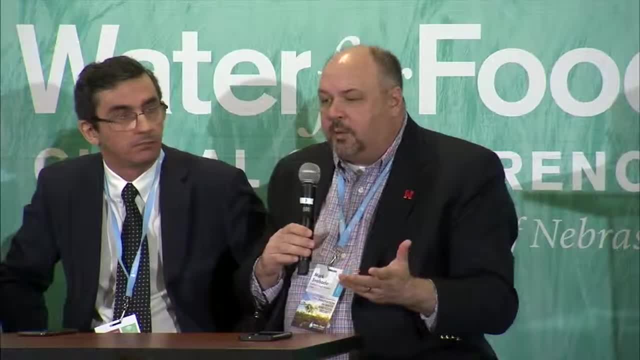 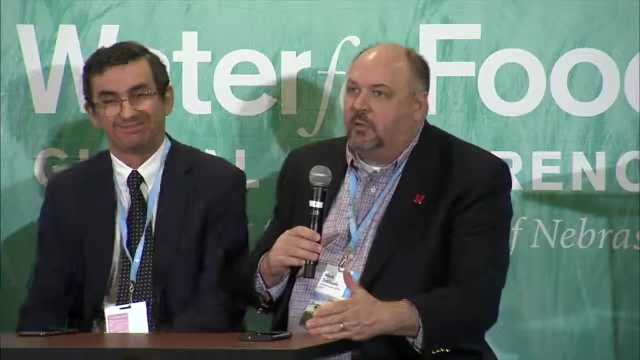 I think one of the things that we've been trying to do over those consecutive dry days is: to me, perhaps no hazard is more analogous to climate change than drought. It's the frog in the pot, right. It heats up slowly. That frog doesn't figure out until it's too late to jump out. 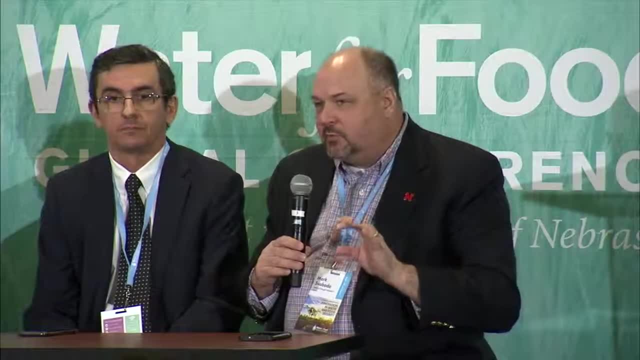 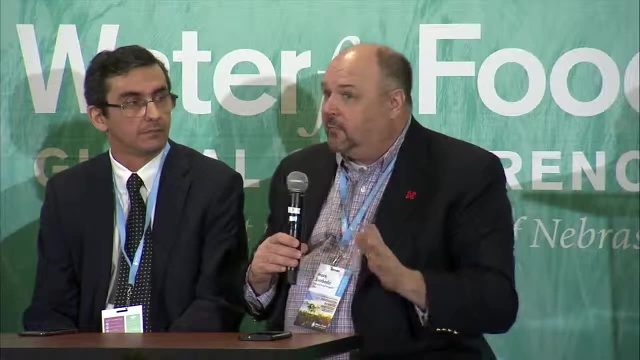 But it gives impetus to the pillar one, where all the more reason why we should be heating the day-to-day, diligent, week-to-week, month-to-month monitoring. And even then we stick our heads in the sand and don't react to it until it's too late. 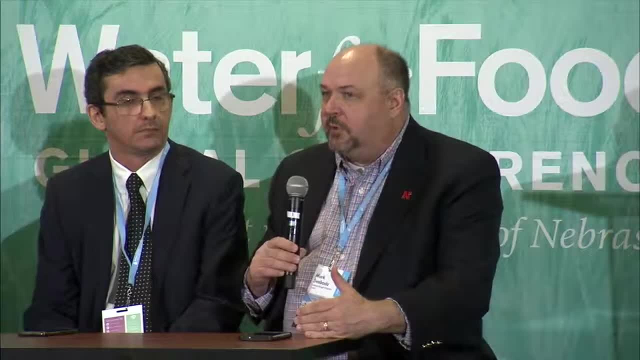 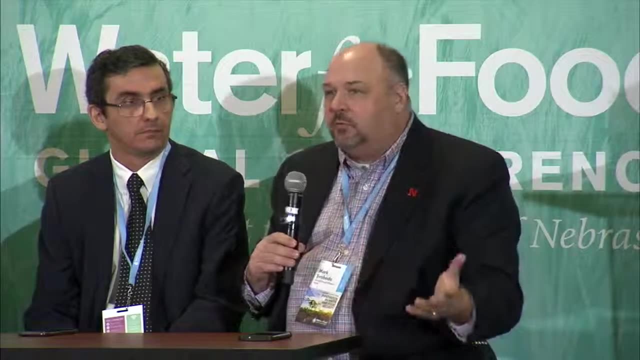 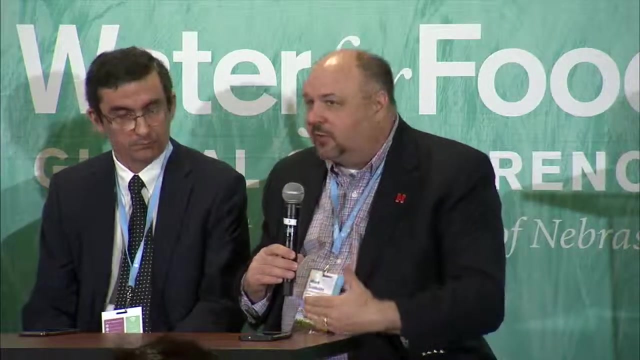 So these baselines are changing the frost-free period, the days between droughts. The more intense events on a crusted landscape causes more rapid flooding. Some of your worst floods are during droughts. because of that reason And the latest national climate assessments, 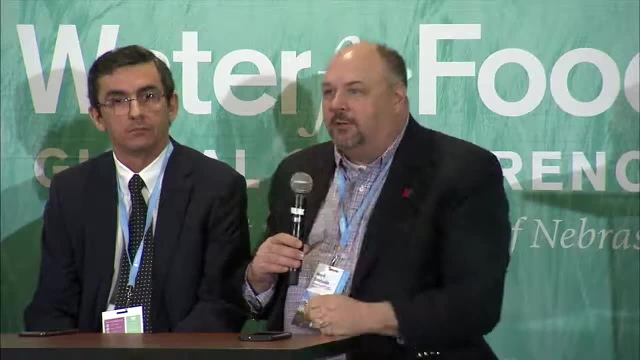 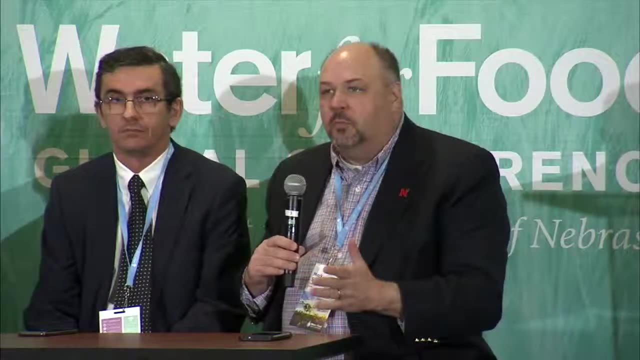 showing these statistics and trends are there. The guy right next to you, Dr Rowe, has worked a lot in this area with the Nebraska Climate Change Report that came out a few years ago. others in the room, Certainly more experts than I am. 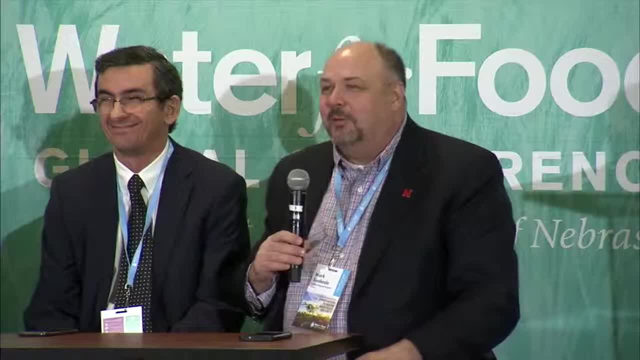 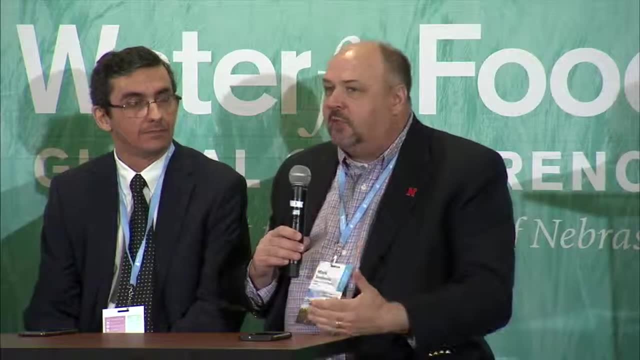 even though he taught me a lot of applied climate Going through there. that dates me, but I think it really dates you, Clint. So, anyway, I think these are all things. So the signs are there and people choose to ignore them often. 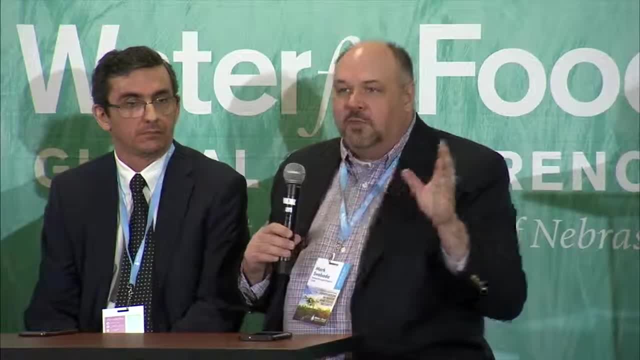 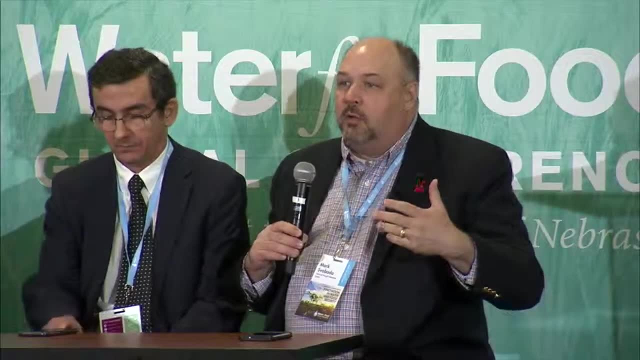 That we just got to keep fighting the good fight And you've seen the states that are planning for drought or for climate or other things are growing. FEMA is now requiring in the multi-hazard plans you're seeing drought integrated in. 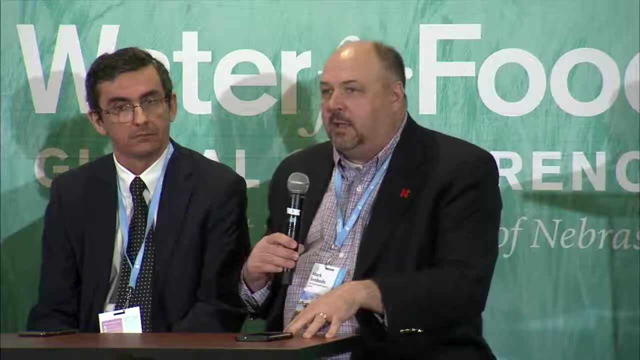 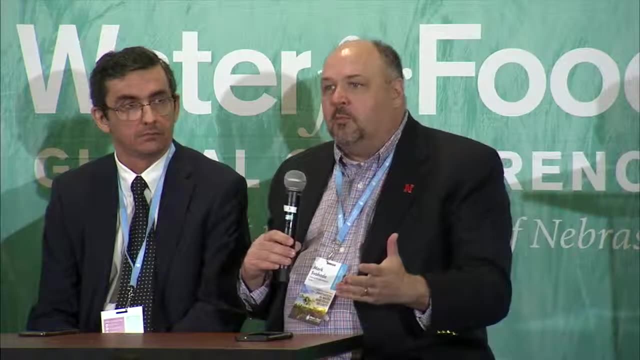 To other plans. so we advocate drought as a piece of any planning activity, Not just a stand-alone drought plan. but states have fewer resources, people wearing a lot of hats- Let's make it more. let's provide resources and guides to help them integrate it into things already on the books. 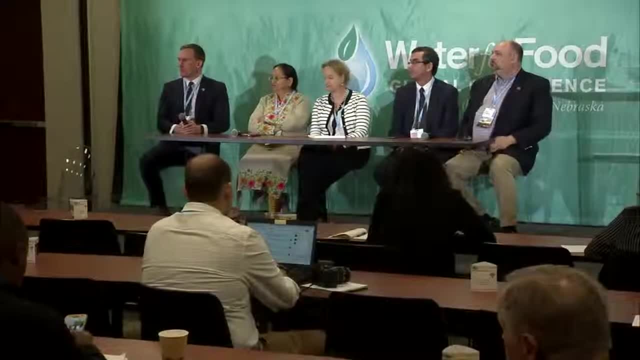 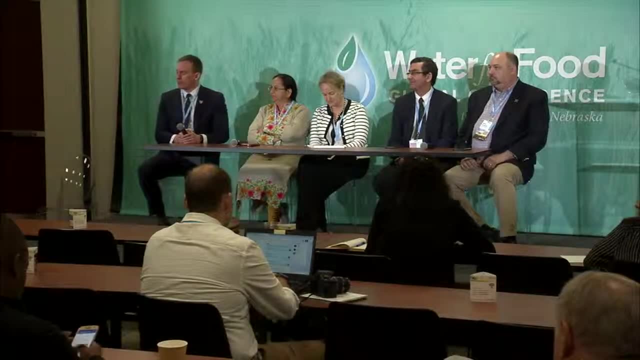 Whether it's a water plan, a master plan or a drought plan. My question is a little bit ambiguous, but I would like to see if you can clarify some of it. And it's about the social aspect of drought, And do you see the social intervention changing? 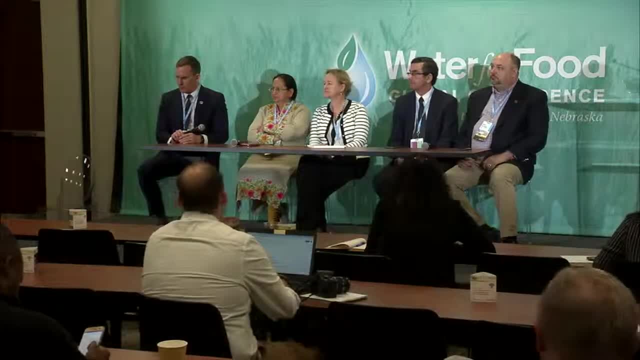 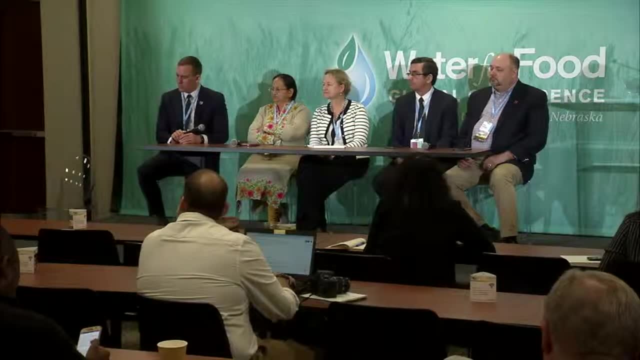 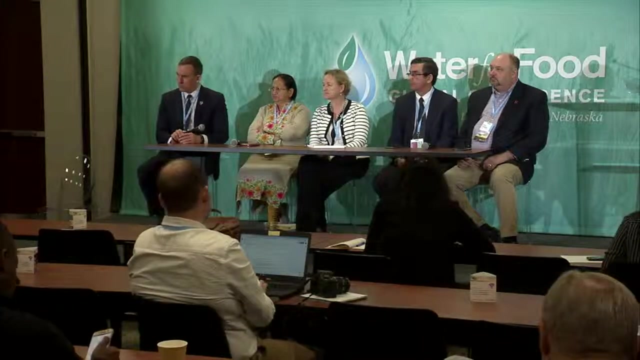 from a relatively passive way to a more active way. So far, what the examples that you have shown are lead by private, public sector, centralized entities, And the society is seen as the affected rather than the participant or the co-participant in some way. 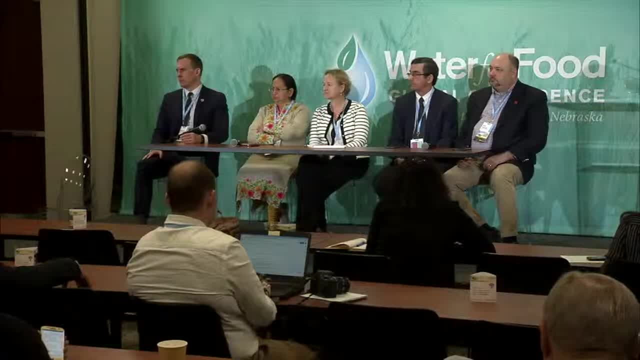 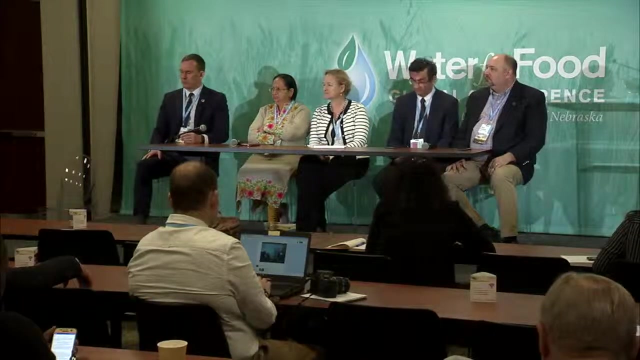 So what do you think about that? And what do you think about solving the problem or help to tackle it? So do you see intervention of society more active in the future? If it's not the case, how we can create a more social awareness? 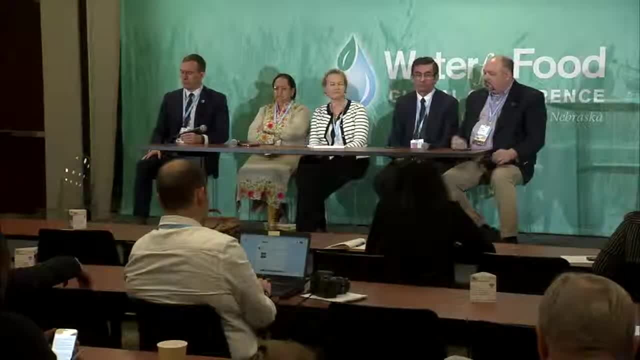 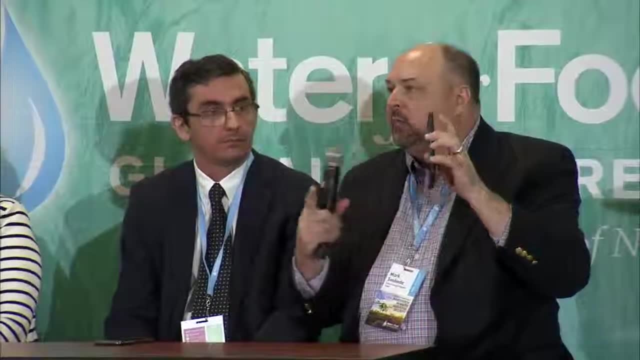 or society more aware about these issues. I'll just give you a one-word answer: yes and right here. Even when we were in Mali and Dr Wardlow and Dr Hazel, I remember a workshop we did there with the WMO. 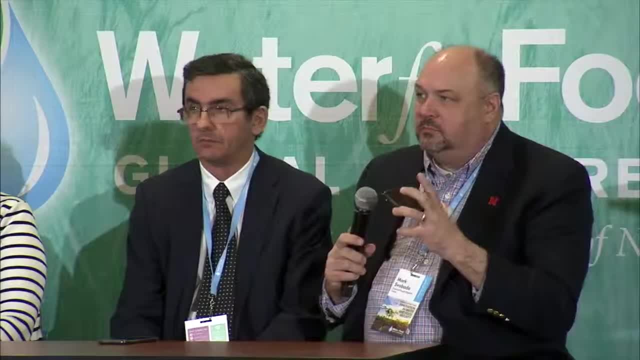 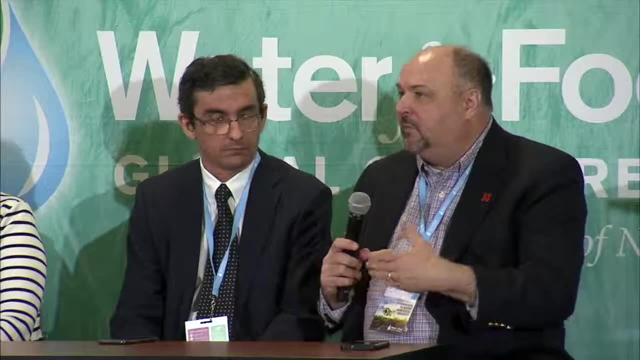 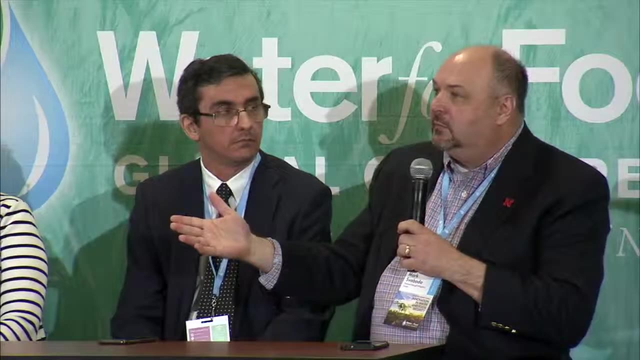 how they might not have much, but they've got a phone and it's a voice And I remember their med service. We couldn't hardly get data from them, But farmers and people out on the field in Mali, you wouldn't think that at all. 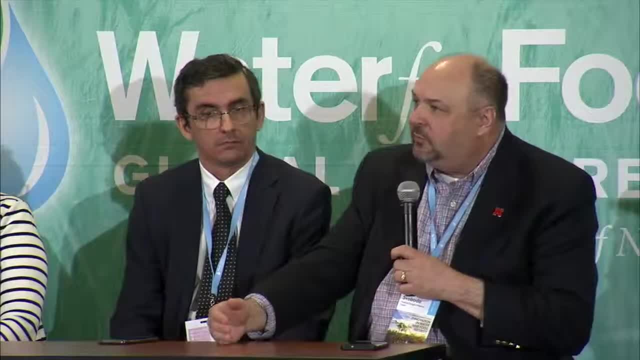 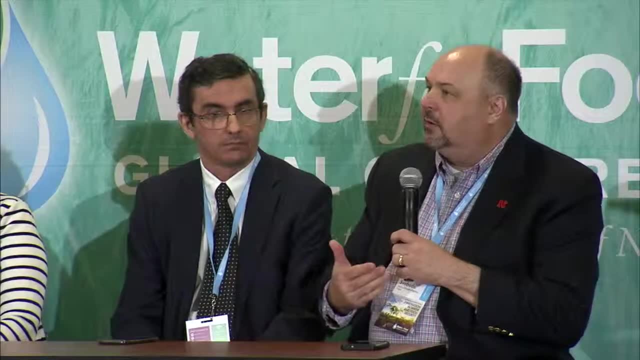 They've made the technology leap. They're providing information through those phones into the agencies at the state level or the central level, providing pictures of hey, we're hurting here on the ground. Hear my voice. I mentioned hashtag 17,. 2017 drought. 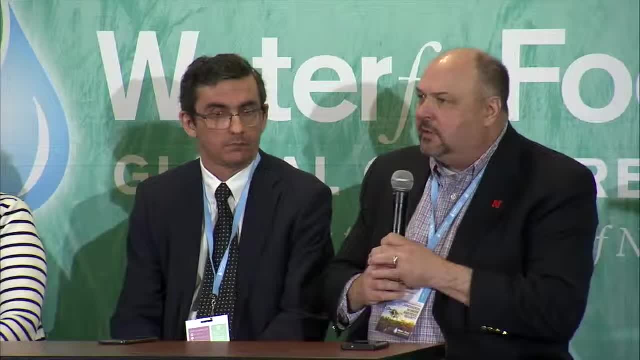 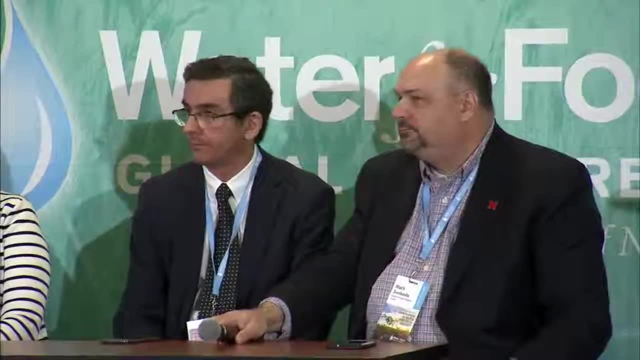 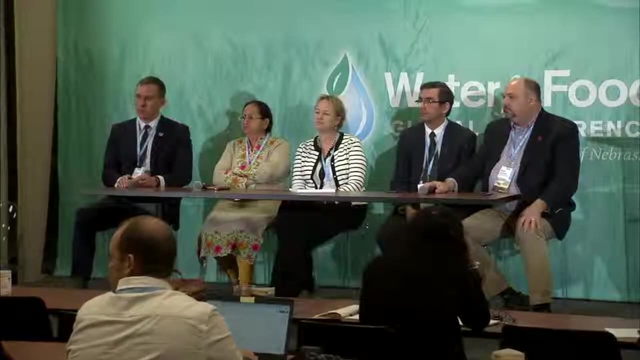 in the Dakotas for the livestock producers just a couple of years ago. So I'm seeing a much more active voice in social media and people being connected to their devices. What about private companies and their involvement in some of these things? Or Farm Bureau? 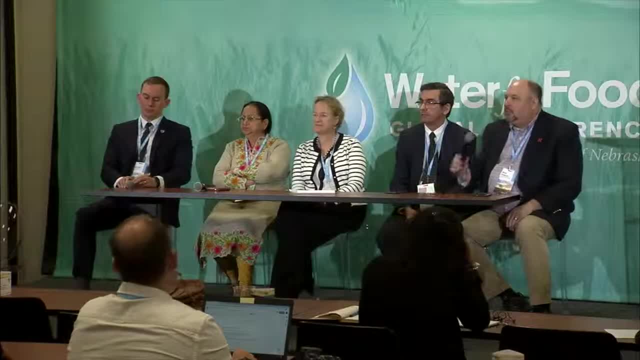 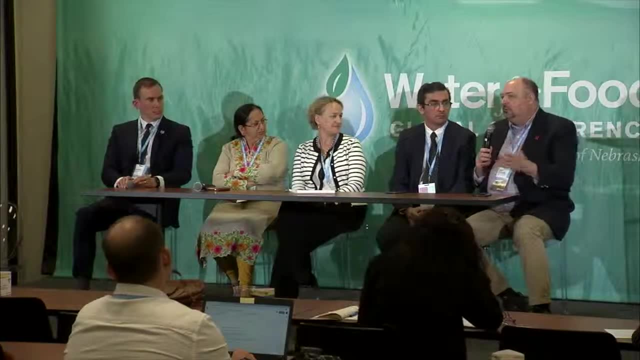 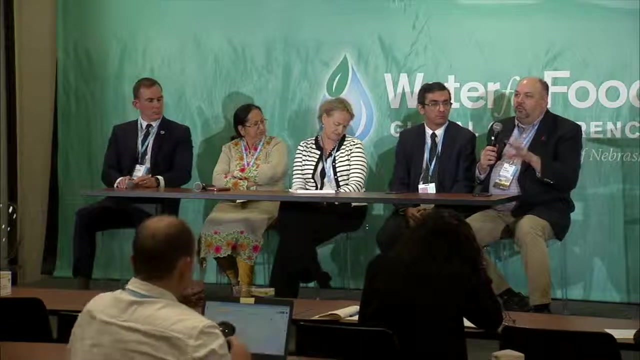 Or the State Department Or some of these NGOs. Are you seeing more involvement? Yeah, good point. We monitor, at least at the Drought Center, a couple of my staff- Actually Mike, as you recall- they're monitoring that blog atmosphere, those voices coming in. 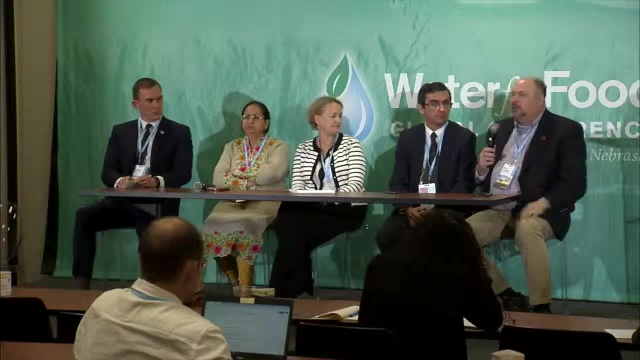 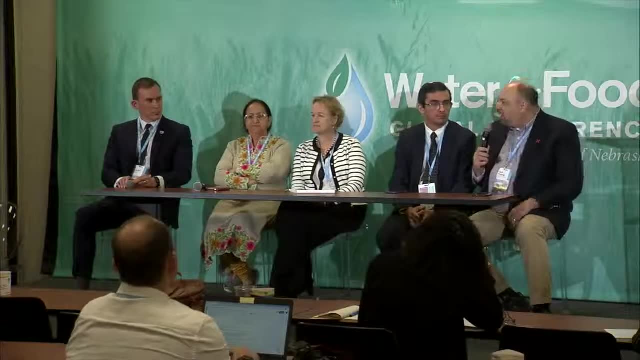 about impacts, what they're seeing, how it's affecting crops, livestock, through the Farm Bureau, through other agribusiness entities. So, yeah, I think the bottom line for me would be yes, And about others I don't know. 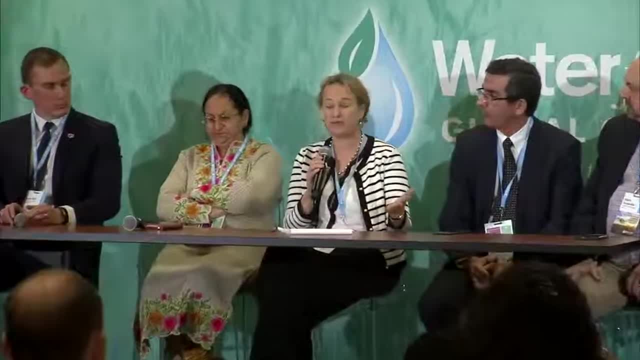 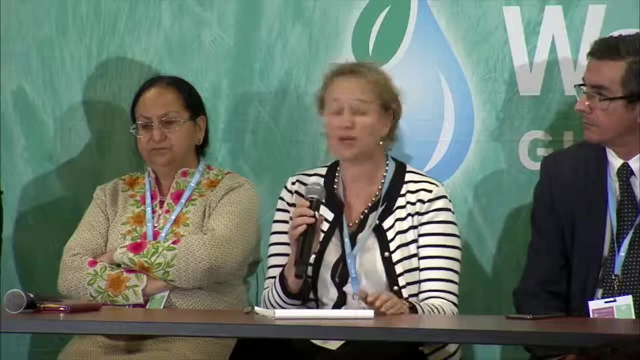 But I think that's a very good thing. We're working with a number of different organizations, farmers' unions. It's a very good conduit to get, because different sectors need different inputs, One of the things we're also working with under phase two. 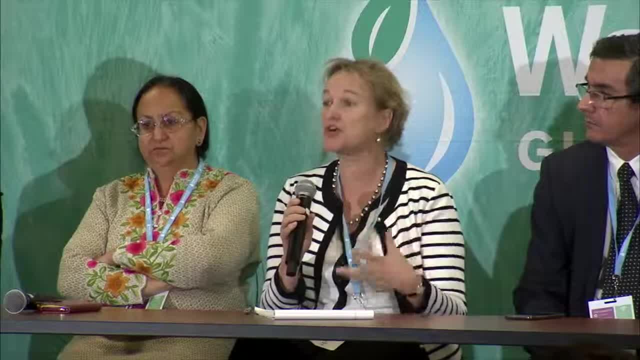 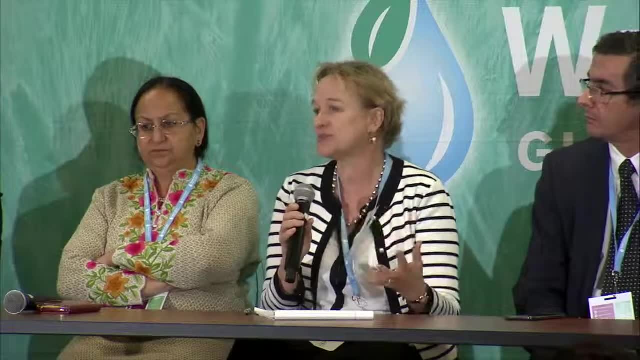 we will be doing workshops with journalists. It's very important to show what is a drought. What does it mean to be a drought? It's all very well screaming when the drought's there, when the water's turned off, But we want a much better engagement on that. 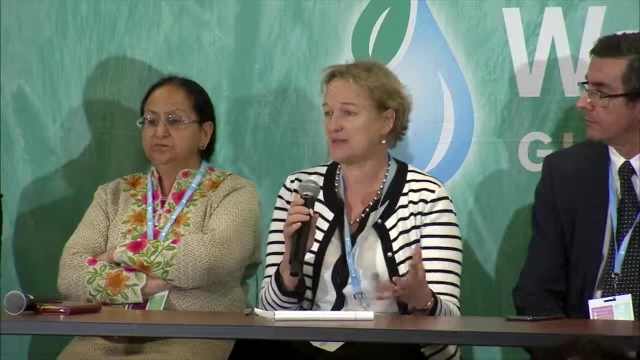 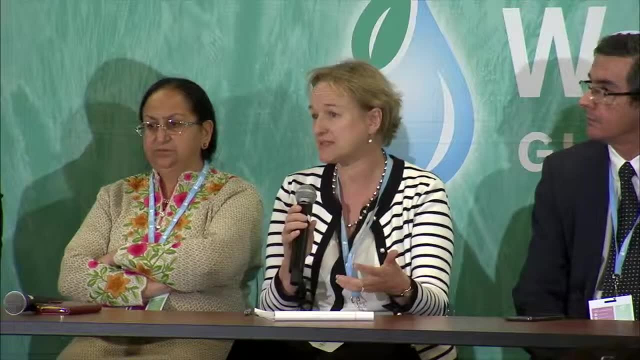 We're also talking to reinsurance companies and to banks, For example. you know people are farmers are not able to make their payments during times of drought. What can we do in understanding that? How can that be felt? So many, many different sectors- we. 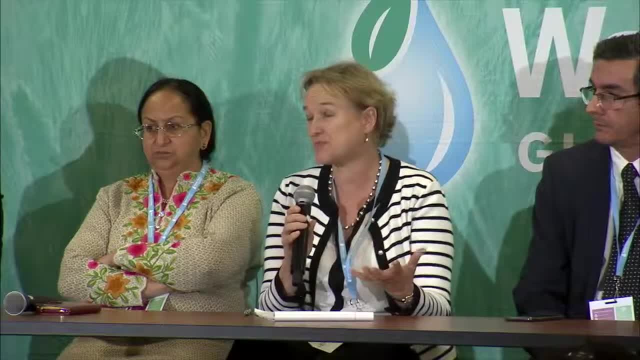 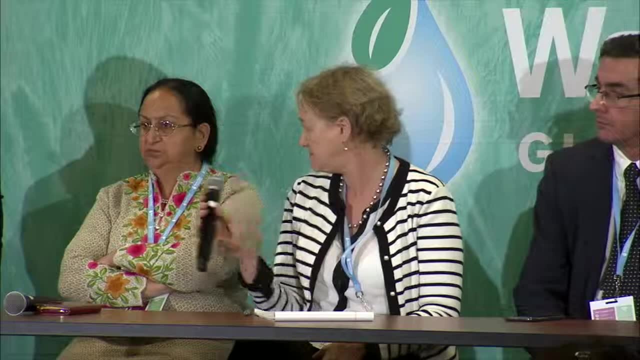 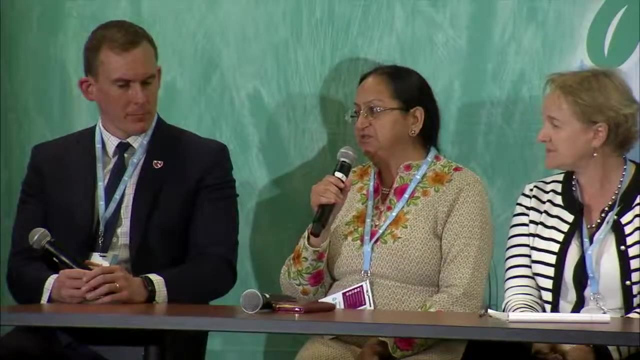 need to talk to, to help understand drought and ensure that, as we know, droughts are going to increase in extent and longevity. that communication is good. Well, as far as our side story is concerned, we have just developed the protocol, We have validated it and we have showcased it.